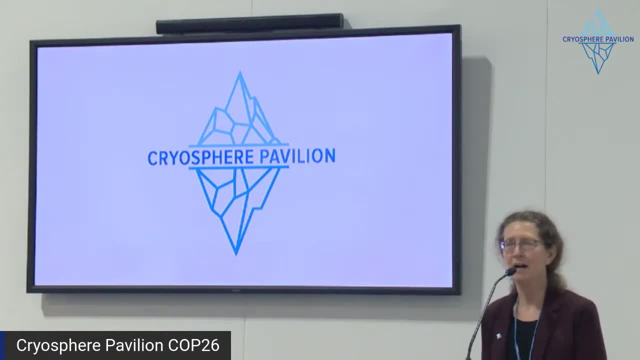 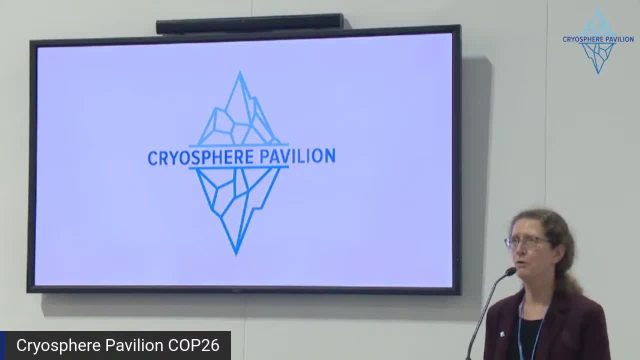 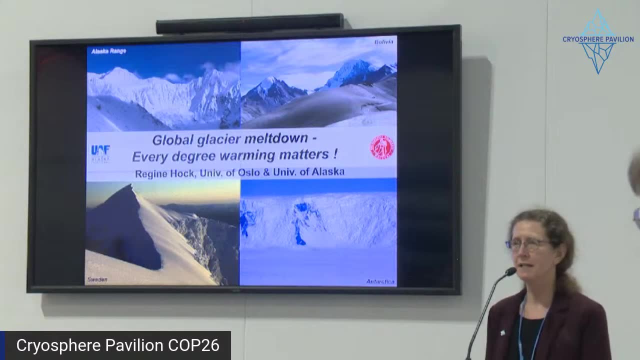 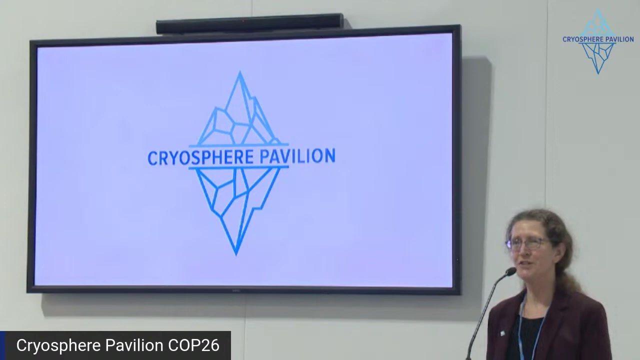 They are an incredibly important part of the global cryosphere and indeed, the global climate system. As a special treat, at the beginning of this event, we have a brief address by the co-chair of IPCC Working Group 1, Valérie Masson-Delmonte, who will say a few words at the start, Please. 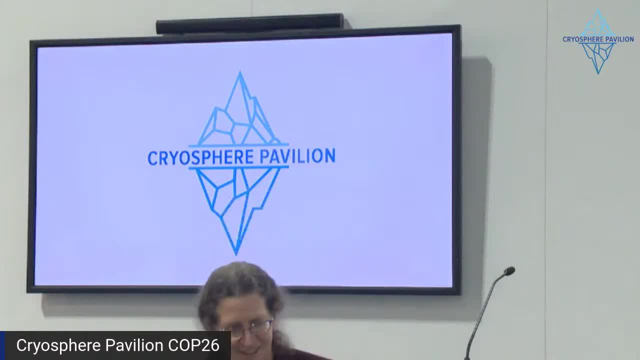 Hello everyone. It's a pleasure to be here. Thank you very much for your invitation And I would like to stress the importance of bringing scientific information within COP meetings. And it's a pleasure here to have nearby pavilions on climate, on the cross here on water. 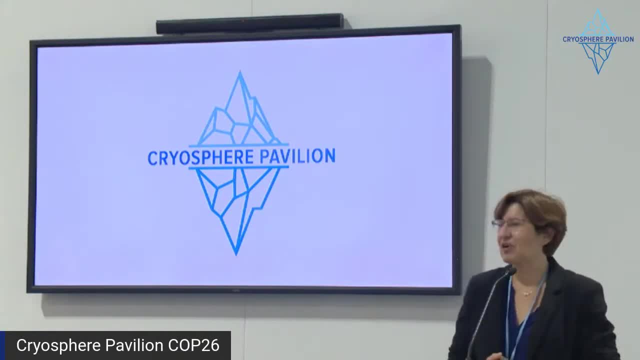 We may have an ocean one nearby in the future and they are closed. They're closely connected. So I would like to share a few things related to the last IPCC AR5 report on the physical science basis, And in that report we place an emphasis in communicating clearly the latest scientific knowledge. 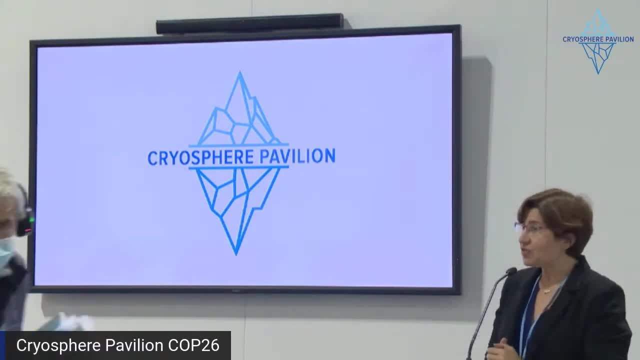 So if you are interested about mountain regions and glaciers, on the IPCC website you will find a two-page summary. This is part of our regional fact sheets And you can directly. You can directly access the summary of what has already happened. the role of human influence in what has already been observed. 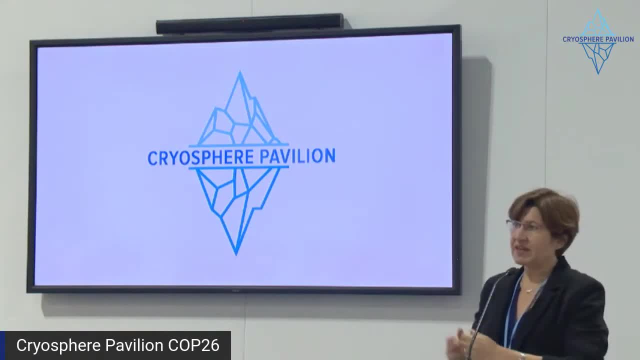 and the projections for mountain regions. So it's something novel. Previously the mountain regions were a bit hidden within the IPCC reports And this builds on the chapter on high mountains that was coordinated by Regine Hocker for the special report on the ocean and cryosphere. 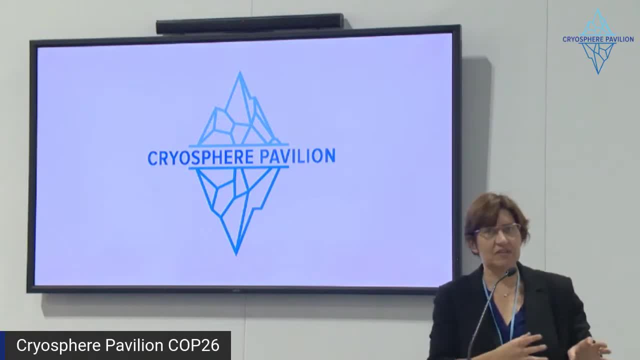 So any change that is brought up in the IPCC assessments can have a legacy And then we update the knowledge and we do all our best efforts to share that. Then a few words on the main messages from the Working Group One report, Some of the highlights: 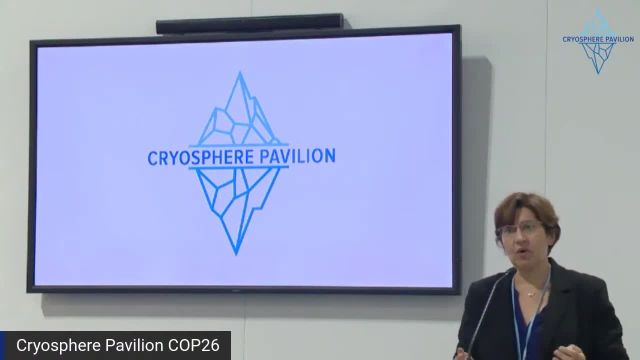 So we're now at about 1.1 degrees Celsius of global warming the last decade, compared to the late 19th century. The changes associated with that level of warming are widespread. They are rapid And bringing in information from natural archives- paleoclimatology- we saw that many are unprecedented. 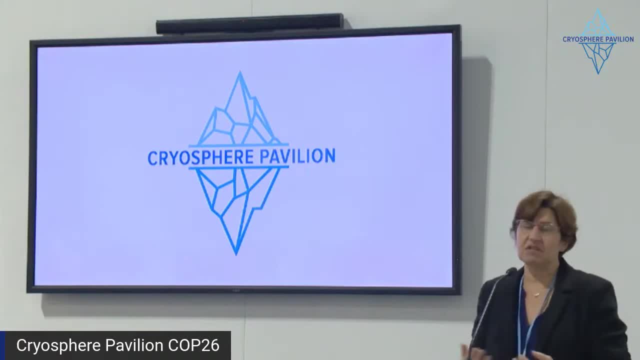 Over timescales of centuries to thousands of years, And it's the case for the global loss of glaciers. The other point is that human influence on the climate system is now unequivocal, And this results from looking at all the components of the climate system together. 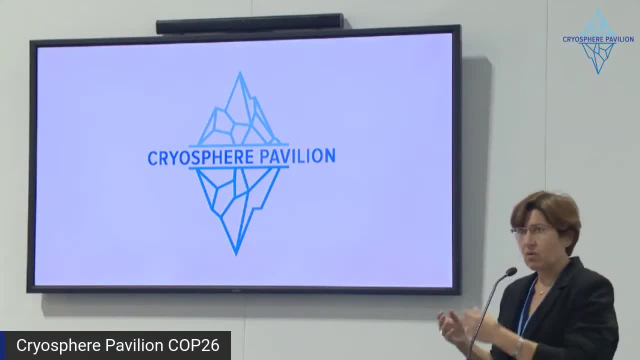 So human influence, warming the atmosphere, warming the land, warming or heating the ocean and leading to widespread loss of snow and ice, And through that whole system approach, our conclusion is that the climate system is now un-equivocal And our conclusions are very clear. 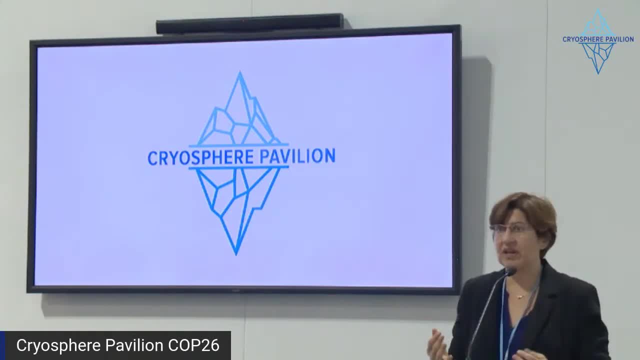 We also see a clear human influence, not just on trends but also on the frequency and intensity of extreme events- hot extremes, heavy rainfall events or droughts in some regions- And that's a novel advance from the science of attribution For future changes. of course, future warming depends on future emissions. 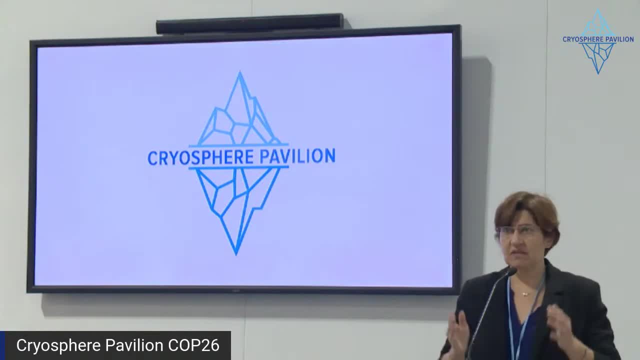 For global surface temperature. if CO2 emissions are put to zero, there's very limited. There's very limited warming averaged over 50 years. However, we have already committed the slow components to continue to change. It's the case for glaciers. 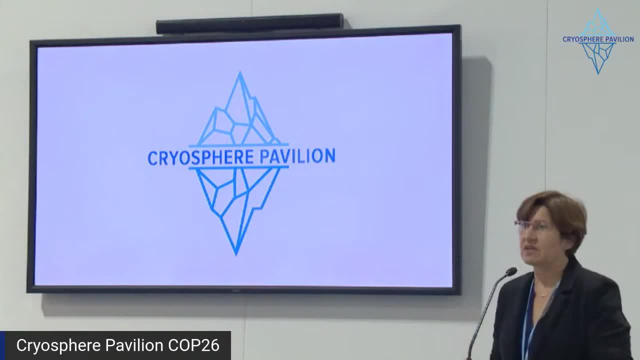 They will continue to adjust to today's warming. It's the case for the deep ocean, for the ice sheets, And our report shows that we've already committed sea level to rise on the long-time scale by something like 70 centimeters to more than one meter. 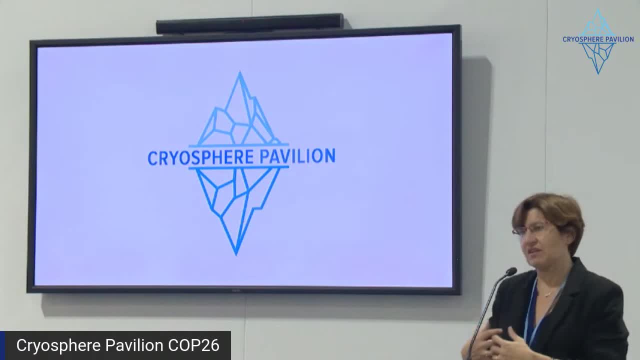 So that's also a novel advance in understanding what is committed from our past emissions. So the report shows that future warming depends on future emissions. Many regional changes are directly linked to the level of warming and therefore every single increment of warming matters and every avoided increment of warming matters. 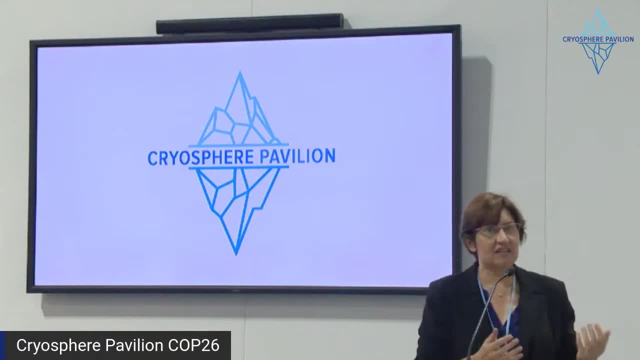 It's the case for the fast response of the snow cover or Arctic sea ice. It's also the case for the slower response of glaciers. I think these events will be the opportunity to dive deeper into how every single level of warming matters for the level of warming. 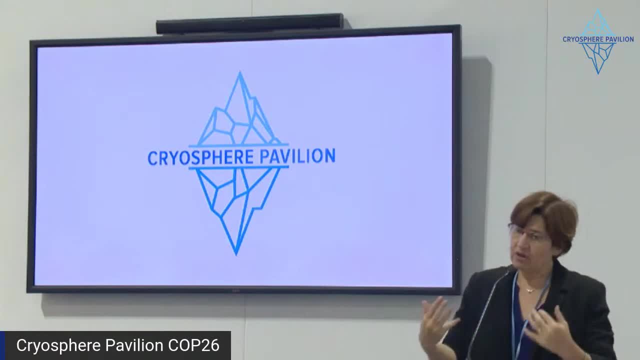 long-term fate of glaciers for the slow, committed changes associated with sea level rise. we show that how much we can slow the rate of sea level rise by limited peak warming and further declines in greenhouse gas emissions, for instance- and that's novel. in our report we show how much 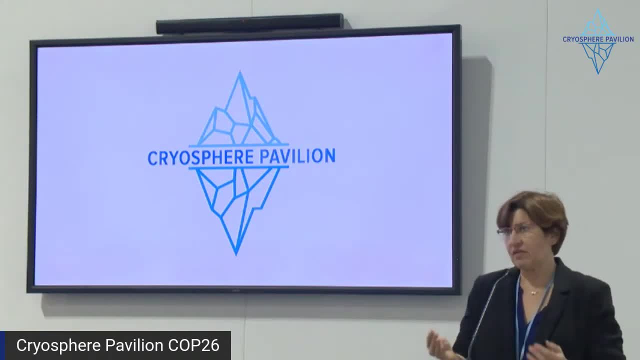 we can save time for the horizon when sea level rise would reach 50 centimeters, one meters, 1.5 or 2 meters, depending on the emissions scenarios. i was yesterday at an event with the members of parliaments from tuvalu, bangladesh or madagascar- very vulnerable areas- in a discussion on loss and 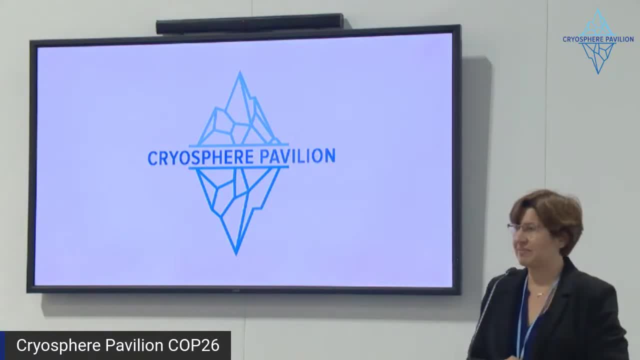 damage, and that's something that's really important for them to understand how much action now regarding greenhouse gas emissions has long-term committed consequences and any single effort to reduce emission gives them more time to adjust to invest on coastal protection or nature-based solutions that can protect coastal livelihoods. 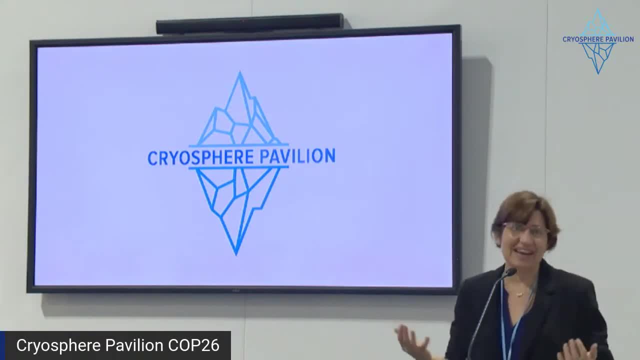 and and and people who live in in these areas, and that's also related to the fate of the glaciers, of course. so i wanted to flag a couple of these advances that are reflected in our report. if you're interested to know more on on the multiple characteristics in every region, that 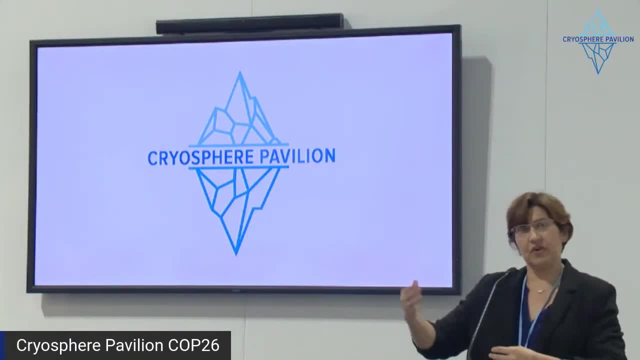 are already changing and will continue to change with further warming. we have an online interactive atlas, which is a novel tool, and you can explore yourself the data sets from the report in an open science, open data approach. make your own maps for the multiple characteristics that matter for you, where you live, and access the data sets. so this is what i wanted to stress. 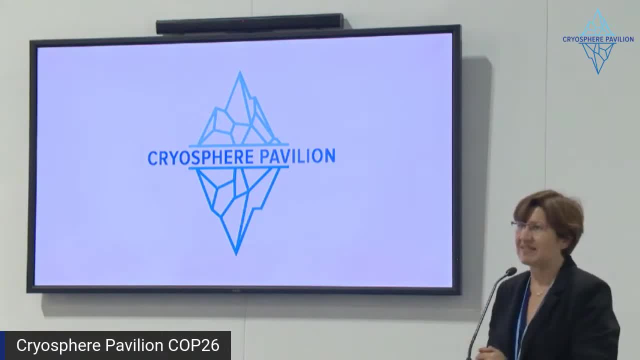 as an effort made by the scientists involved in the physical science basis to make climate information as broadly available as possible, and i've put an emphasis on the importance of of limiting warming. i would just like to flag one more point: actionable information at the regional scale that is critical to anticipate. many decisions are still made today looking backwards. 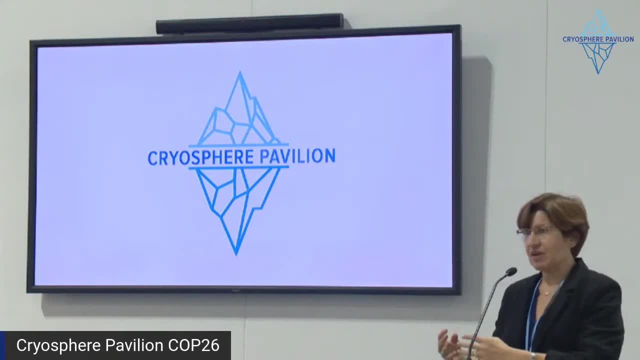 an event is happening, you react. you take action to limit the scale of the impact if the same event occurs again, but we know that trends will continue. in the next decade we expect to reach a level of warming of 1.5 degrees celsius, averaged over 20 years in the 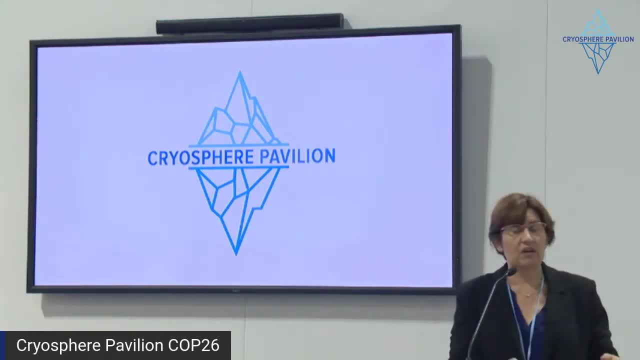 next 20 years. if emissions do not decline now in the coming years, we could still reach 2 degrees of warming by around 2050, unless there are deep reductions in emissions of methane, co2 and other greenhouse gases. so providing a clear picture of what to expect in every region associated. 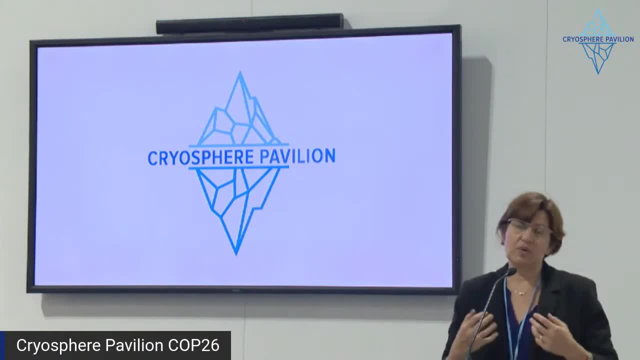 with future warming is really important to take action for resilience, for adaptation, using science, information to look forward and be prepared to what to expect, not just the changes in climate and climate change looking backwards. with that, i would like to thank you for this opportunity to to share these. 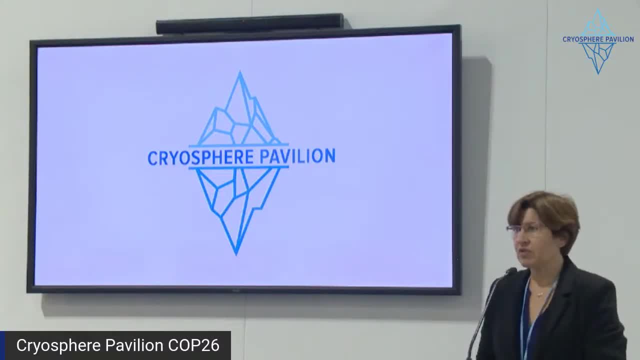 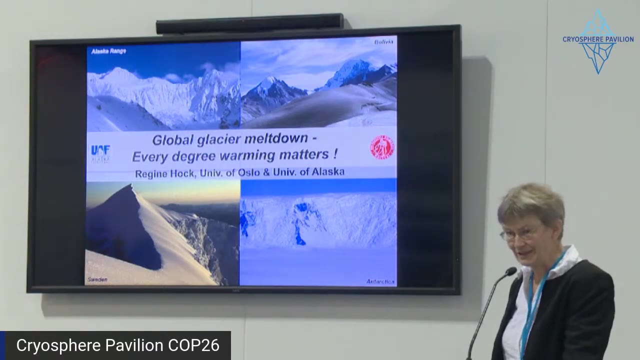 elements, and i hope you will. you will use this report to inform your decisions, thank you. okay, thank you, and thank you for having the opportunity to speak here. so i will take you to the world of glaziers and try to convince you that every degree warming 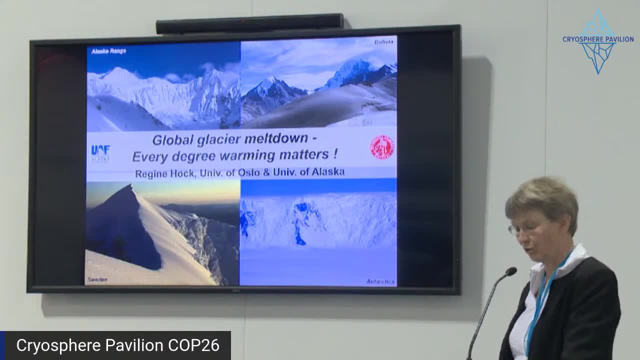 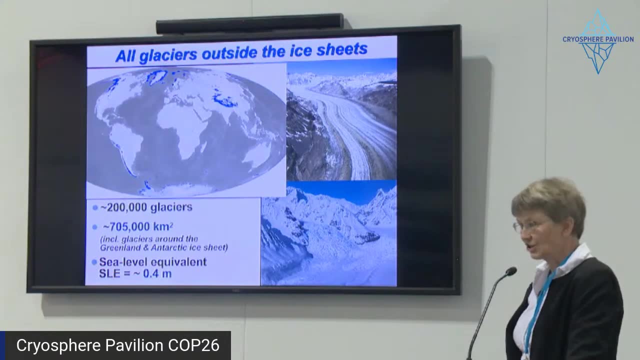 matters, or especially avoiding every increment of warming for the survival of the glaziers. i will talk about all glaziers outside the ice sheet, so not the ice sheet in greenland antarctica, but all the glaziers outside the ice sheet. that is about 200 000 glaziers covering an area of 700 000. 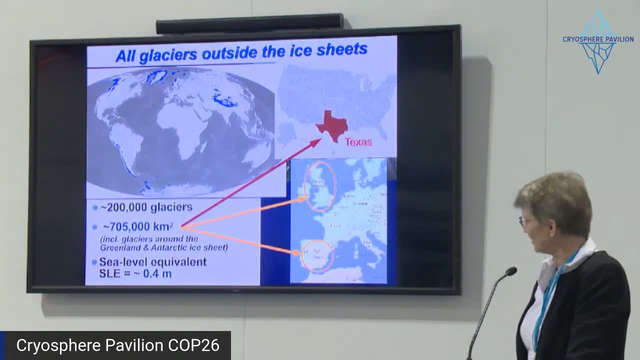 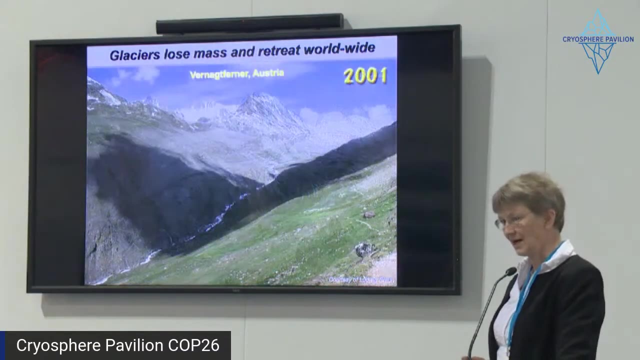 square kilometers, which is the area of texas or the area of the uk and spain together, and the sea level equivalent. if you melted all glaziers, sea level would rise about 40 centimeters. globally, these glaziers have dramatically retreated, thinned and lost. 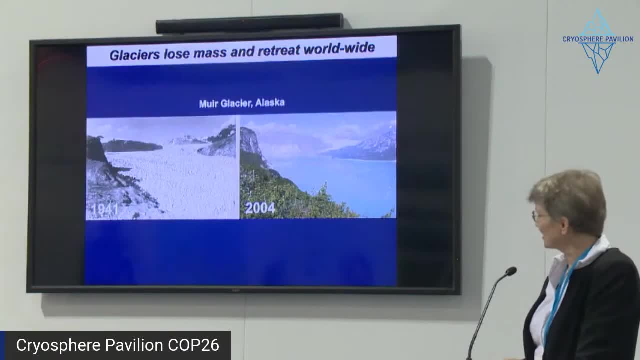 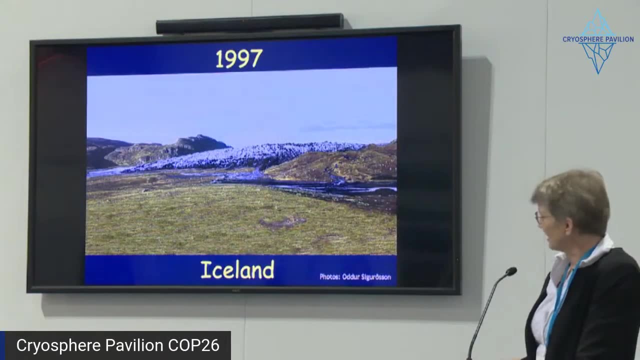 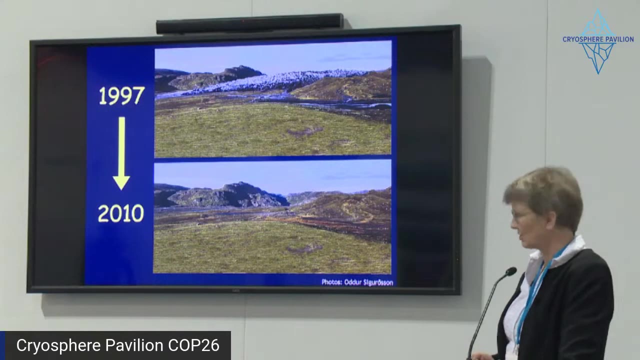 mass in the last century and decades here. just a few examples here from alaska: a dramatic change, pedagonia, and here in iceland and just a few years, as you can see here. so within 13 years, a dramatic change. the laser is not visible anymore from this location. 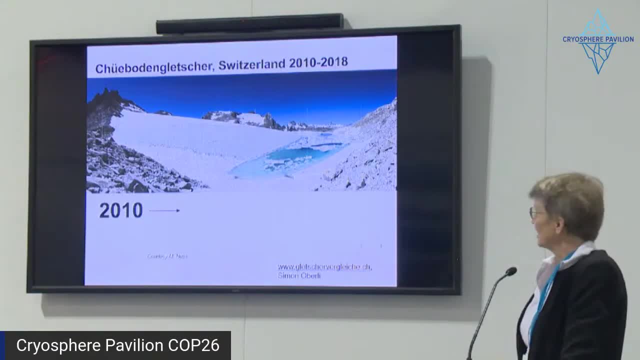 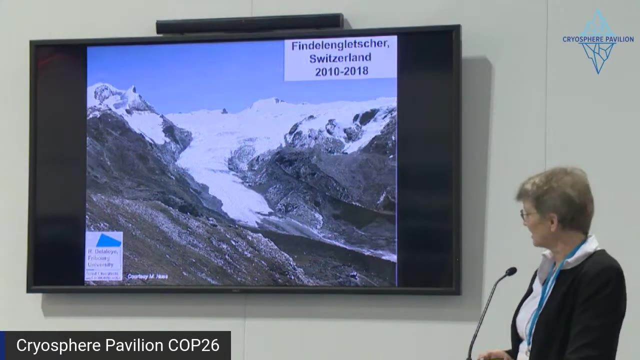 or what is really new is, in the very recent years there's dramatic changes just within a couple, within a few years, like here in switzerland, just in, in, uh, within eight years i mean a massive change of this little glacier here and the same here findling glacier in switzerland. massive changes just in. 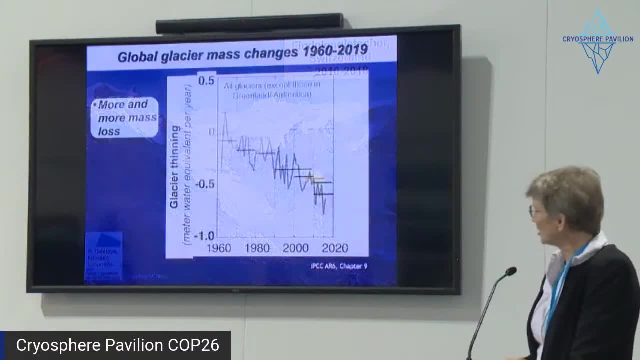 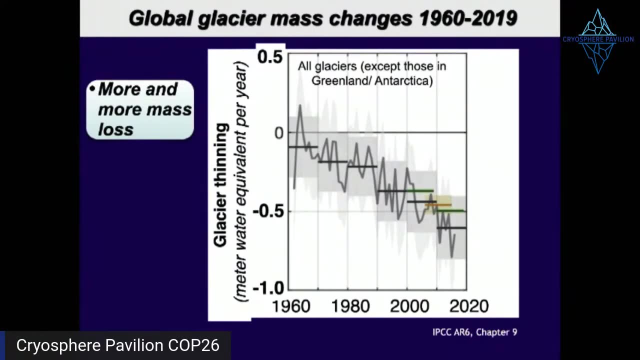 a few years. on a global scale, this is now all glaciers in the world, the thinning rate per year, the annual variations here and also, like um, for every decade, the mean. so minus one, 0.5, means an average thinning over all glaciers in the world of a half a meter per year. 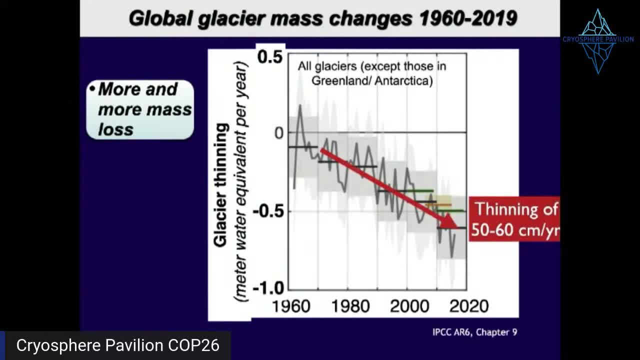 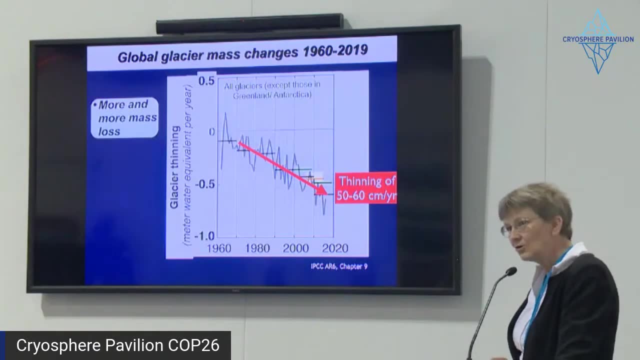 and what you can see is that the thinning is increasing, so the mass. there's more and more mass loss from these glaciers. so now the average thinning rate is about 50 to 60 centimeters per year, average over all layers in the world. but locally there's differences, like regions, like the. 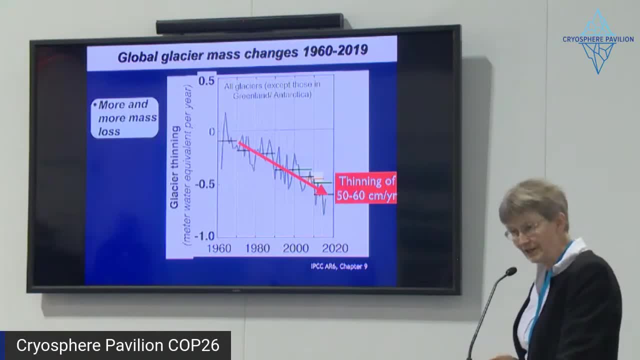 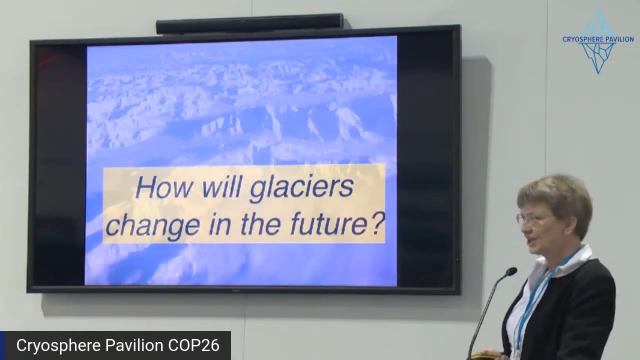 european alps, they are thinning at a rate of a meter per year, whereas whereas other regions, like in the high polar regions, like northern uh, like uh canadian arctic, are thinning maybe at a rate of 10 or 20 centimeters per year. so how will glaciers change in the future? here a simulation of 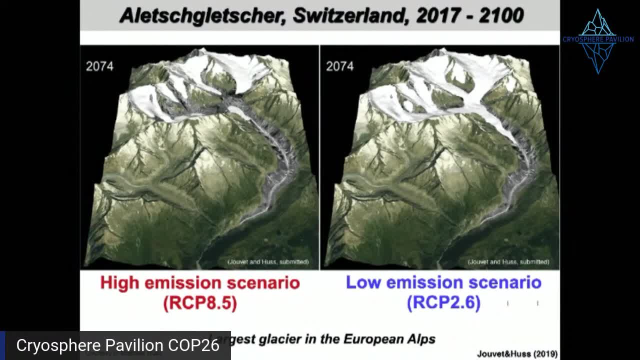 the average thinning rate in switzerland, the largest glacier on the european alps and what you can see. with a high emission scenario it's almost going to disappear. but also what is encouraging here is to see that the emission scenario matters. so with a low emission scenario, um, at least sort of half of the glacier is still left. 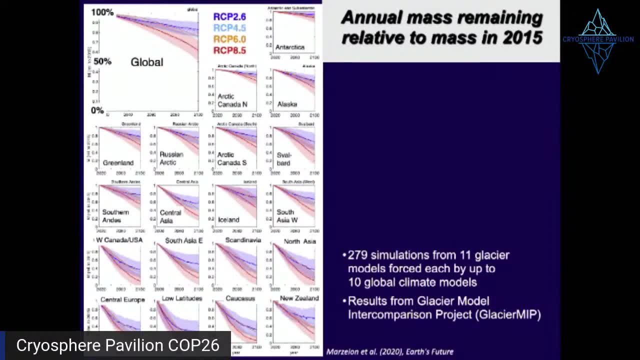 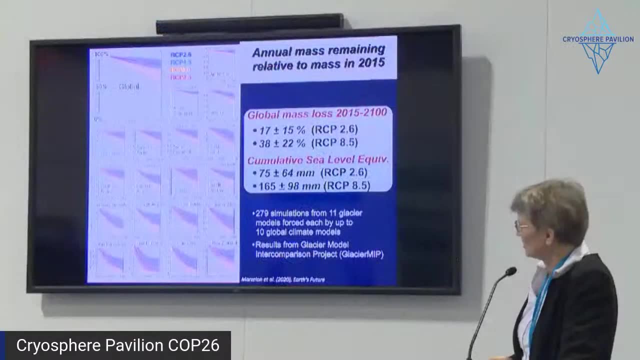 what you see here is the annual mass that is remaining relative to now. now we have a hundred percent and um globally and for every single region that has glaciers in the world, globally we see a mass reduction of about almost 20 to 40 percent by the end of the century, depending on the emission. 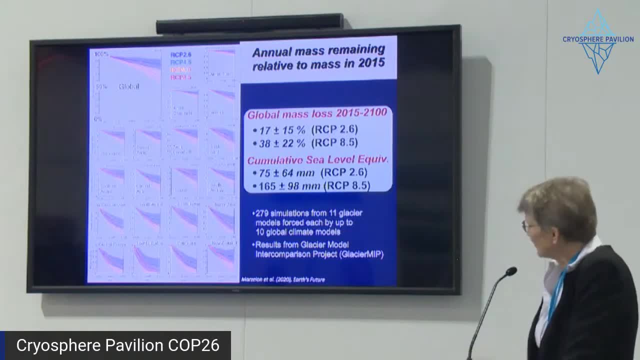 scenario and that corresponds to a sea level equivalent of about 8 to 17 centimeters. but when you look locally, there's huge differences here. the canadian arctic, alaska, the glaciers around greenland, russian arctic, uh, the. the mass losses are maybe 10, 20, 30. 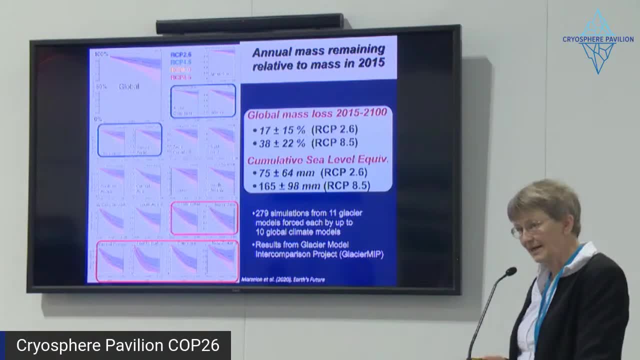 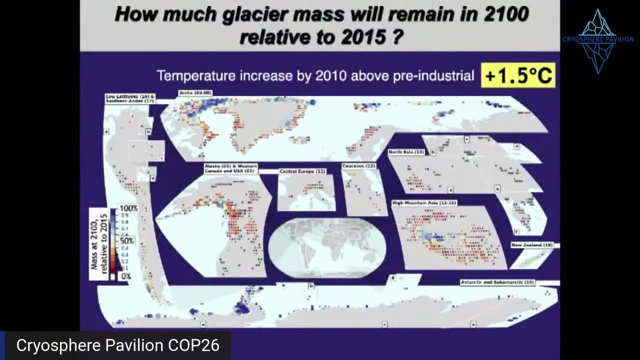 percent. but the regions that have very little ice right now, like scandinavia, central europe, under the high emission scenario, their projections are almost complete deglazation, so dramatic changes. so here we translated these emission scenarios from the global climate models into degrees warming above pre-industrial, and what you see here is now. 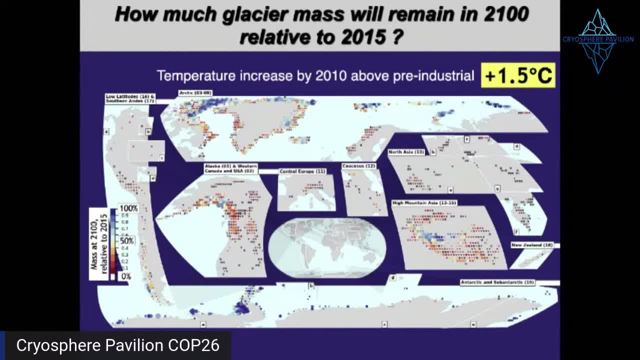 for every grid cell that has a glacier there's a dot for how much um? how much ice mass is remaining by the end of the century for a plus 1.5 degree scenario. so the more blue you see, the better it looks, and mass is remaining. so dark blue is essentially 90 to almost 100 percent of the 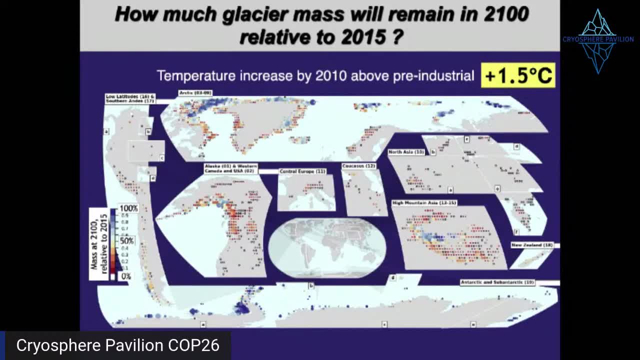 ice mass is still remaining by the end of the century. for the plus 1.5 degrees, the redder it is, the less mass is remaining. the dark red means only 5, 10 or 15 or nothing is remaining, and every black dot means the glaciers are gone. and this is here for two plus two degrees plus three degrees plus. 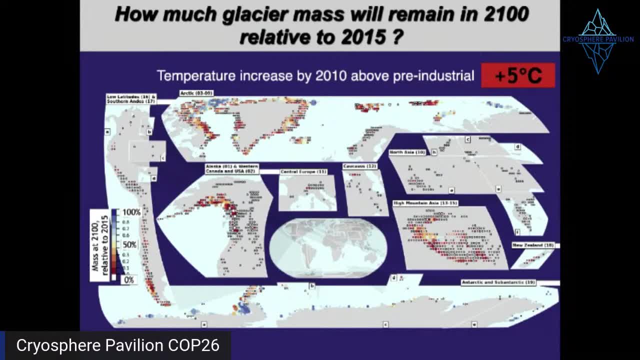 four degrees plus five degrees, so by emission scenarios here plus five degree degrees. there's still a lot of mass remaining in the very high polar regions. but the rest of the world is especially these regions here in scandinavia, european alps, kakas and caucasus and so on. the glaciers are essentially gone. 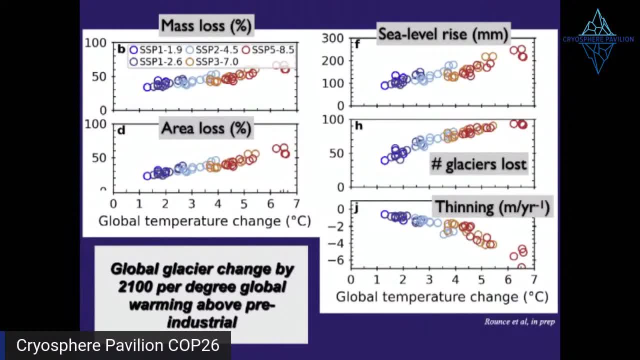 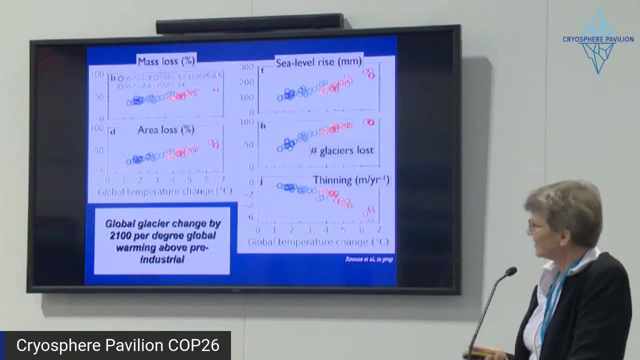 here you see on a global scale, the global glacier change projected by the end of the century. for every degree global warming, above in above, industrial, pre-industrial, You see the mass loss for every degree in percent. the sea level rise, the area loss, the number of glaciers lost almost 100% by the end of the century. for the: 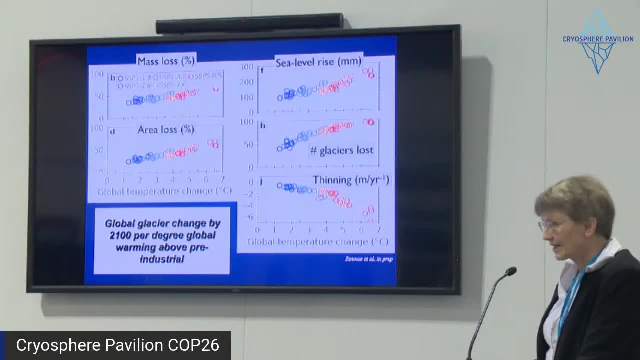 high temperature scenario And you see the thinning rate, like the thinning rate for the high temperature, plus six degrees, is almost a six meter per year thinning over all the glaciers in the world, And what you see here. so the key message is here temperature matters, Every degree. 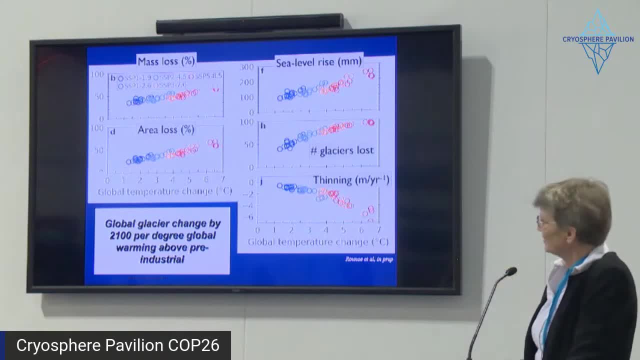 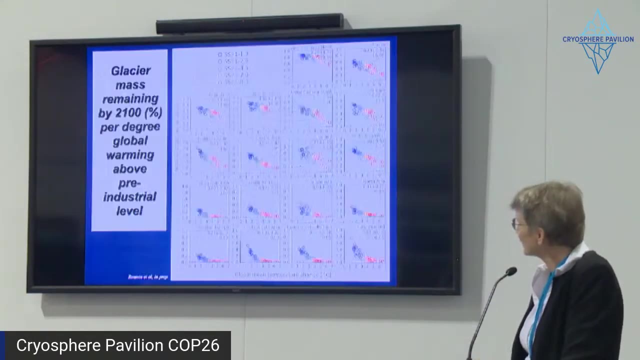 matters. So it's just a linear increase: more mass loss, more area loss, more sea level rise with every increment of more global warming And the positive message with this is limiting the warming you can, limiting the mass loss. This is the same figure here for every region now in the world. 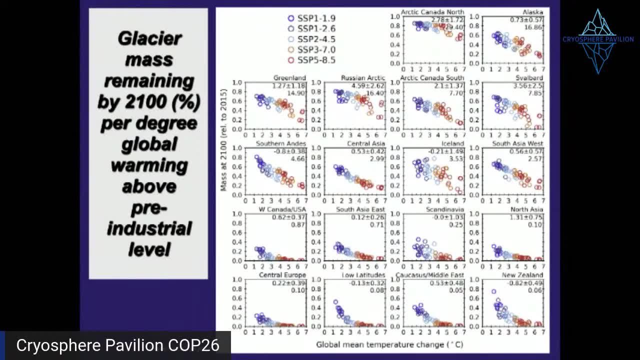 And again now it is shown the mass, the initial mass, and how much is remaining, And for all regions. yeah, here this goes almost linearly down. for some regions- Central Europe and low latitudes- they're very sensitive if it's one degree warming or two degree warming. 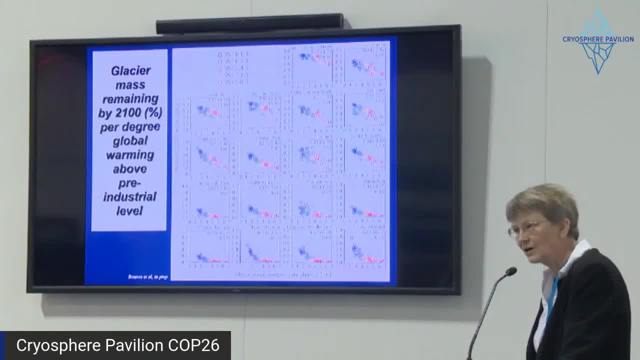 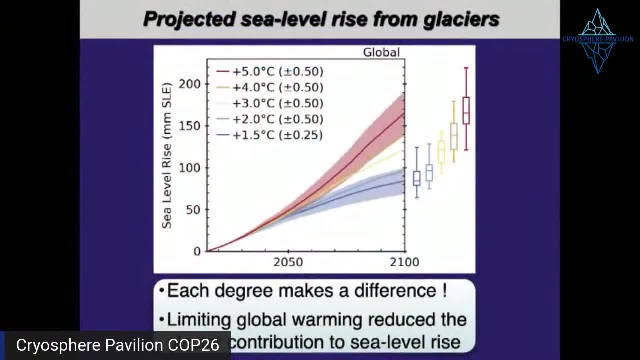 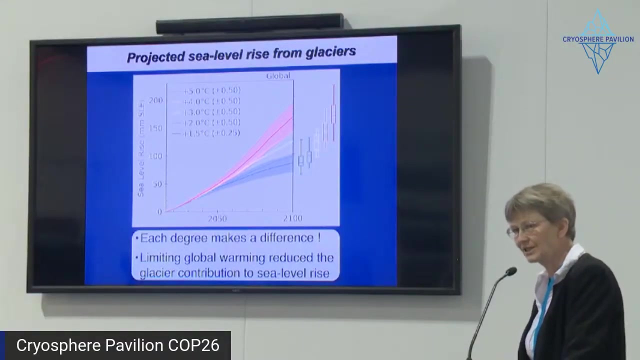 Here you see the projected sea level rise from these glaciers And also here you see clearly, by the end of the century every degree more warming matters. The contribution by the end of the century is higher with every single degree warming. So each degree makes a difference And that also means limiting global warming. reduces the glacier contribution to sea level rise. 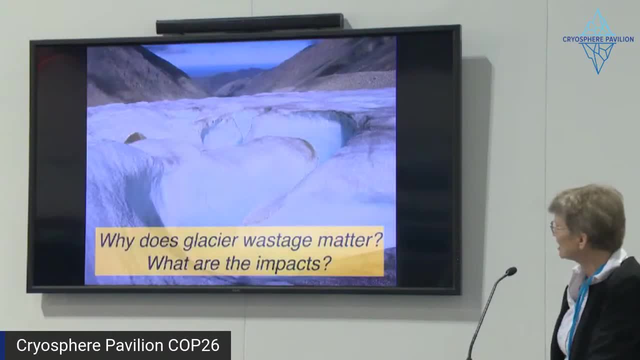 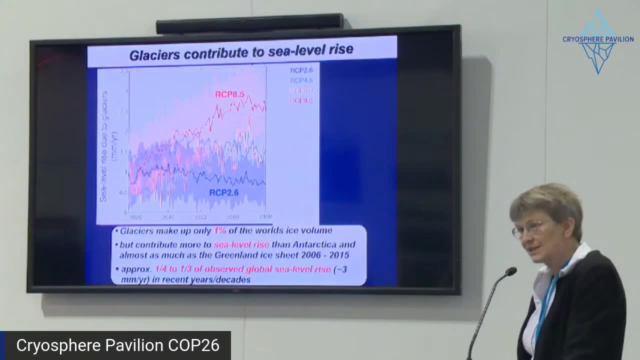 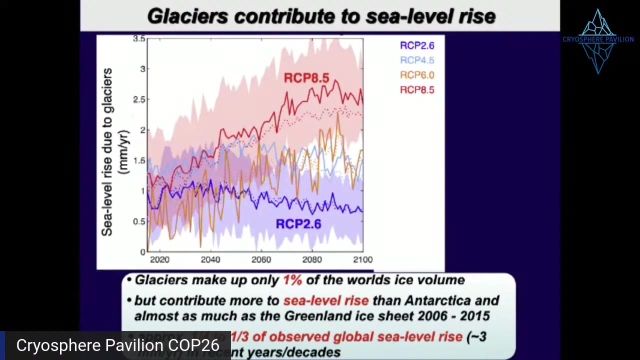 Almost here in a linear way. What are the impacts? I mentioned already here sea level rise, These glaciers outside the ice sheets. they make only up one percent of the world's ice volume, But they contribute to sea level rise in the past, in the recent decades, more than Antarctica and more. 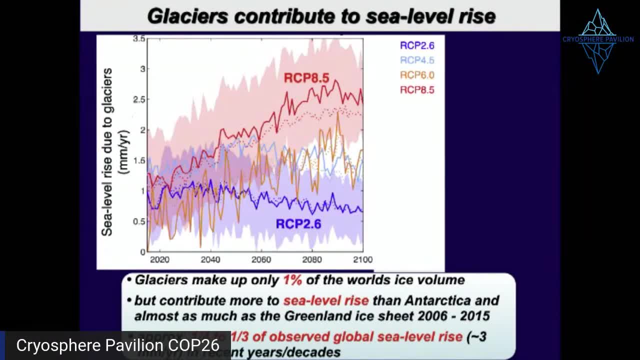 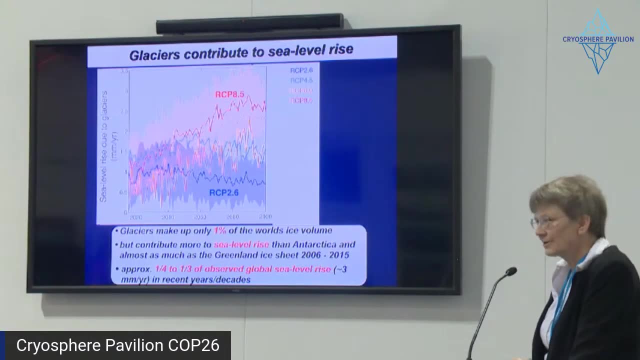 almost just as much as the Greenland ice sheet here during this recent period And overall these glaciers outside the ice sheets have contributed about. they make a fourth to a third of observed sea level rise in the recent decades. And what is really? when you look at the projections you see for the higher emission scenario, the RCP 8.5,. 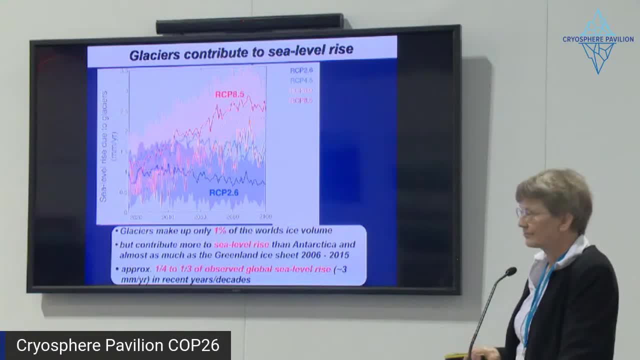 it goes linearly up. the rate of sea level rise every year And for the RCP 2.6, you see, it goes down again And that's because some glaciers, they, they retreat to higher elevations and they can then survive at higher elevations. 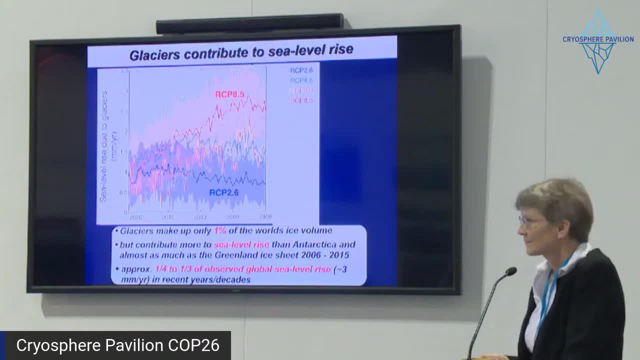 And don't contribute any more to the environment, contribute anymore to sea level rise. But what is really interesting is we have right now a sea level contribution every year of about 3, 3.3 millimeters By the end of the century. what we 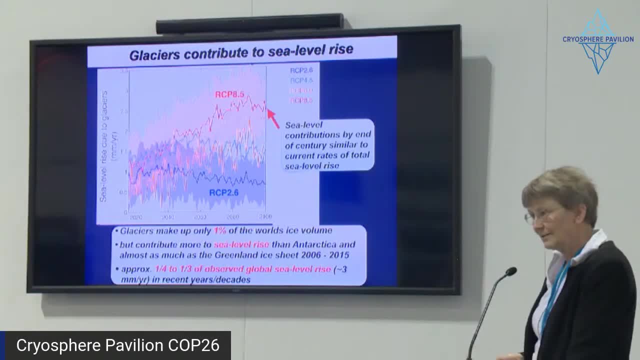 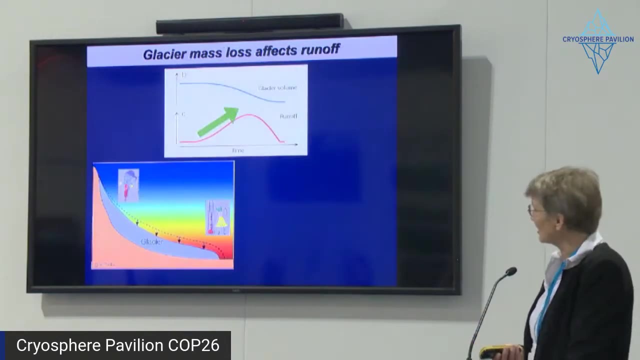 project here is sea level contributions for the high emission scenario that are just as high as the entire sea level rise right now from the ice sheets and thermal expansion and other sources, So it's really a major contributor here. Another important point is that glacier mass loss affects 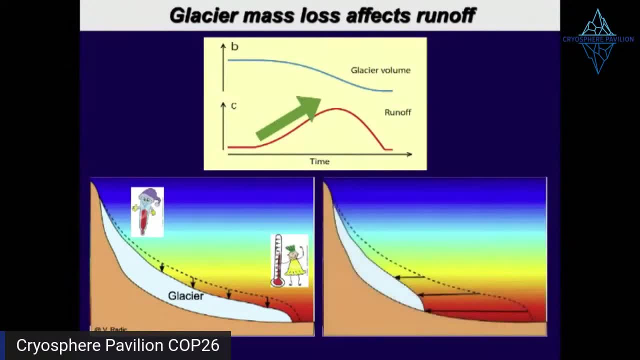 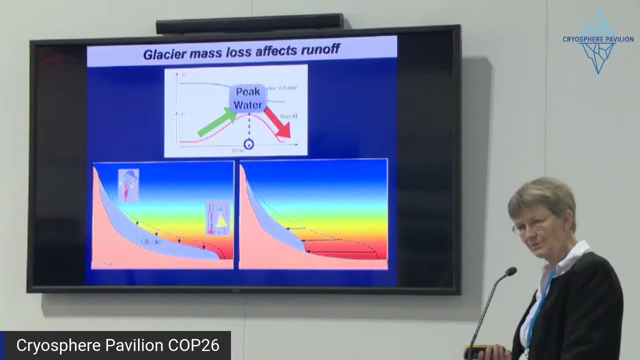 runoff. When glaciers retreat, runoff typically goes up, first because there's more melt, and then the runoff will go down. And this point, this turning point, we call peak water, and that is, of course, very important for water resources management. We need to know: is there more water? 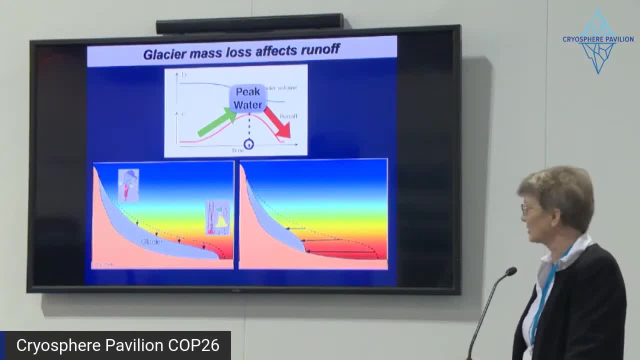 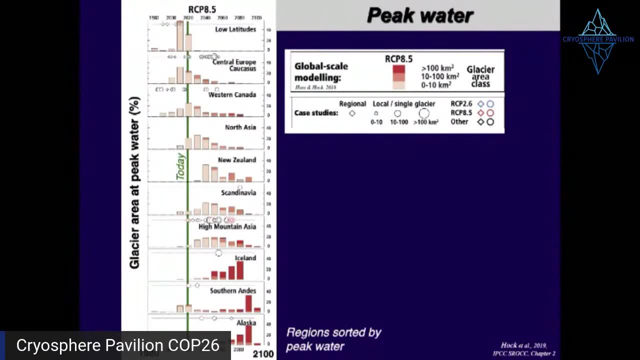 coming from the glaciers or is there less? There's less water coming from the glaciers with time. This is your compilation here from the IPCC SROC report of all studies about peak water. The bars are a modeling study. modeling when does peak water happen with every single glacier in. 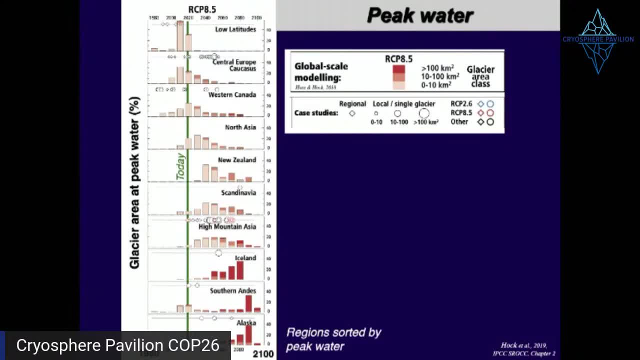 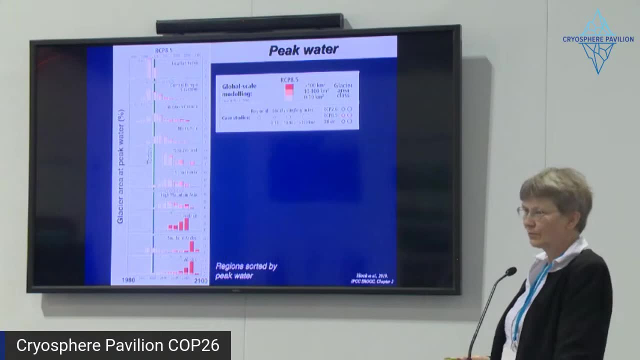 these regions And the sum of all the area of the bars is 100% for an area And obviously within an area there are spatial variations, So this is why these bars are spread out. But you see, the line here for today is the green line And the more of the bars are to the left. 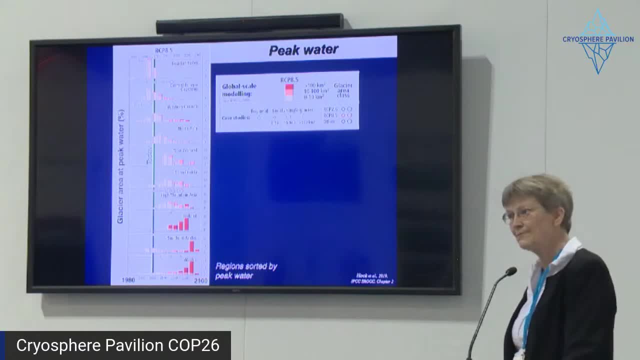 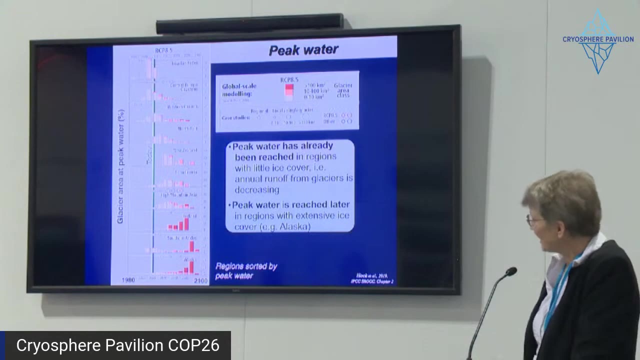 the more of the area in that region has already passed peak water. That means there's less water coming from this net glacier storage, contributing to rivers And in regions. so peak water has already been reached, especially in regions with little ice cover, like the low latitudes, Central Europe. 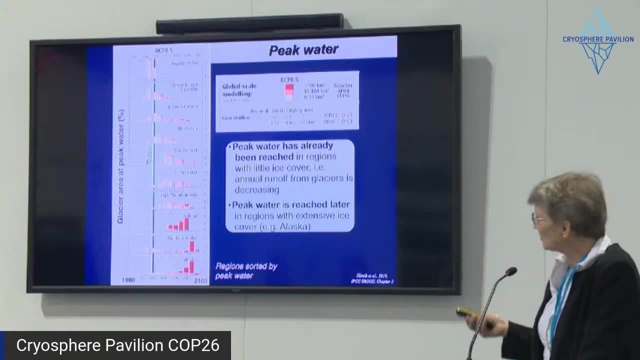 or Western Canada. But peak water is reached much later in regions with extensive ice cover, So like Alaska or the southern Andes or Iceland. That means in these regions runoff water from the glacier is actually increasing and contributing to streamflow. And, of course, then can be used for agriculture and hydropower and so on. So it also depends where you are, if runoff is increasing or if runoff is decreasing due to the melt of glaciers. Within the region there's huge spatial variations. This is here: peak water, the colors of the years. 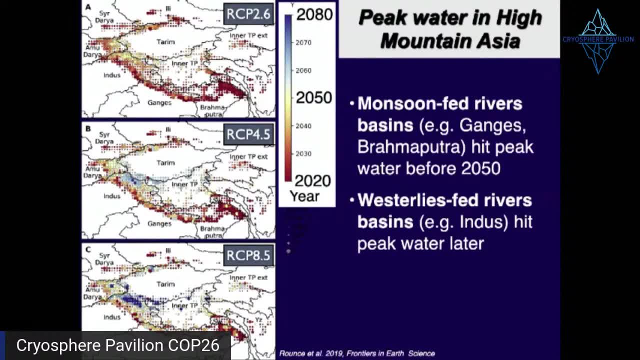 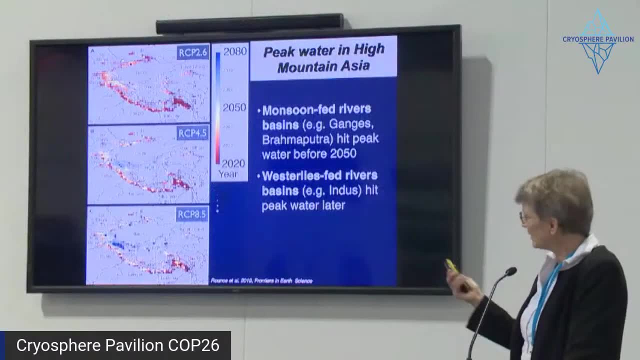 when peak water is reached here in high mountain Asia. So each dot is when the peak water has reached A lot. of red means it's reached already, while runoff is decreasing. Blue is it will be reached much, much later. And the key message here is that there's huge spatial variations. 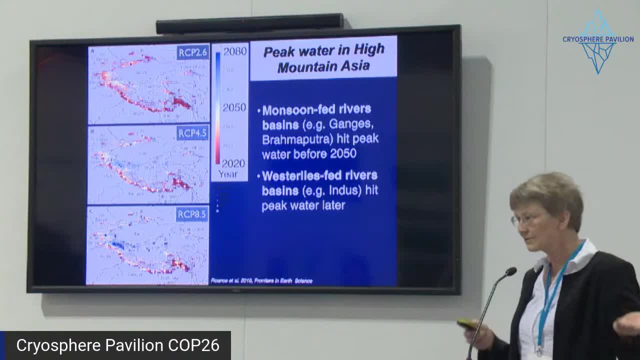 It really depends where you are. In one catch point the runoff can be increasing, whereas in other it is decreasing due to glacier melt, And here the differences are climate related, depending. if you're in a monsoon-fed river like the Ganges and Brahmaputra, peak water will be hit. 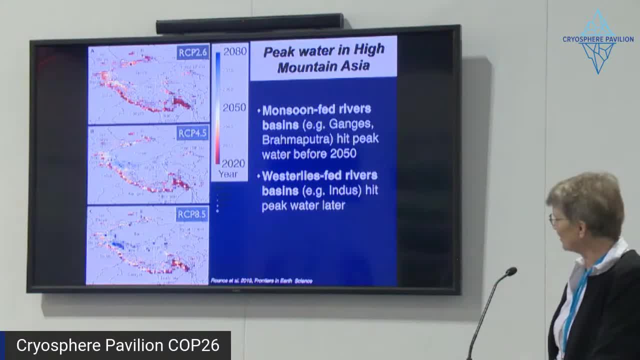 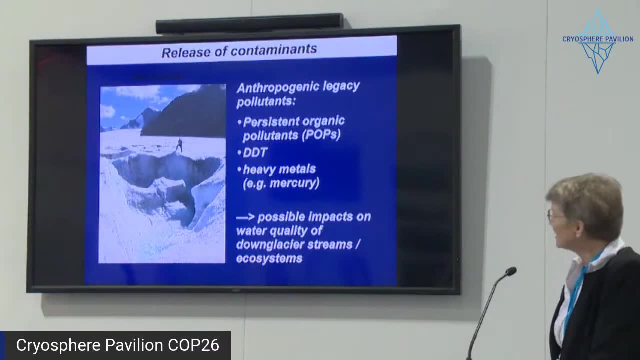 before the middle of the century. Whereas here in westerly-fed rivers like the Indus, peak water is hit later, So the runoff can be increasing, whereas here in the Indus peak water is hit later, But large spatial variations, The melt water from the glacier- there's another impact here. 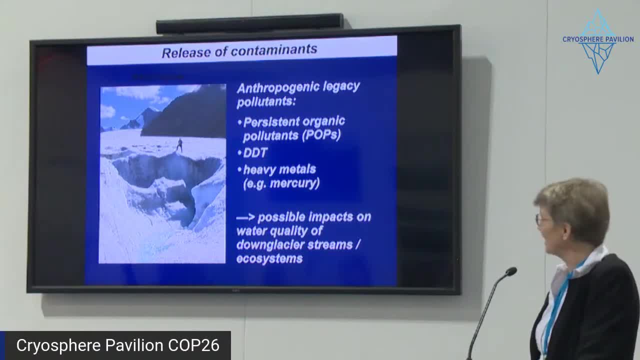 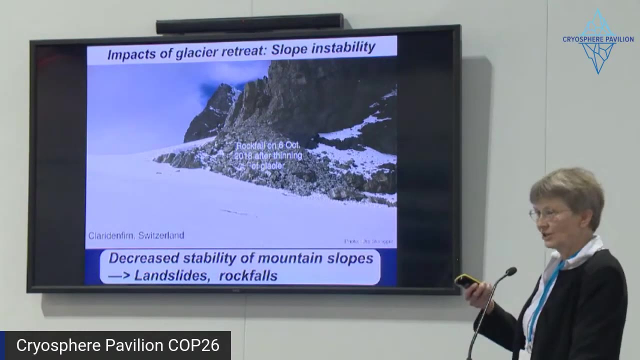 can release contaminants. There's anthropogenic legacy pollutants in the glaciers And there's possible impact here on water quality of downed glacier streams and ecosystems when the glaciers melt. Another impact is when the glacier is thin. they expose the rock and it can 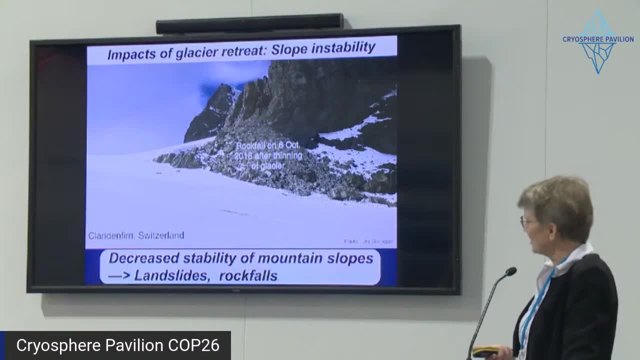 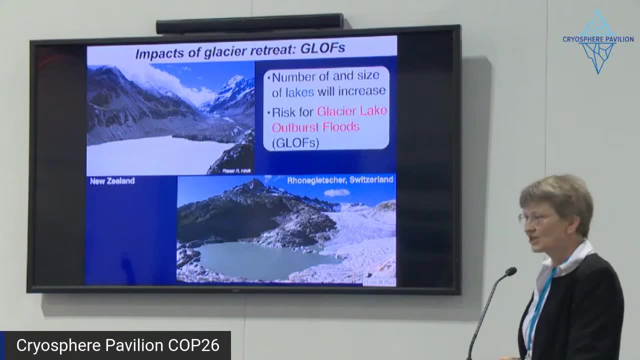 lead here to rock instabilities. Here an example here from Switzerland after a rock fall after a massive thinning. Another impact is the potential for glacier outburst floods. The number and size of lakes is projected to increase as the glaciers retreat and water is filling over deepenings, And that implies a risk for glacier outburst floods. 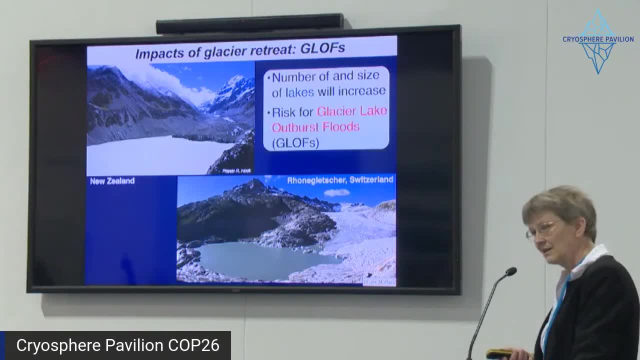 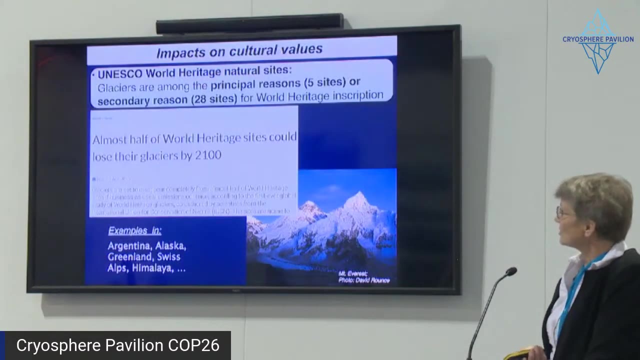 And those are really the most deadly hazards from glaciers. So the most deadly event here was in India in 2013, with more than 4,000 fatalities because one of the glaciers catastrophically drained. It also impacts cultural values here. In a number of cases, glaciers were the principal. 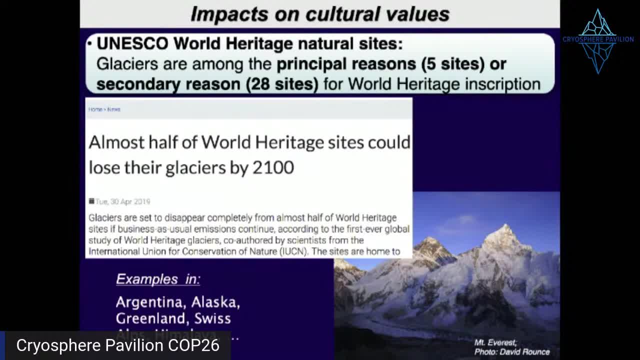 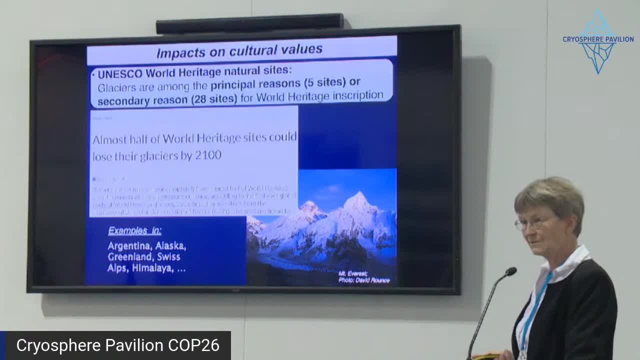 reason or the secondary reason for world heritage inscription. But the projection show that in half of these world heritage sites could lose their glaciers completely. So the reason why they became world heritage sites disappears. Another impact is here on cultural values In many communities around the world. 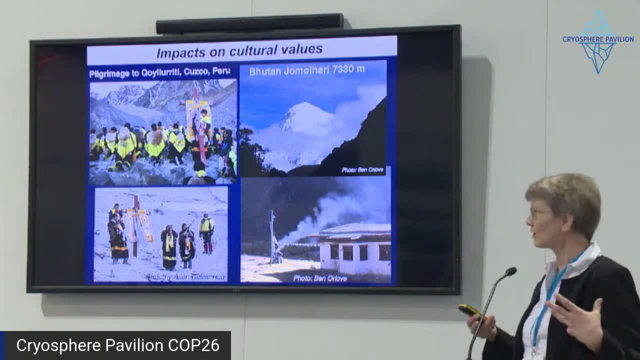 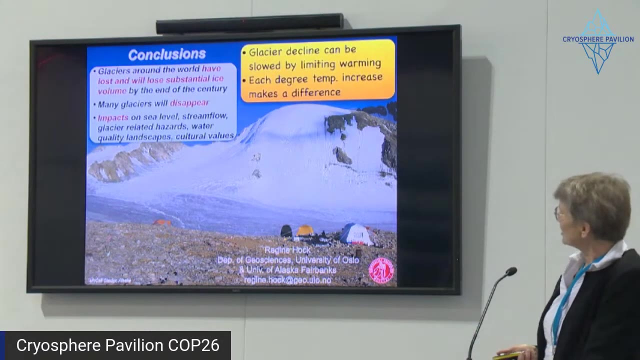 the glaciers are part of their spiritual belief system, a part of their culture, And it has been shown that it has negative impact on their well-being if these glaciers suddenly disappear. So I just want to conclude here. My main conclusion is this here, Glacier decline can. 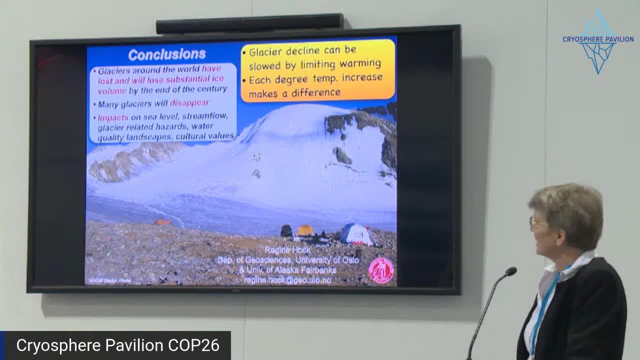 be slowed by limiting warming, And each degree, really each increment, avoiding each increment of temperature increase makes a difference for the meltdown of the glaciers that we observe right now. Thank you very much. I think yes, yes, Any. anybody has any questions Happy to answer. 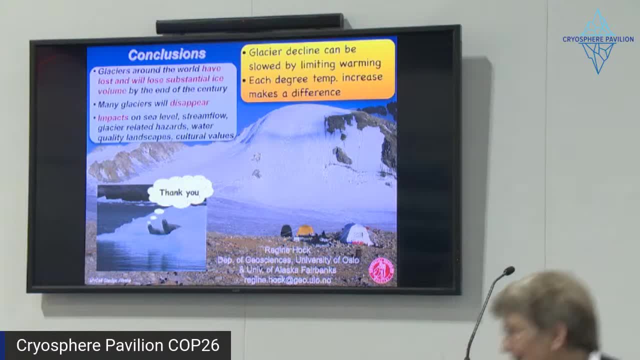 I think you need to go to Hi. Did you look at the impact on the changes of occurrence with the cold water coming down or the determination of the glaciers, and how it captivates the current in the water TICO current system in the world because of 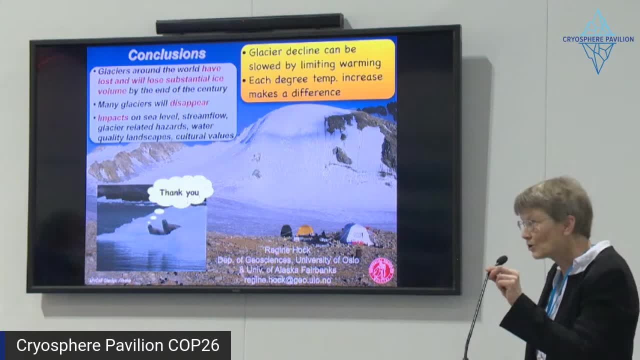 glass melting. I didn't talk about it. This is mostly research associated to the freshwater influx, from the green and ice sheet, for instance, but also in the Gulf of Alaska it has been shown that it impacts ocean currents and it impacts actually the ecosystem, the. 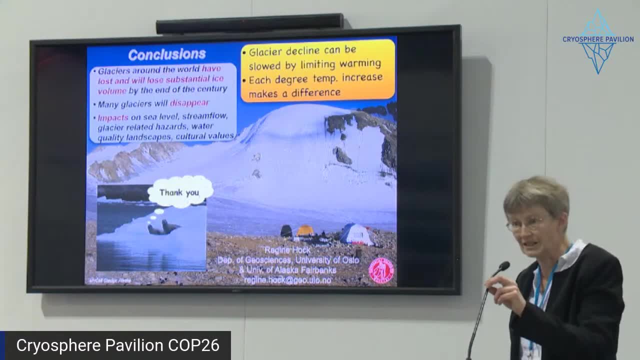 nutrient intake into the ocean. There's research about that and there's definitely impacts. I think the talk is on YouTube and I'm also happy to share any slides and information. You can just contact me and I can send you stuff. Do we have? 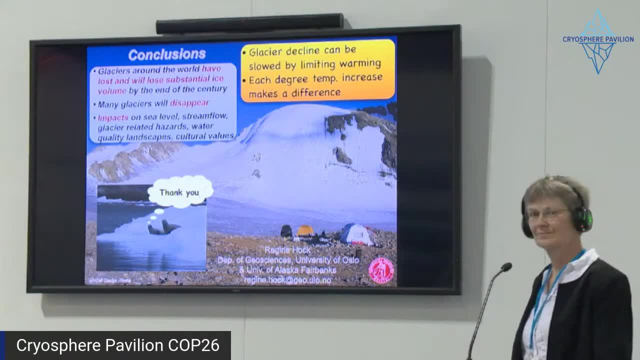 any more questions. I realize it's always dangerous to ask a scientist to speculate, but can you discuss? let's say, we exceed two degrees or even three degrees? What is the time frame to restore glaciers if they, let's say, they're totally lost? 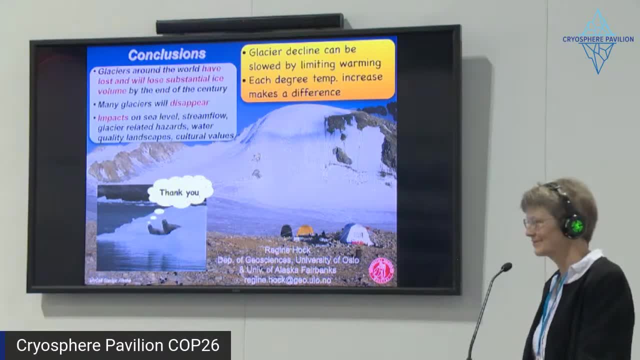 so there's no more ice. How long would it take to restore a glacier, to say its 1950 extent, do you think? Well, that's a difficult question. There's not many projections doing that, but there is in some regions. 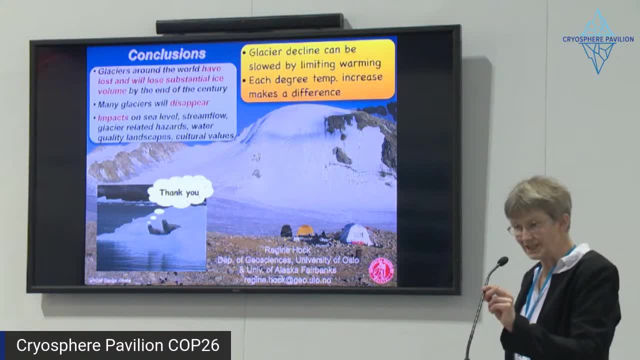 I didn't show it, but if warming is limited to 1.2 or 2 degrees, it has been shown that the mass is, there's a mass loss. but then it sort of reaches a turning point once the glaciers retreat sufficiently high, up to colder regions that the glaciers actually start growing again, And that has been shown to happen in the European Alps for instance, And the time scale it will very much depend on where you are, But it has been shown that the glaciers can grow again. 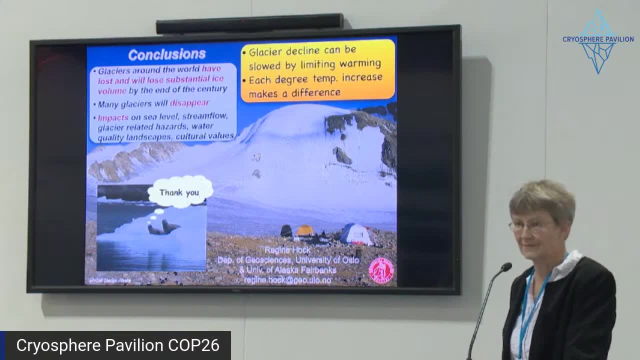 if the warming is limited to 1.5 or 2 degrees. Any more questions from the audience? Yes, There seem to be some regions in the world, like Karakoram in Pakistan, with the Karakoram anomaly, where glaciers would be moving either stable or 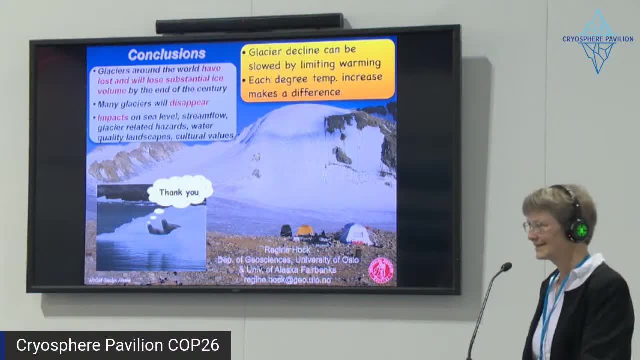 even advancing. Can you elaborate on that if you have any facts or opinion? Yes, In the high mountain ages overall the average of the glacier thinning is actually quite little. It's much less than in the rest of the world, And that has. 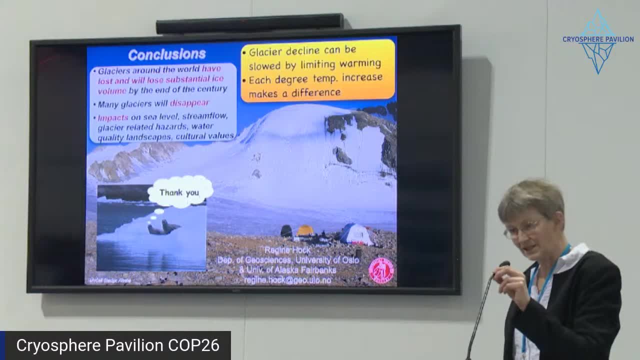 to do with. there are some regions, though, that have, at least until recently, been either stable or even gaining mass, And that is still a little bit of a mystery, but there's a lot of research going on on that topic and related with local 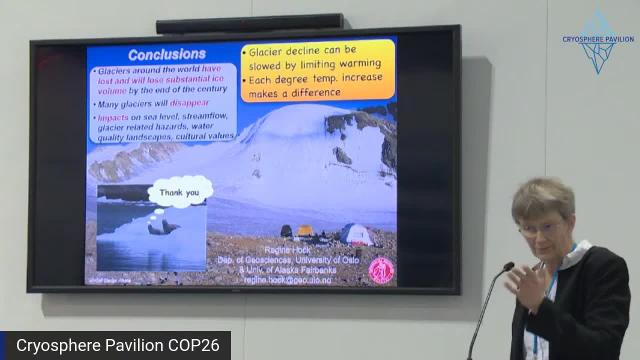 meteorological conditions That in some regions the glaciers were stable or even advancing and gaining mass. But in the long run, the projections show that this — with every degree warming — they're losing there will lose mass as well. Yes, it has already. 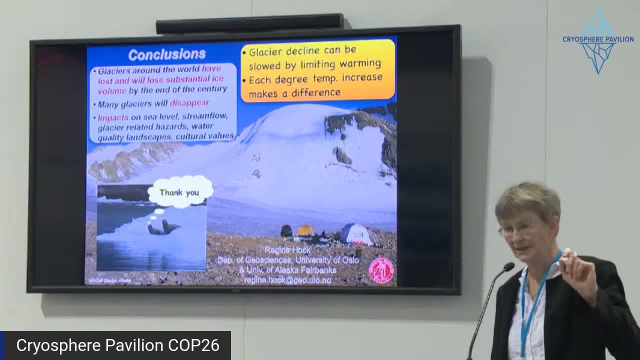 I mean, this was until very recently. There was mass gain or more or less stable, but the data shows that in recent years this trend is reversed and they're losing mass as well. now, Is there any way that you can contextualize? 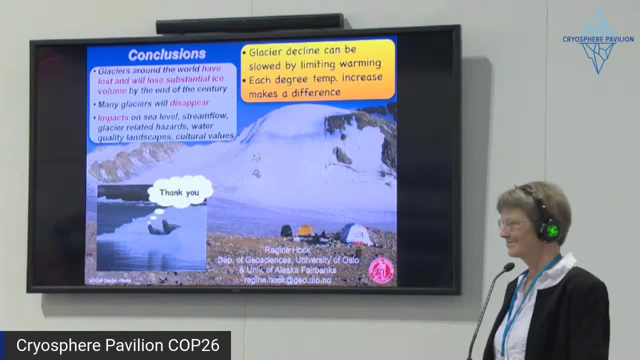 the amount of like the impact that the rising of the ocean is going to have by the end of the century. You talked about 17, like 8 to 17 centimeters, but how much is that really going to impact on land? 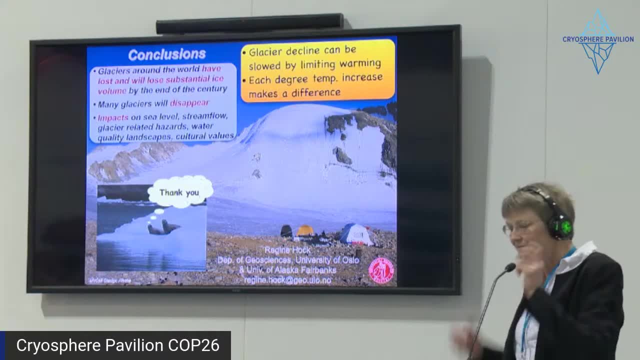 and is that going to displace a lot of people? Yes, I mean the impact of. there's, of course, an impact of the amount of mass gain, or more mean global sea level rise, but the biggest impact is the storm surges. 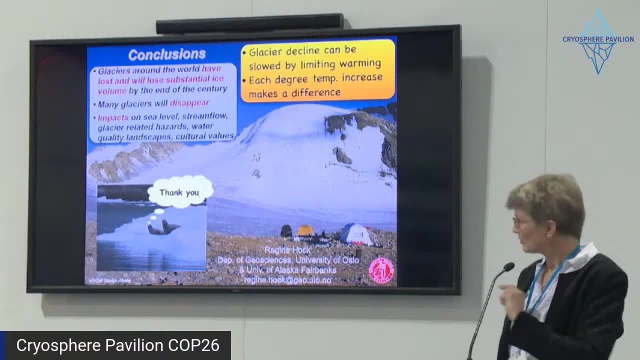 that with every centimeter of sea level rise- because that doesn't also here- the glaciers at the maximum can contribute 40 centimeters and that might not sound very much, but it is really the increase in the in storm surges and floods. 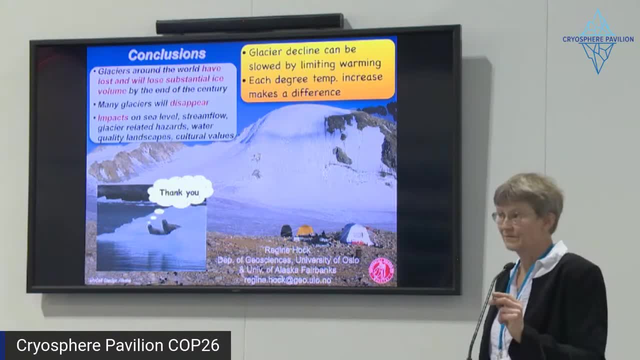 and events like that that will dramatically change In terms of sea level rise. do you know what the ratio is right now of the effects of thermal expansion versus loss of land ice and how that is going to be changing, say, over the next 50 years? 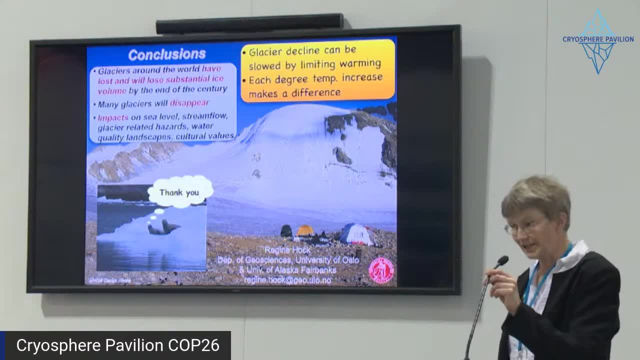 The quiet sphere contribution is the major contribution that was established, latest in the SROC report, IPECC report. More than half of it comes from the contribution of mass loss from the land to the oceans And of course, with the increase. 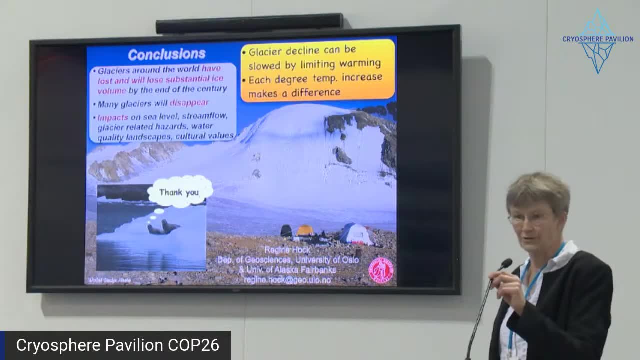 in glacier melt and also melt from the Greenland ice sheet and Antarctica, that contribution is only gonna rise. That's a relative contribution. What do you think should be improved in terms of observations to better constrain the projections for glaciers? That's a very good question. Until very recently we had only observations, so mostly. 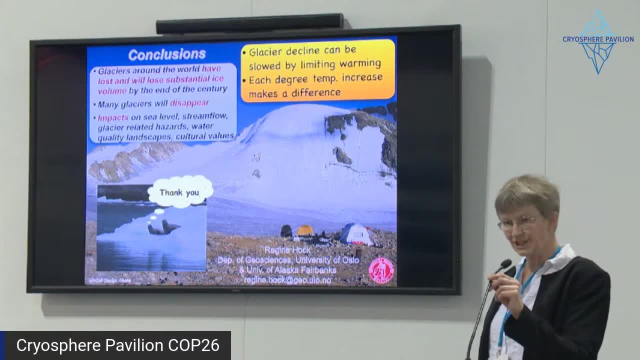 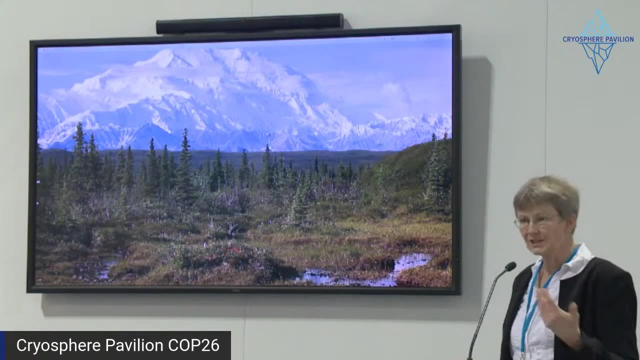 observations from the regions that actually have little ice, like the European Isles, Scandinavia, Western US, Canada. So with, of course, now the more and more satellite data, there is data also from the other region, but that is still, I would say, the biggest gap is. 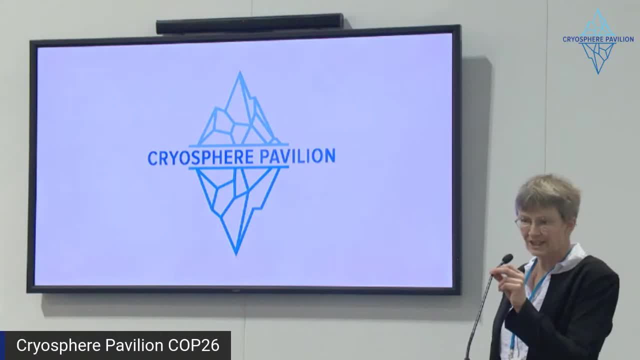 getting data from these inaccessible high polar regions, Also the glaciers around Antarctica, on the Antarctic islands. there's very, very little data to constrain it. Satellite data hasn't made possible any data So it's not possible to come up now with global estimates. but that's the regions where. 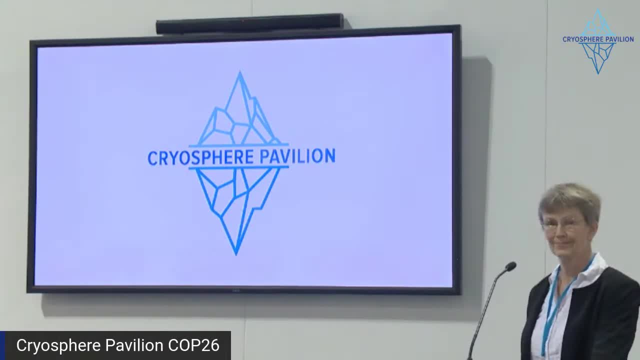 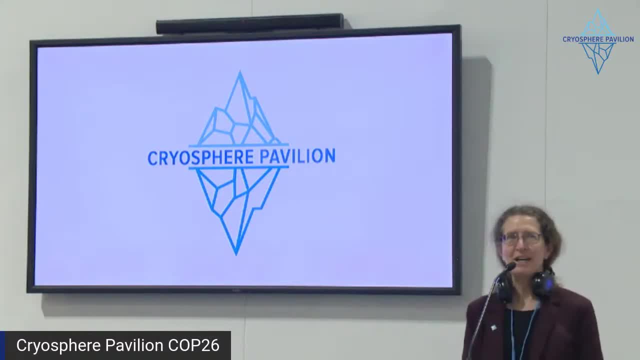 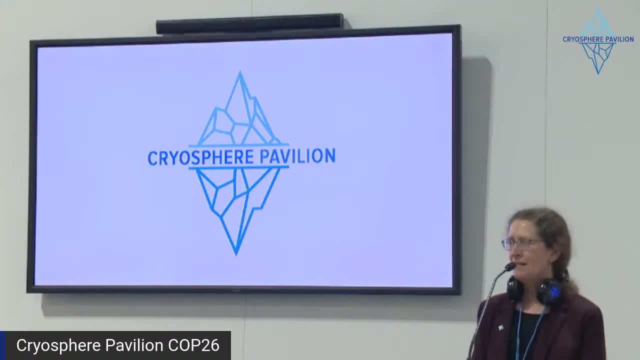 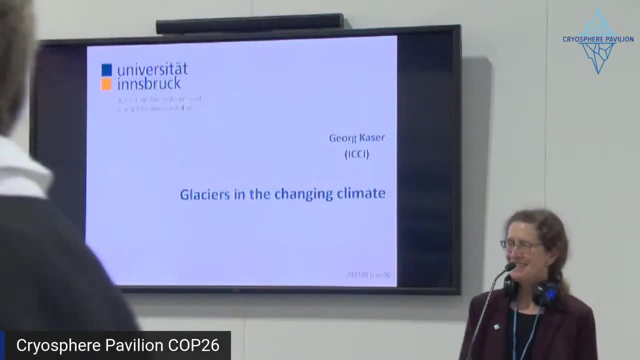 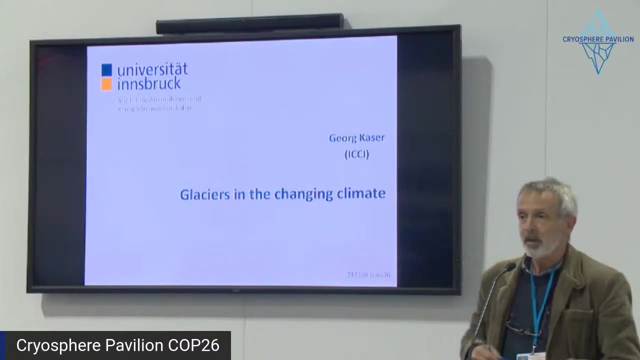 I would like to introduce Dr Gerrod Kooser, also an IPCC author, who would like to say a few words to add onto Regina, and then we can continue also this discussion with both of them. So, Gerrod, please, Thank you, Pam, and thank you Regina for having introduced the topic so nicely and 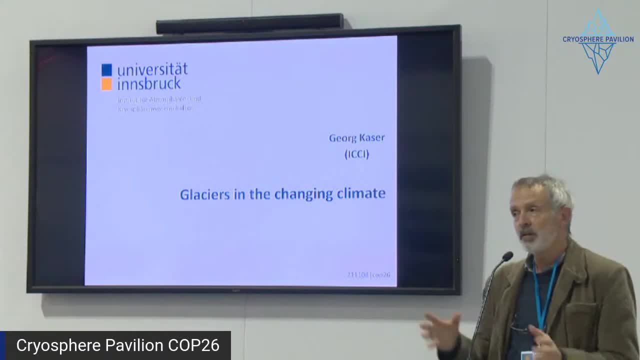 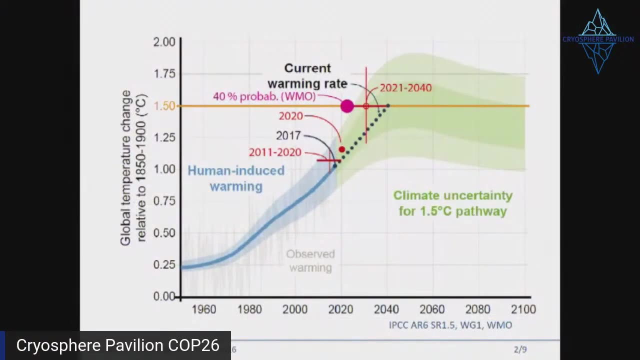 so comprehensively. I actually would like to shift a little bit the perspective on the same issue, And that is to have a view first on the Paris Agreement. There was a very nice picture actually in the frequently asked questions of the special report 1.5,. 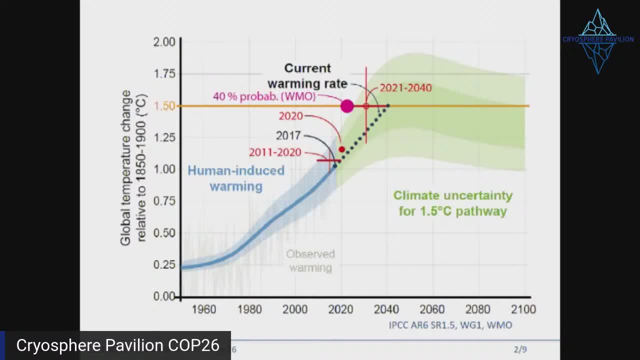 which gave the view on how we could manage to get to a 1.5 world. So the blue line is what was passed by 2017, when the report went out. The dark dotted line is the projection that would have meant by then that we penetrate the 1.5 by 2040.. 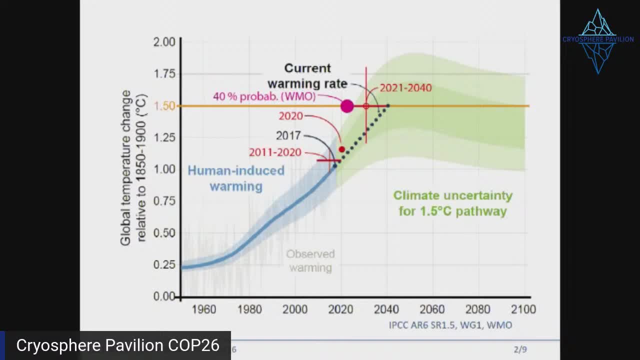 And if we would like to shift into a 1.5 degree world, we would have to turn the curve around along these green shaded areas, And that if we would do so, we would even avoid to penetrate a 2.0 degree world warmer. 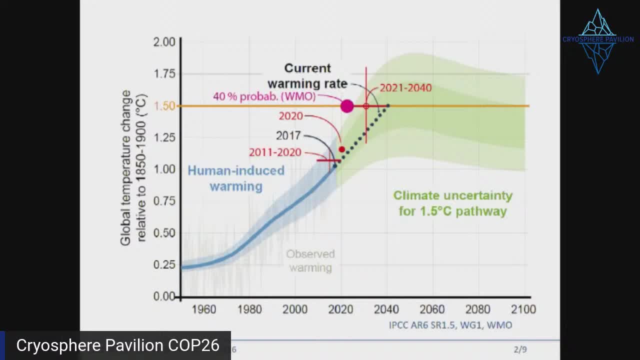 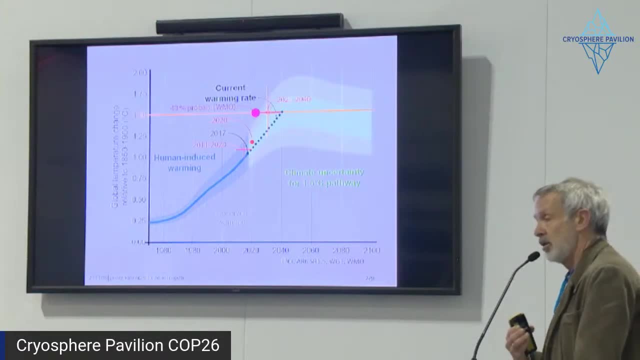 which I think we could all agree, that if we would go beyond that, or if the socioeconomic pathways which would drive us beyond this 0.2 degrees world, that would just lead into an instant unstable world, an instability in the climate system. 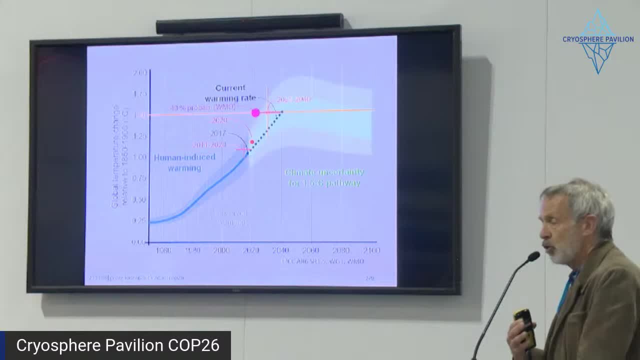 where we human beings would not be able to manage anymore. So we should try everything to stay within that 1.5 pathways. But the most recent numbers which came out by the Working Group 1 report Valérie has chaired for the last five, six years. 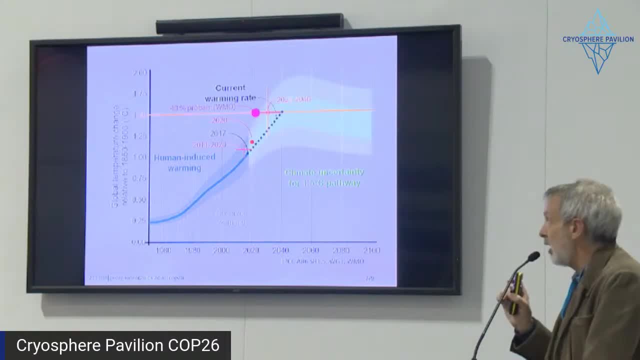 shows that by 2011,. the average 2011-2020, which is already measured and passed, is already to the left of that curve. If we then go into the projections, the IPCC projections for many, many model runs 2021-2040,. 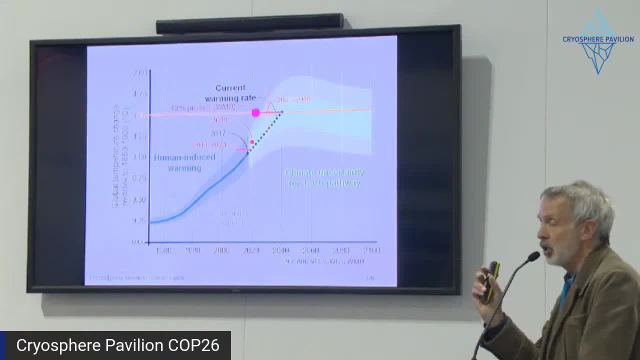 we would be much earlier crossing in an average, not in a single year, in an average day: 1.5 degree already by 2030, within nine years from now, or at least in that period which is centered around 2030.. 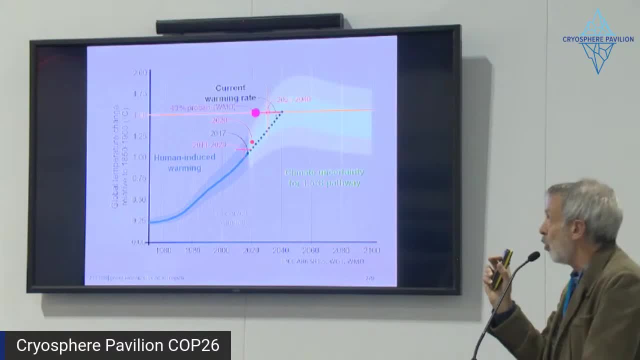 And the WMO has recently- just two or three weeks ago- upgraded their statistical projection, the probability from penetrating 1.5 in a single year before 2025, not only to 20%, as they have projected a couple of months ago. 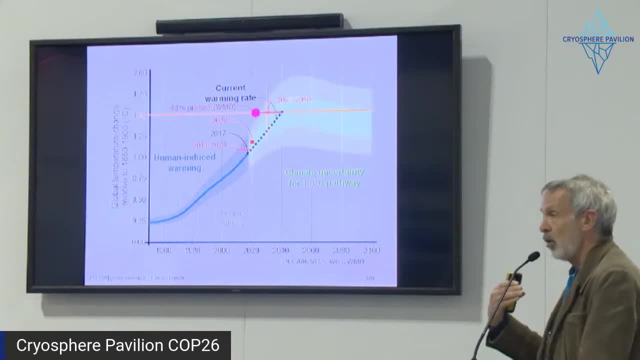 but now they go up to 40%. So the probability that we already passed that 1.5 degree is very, very close, at least for a single year. Then it may go up and down, but on an average that is something which goes much, much quicker. 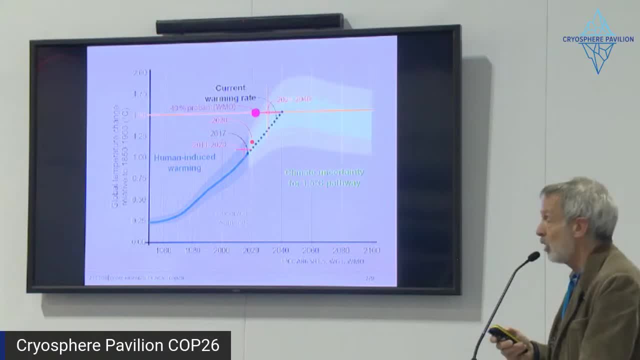 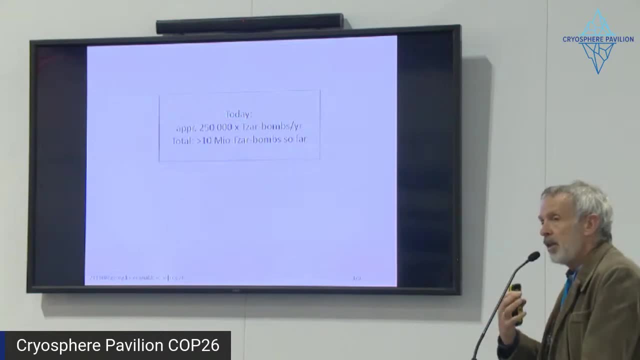 than we thought in Paris and we still thought with the 1.5 degree report. So this is a bit the setting Just to imagine what is behind these degrees. centigrades, degrees on a global scale, this is just an indicator of the energetic state of the planet. and not that much of a local or regional temperature. We can adjust. glaciers would adjust or do not adjust, but we put a lot of energy into that and only about 2% of that energy is used to melt ice. Most goes into the oceans. 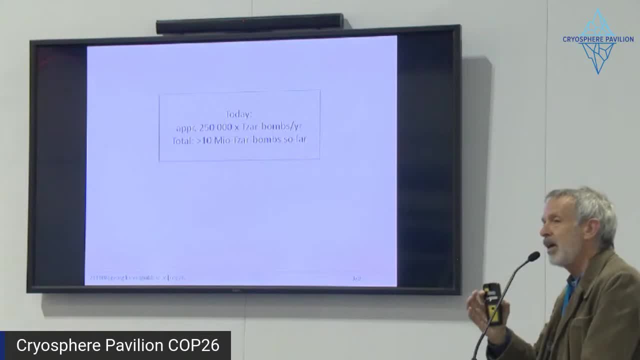 And I made a kind of a calculation which may lead us closer to comprehend what that means, And I have found the Tsar Bomb, which was the biggest ever blown bomb by Nikita Khrushchev in 1961, in order to show the US Americans that Russia or the Soviet Union is stronger than the US. That was the intent And that was a bomb which has never been blown again in that magnitude And that has had a tremendous amount of energy release, 3,400 times bigger than Little Boy which destroyed Hiroshima. 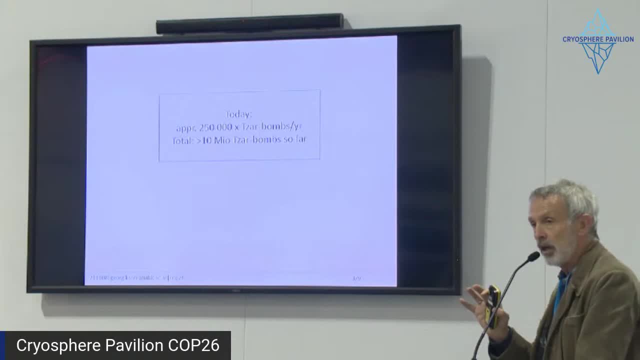 I do not talk about the radiation impact, just about the energy relief. And today- and today means that was 2012,. roughly It's slightly higher. now We are blowing about 250,000 of these bombs per year And in total, we have already accumulated. 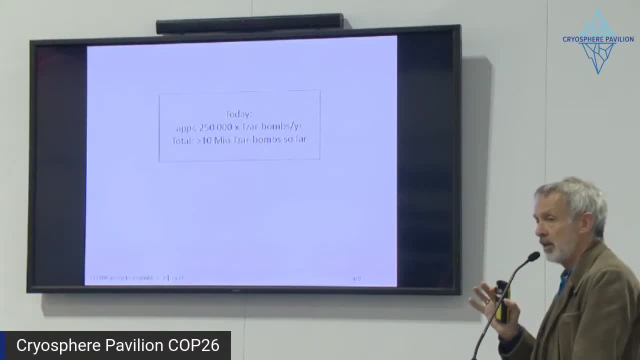 more than 10 million Tsar bombs, or the energy from 10 million Tsar bombs in the human climate modification. This is terrifying history. Not all stays in the system. Part of it is emitted again, but that is about the magnitude we have to talk about. 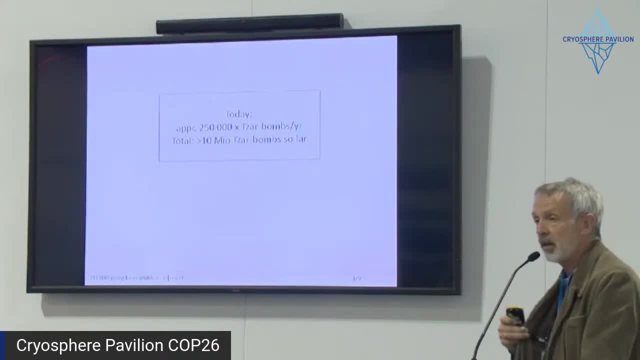 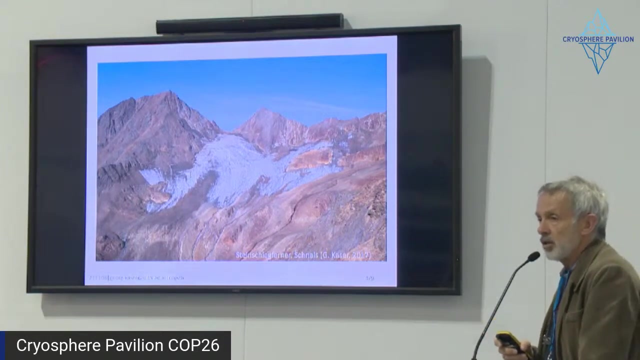 And this is the energy behind these tiny little degrees. Nobody would change a jacket for half a degree in the room or even a degree in the room. It is this energy which stands behind Many of the glaciers. Regina has said that we do not know much about the big glaciers. 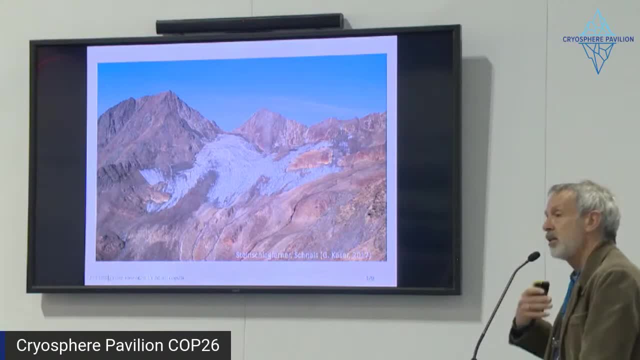 the very big glaciers. but we have also not very much knowledge- or at least is not introduced in the modeling- about these very tiny little glaciers. because if glaciers get this size they experience kind of a self-destroying mechanisms when they get dark, when the slopes get very dark. 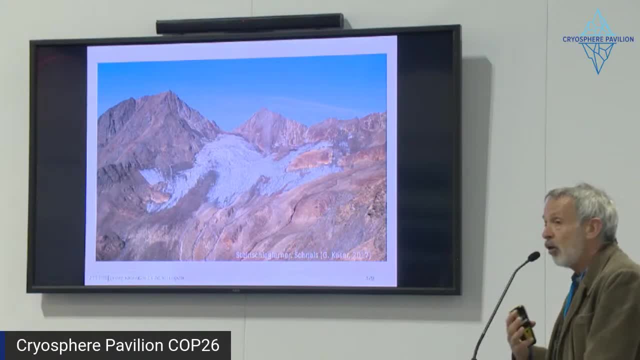 which can heat up in summertime very much, So they contribute much quicker and faster than healthy glaciers would do. We have all glaciers, or many, many glaciers around which are already dying, And dying glaciers are much quicker losing mass than healthy glaciers. 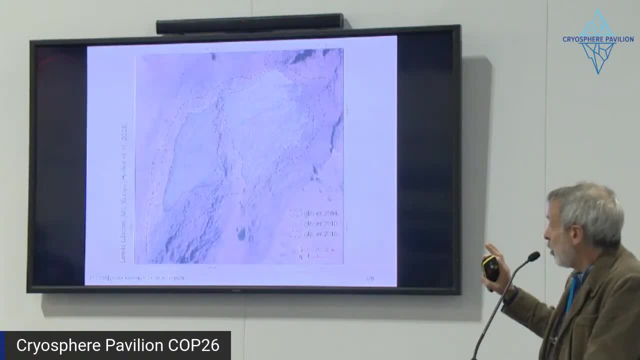 This is, for instance, Louise Glacier from 2004 to 2016,. the last glacier until very recent on Mount Kenya in Kenya. And you see, as soon as these barriers, these rock outcrops come out from a glacier, the disappearance of the glaciers accelerates very, very much. 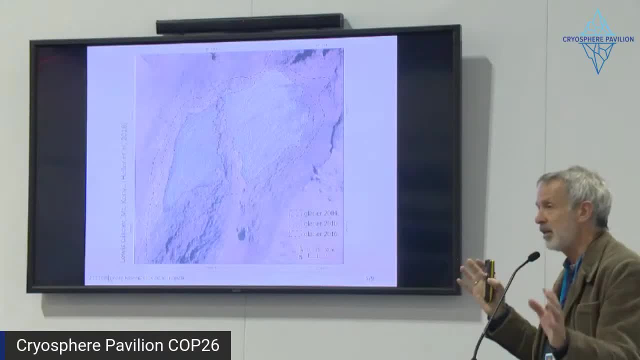 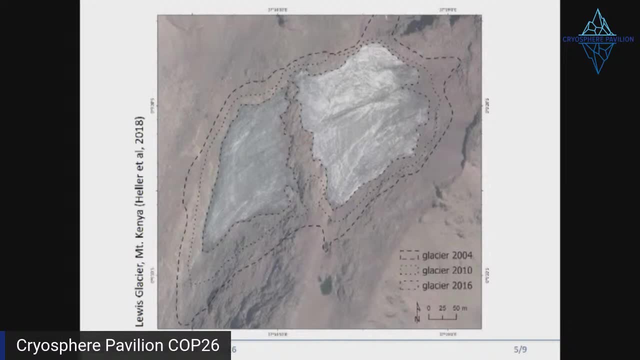 As soon as you have one rock coming out, then the glacier is basically lost. This one in 2016,. this barrier came out and a few years later it was gone. There is only very little ice left. Now back to Paris. 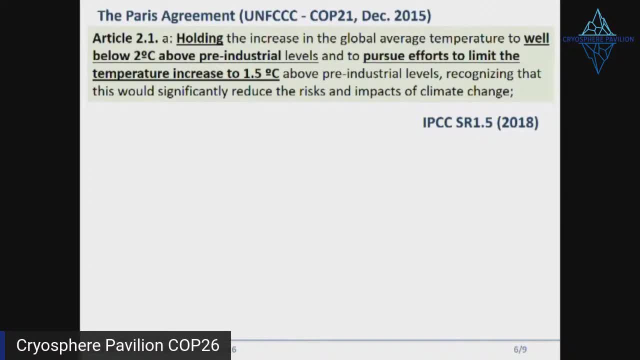 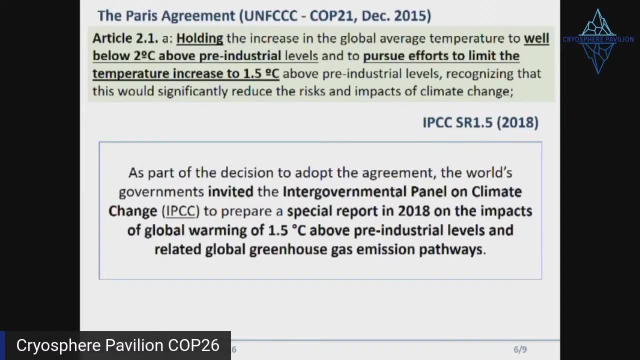 There was this agreement, everyone knows. but there was an add-on to that which made scientists, first of all Valérie, very, very nervous. That was, as part of the decision to adopt the agreement, this 1.5, possibly 2 degrees. the world's governments. 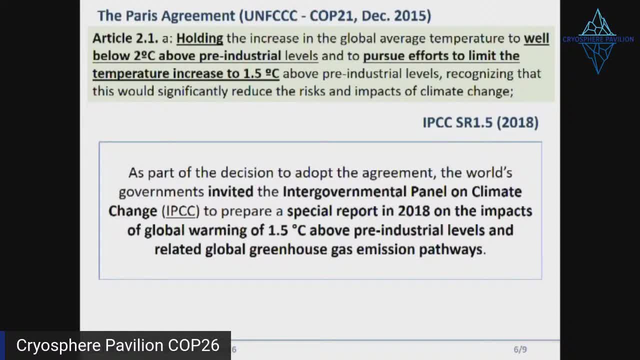 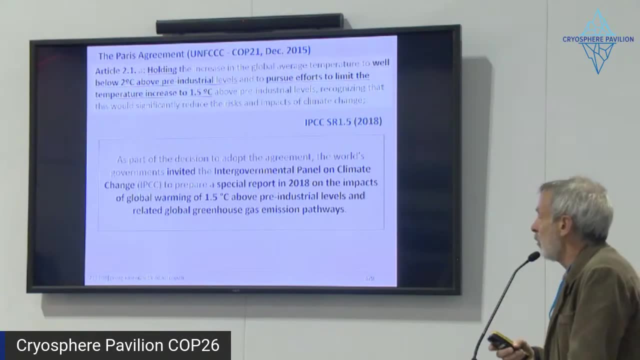 invited the Intergovernmental Panel on Climate Change, And I always add to say: invitation means you have to do it, do it and do it quickly. So we were invited to prepare a special report by 2018 on the impacts of global warming of 1.5 degrees. 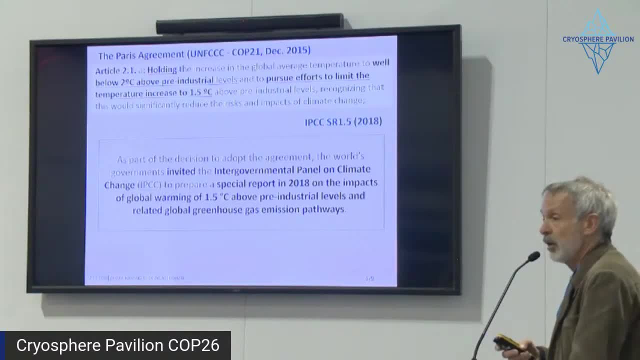 above pre-industrial levels and related global greenhouse gas emissions pathways. This was then this famous SR 1.5 degree report, Which came out by about 90 colleagues around the world, which did a tremendous work in this short time, And it came out in time in October 2018.. 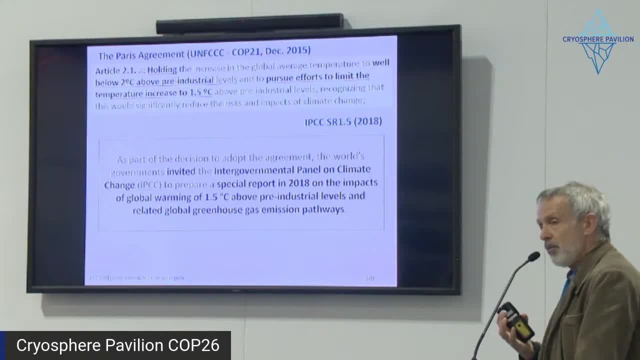 When we were standing around in Paris. by then, many of us were very nervous because there were no models which could help us. They were not available. We had only these 2-degree models, No 1.5 scenario, not even the socio-economic scenarios. 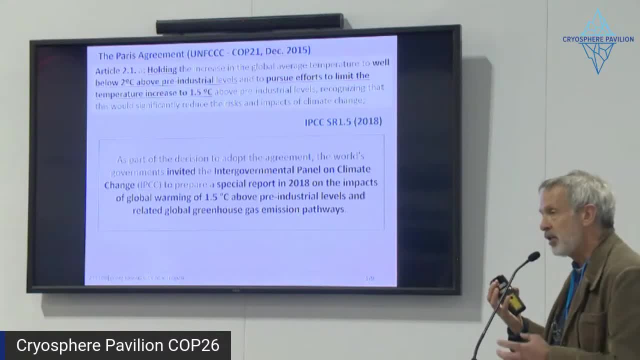 Nothing was available, And we knew that the precision of our models would not allow us to go for 1.5 degrees by then. But there was so much improvement since then that it was possible to do it by 2018.. And it was still in Paris. a situation like that. 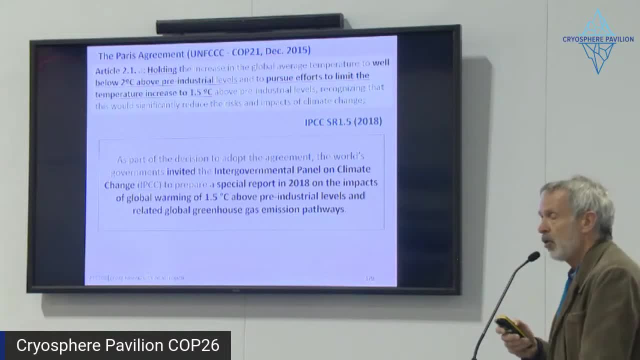 I picked up my phone and sent a message to my colleague, Ben Marzeon, back in Innsbruck- Many of the figures which have been shown right now were from Ben- and said: you have to do something, We have to do something. 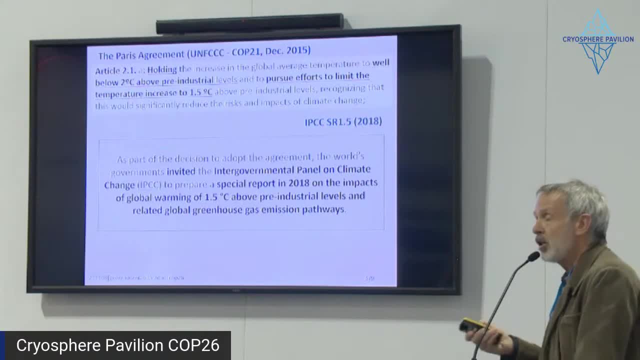 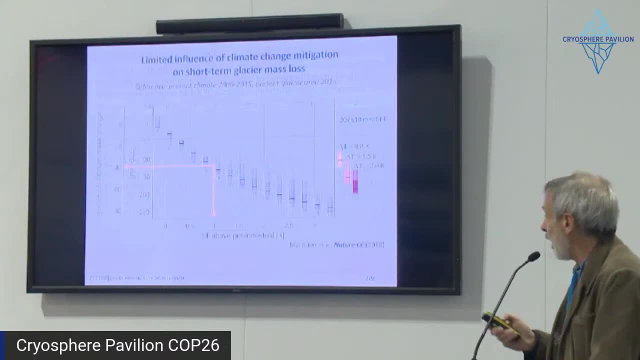 I come back within a week and we have to prepare something on glaciers in a 1.5-degree world. And he said, oh, it's impossible, we cannot. I said you have to do it And it took a little while, until 2018, until it was accepted. 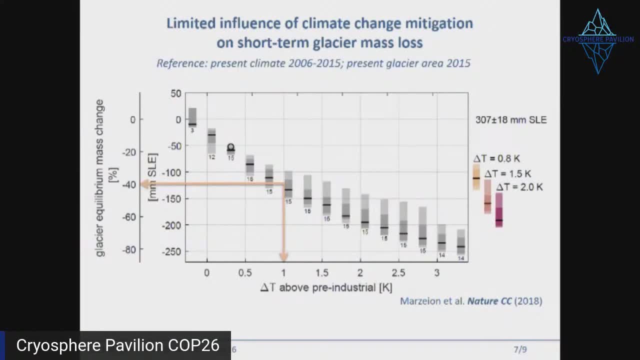 But this was the overall figure And it shows on the lower axis, the horizontal axis, different temperatures of global average temperature. So by then we said 0.8 was Paris. we go down to 1,, 1.5,, 2,, 3, and so on. 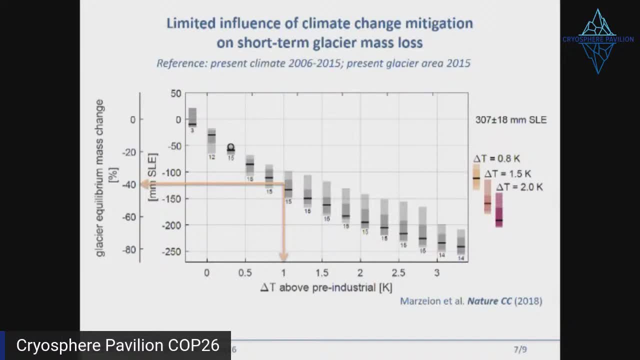 And that was put on glaciers, the glacier area and the glacier mass of 2015, which was available by then, and the climate of 2006 to 2015 as a starting point And if we go, no matter when, into a 1-degree world, 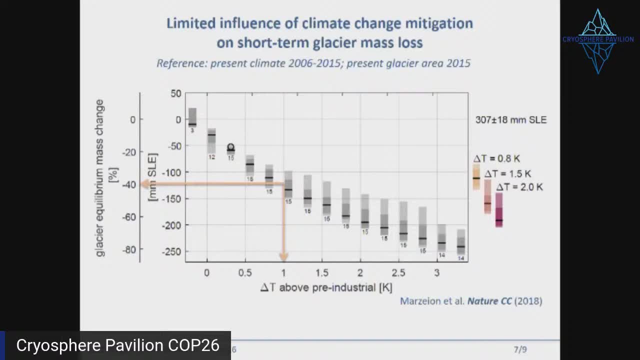 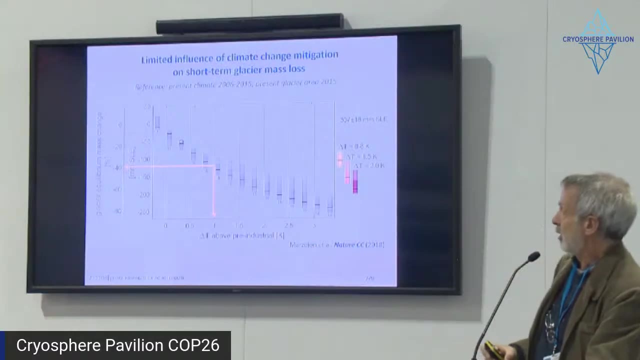 which we have already reached now, and we go into a 1-degree world, which we have already reached now, we would stop that world and wait until all the glaciers have adjusted worldwide. Then we would lose about. this is the left. The left shows that we would then lose 40% compared to the 2015 of all glaciers. 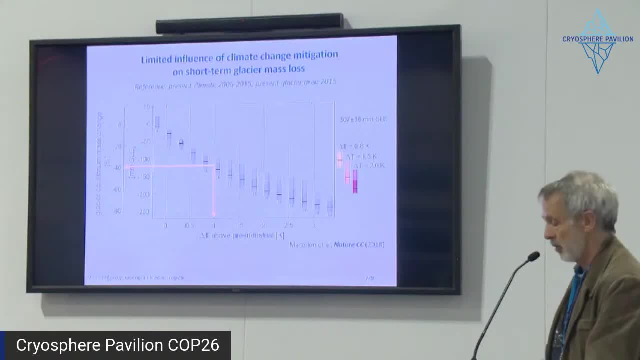 which corresponds to about 12 centimeters of sea level rise. If we go into the 1.5 world, the main target of Paris, we would lose about 50% and we would add about 15 centimeters to the sea level. 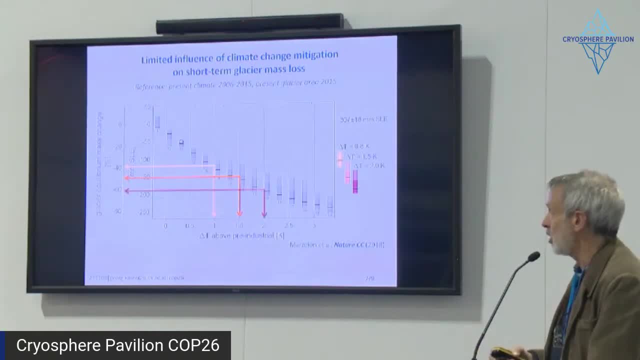 If we would go to a 2-degree world, we would lose about 60% of all glacier surface, glacier mass, and we would rise the sea level by about 20 centimeters, just roughly. But then he was a very- he's a very- curious person. 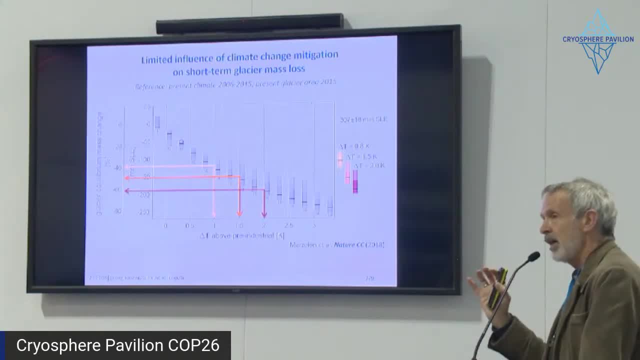 And he said: what if we? or how does this translate into a one kilogram of CO2?? How much ice would we melt, or how much smaller would the end mass be if we add one kilogram of CO2?? And that would be 15 kilograms less. 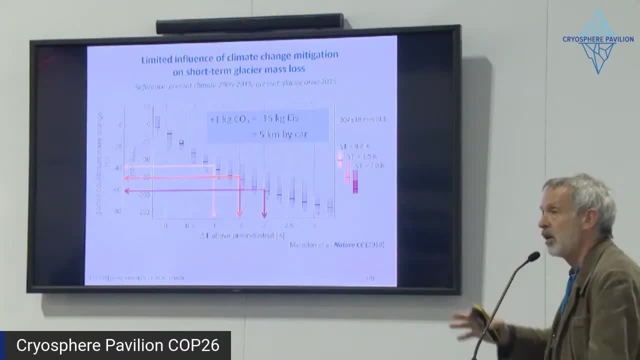 And if you go with a kind of ordinary car, not the big ones, you would emit this one kilogram of CO2 by driving five kilometers. That was an extrapolation from this, from this budget figures. we have a certain budget and then we reach a temperature. 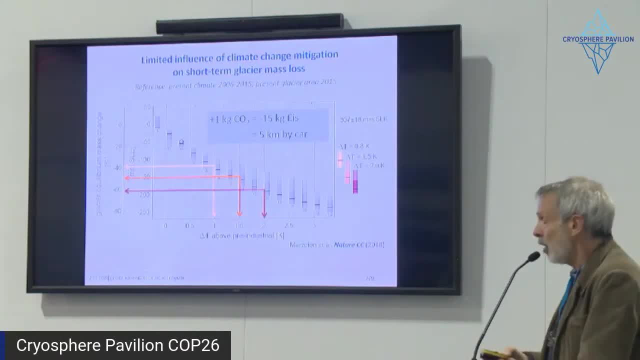 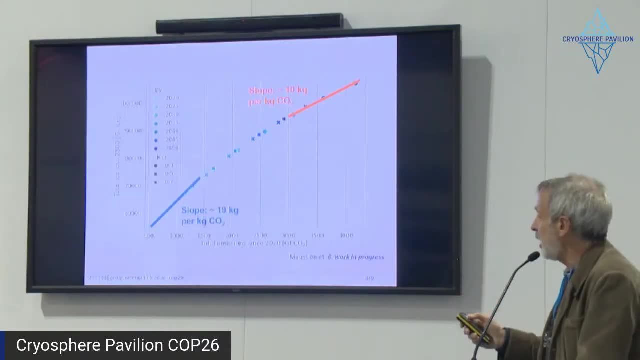 That was a very rough extrapolation And recently one of our younger colleagues, Fabien Massot, did this curve. I do not explain it in detail, but he came up with an even stronger number. For the time being, if with a given surface area. 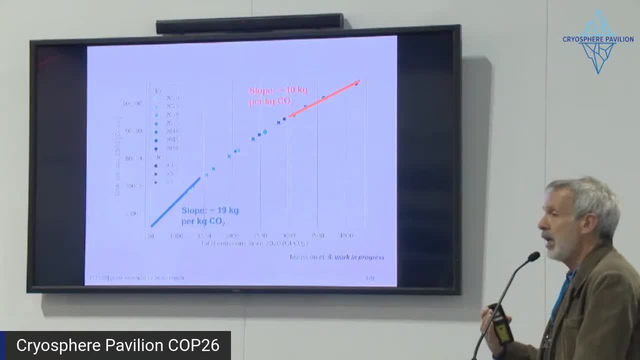 by one kilogram. driving five kilometers would mean we melt 19 kilograms of ice, not just 15.. So this is a more sophisticated approach, And only if the glacier surface area gets smaller and smaller we would also reduce the impact. Of course, the smaller the glacier is, the less damage you can do. 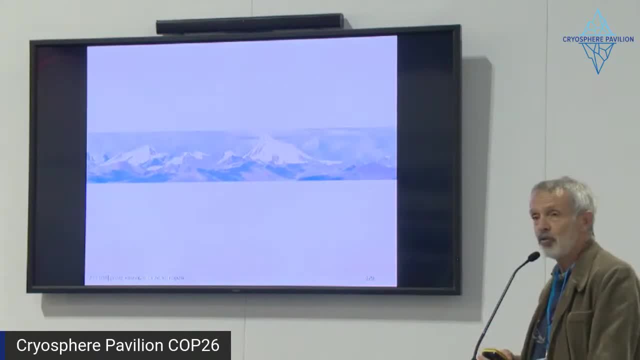 I think that's it. Yeah, it was an instantaneous contribution and a slightly different view than Regina's view, And I hope this has stimulated a bit of thinking. also on a personal level. If there are any questions to Regina or myself, please feel free. 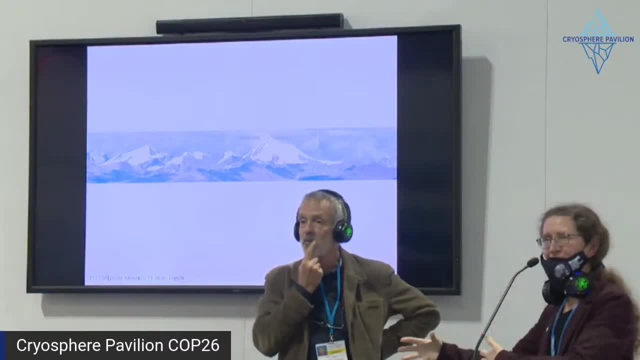 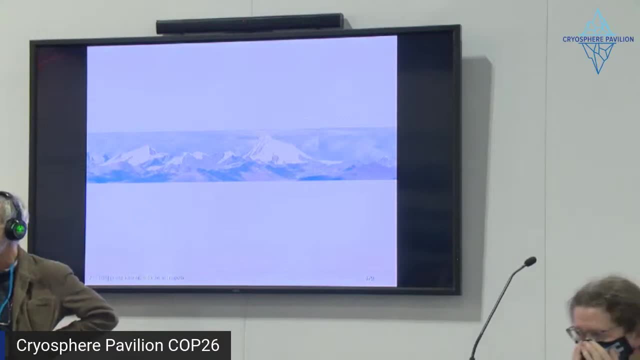 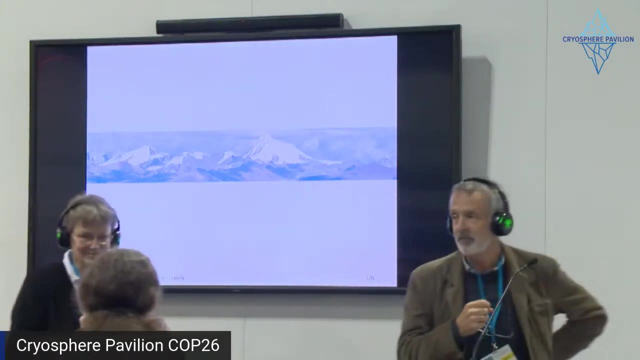 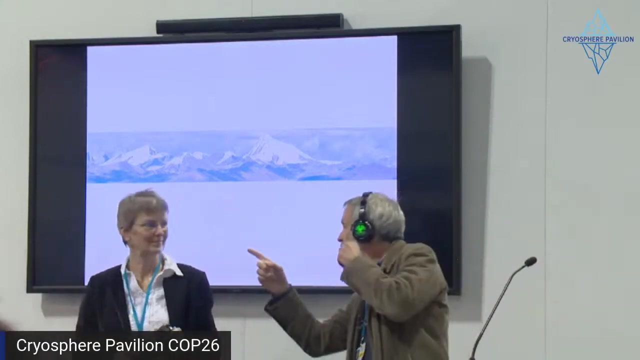 How about I suggest that Regina and Gorg sit up here for a bit and simply take questions? If you have any questions, please feel free to ask them. I'm sorry, I'm not sure I'm able to get through to you. I'm sorry, I'm not sure I'm able to get through to you. 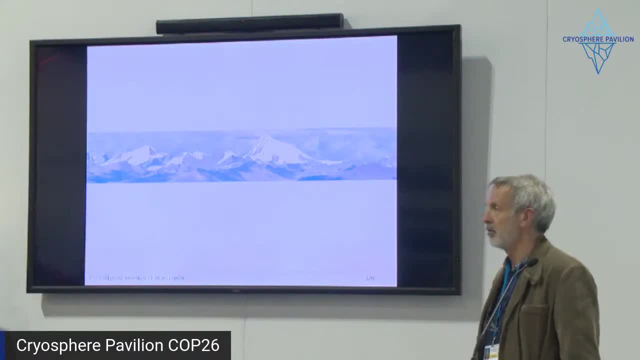 Sorry, I'm not sure I'm able to get through to you. Sorry, no, thanks. so much for that. Just a quick question which is around: Can you just confirm what you're saying? is that the 1.5 degree scenario? 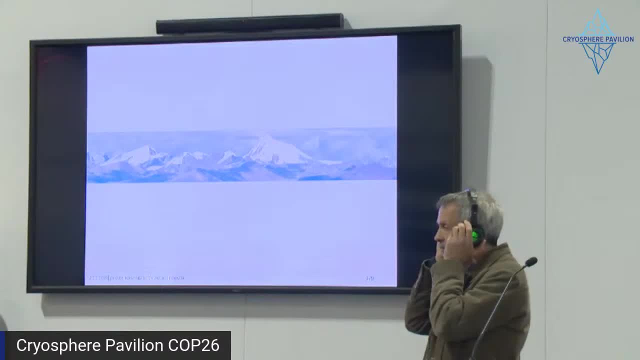 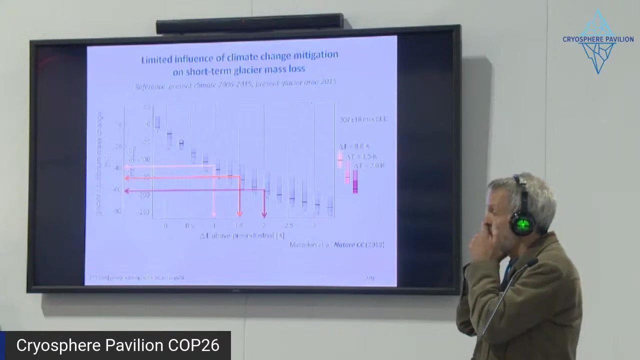 does that bake in? 50% decrease in glaciers and a sea level rise of 15 centimetres? That's just a given. And is that then put into the models that people are using around? Yeah, that set of things, It's really just around the scenarios that governments are using. 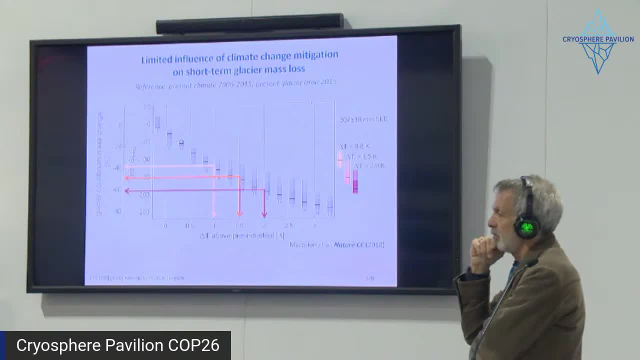 to then look at things like sea level, rise around cities and things like that. Is that all being done at present? If I understood correctly, yes, these are the numbers within the given uncertainty. If I understood correctly, yes, these are the numbers within the given uncertainty. 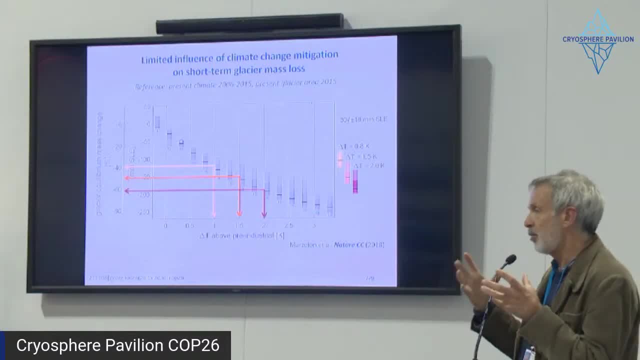 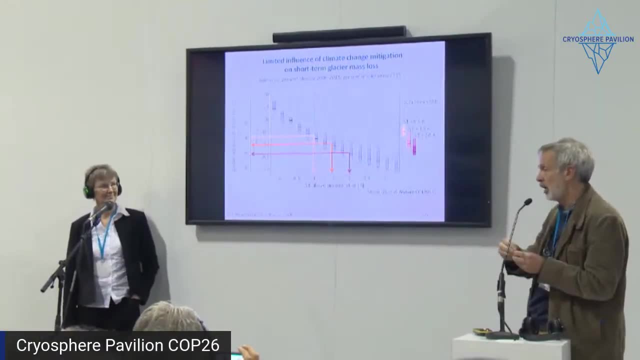 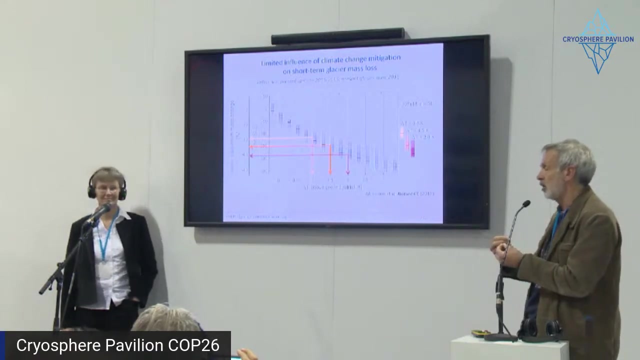 If I understood correctly. yes, these are the numbers within the given uncertainty Of such models And, as I explained, there were a few steps to be done by then. Nowadays we can really go into the model chain from the beginning, from the socio-economic behaviour into the emissions. 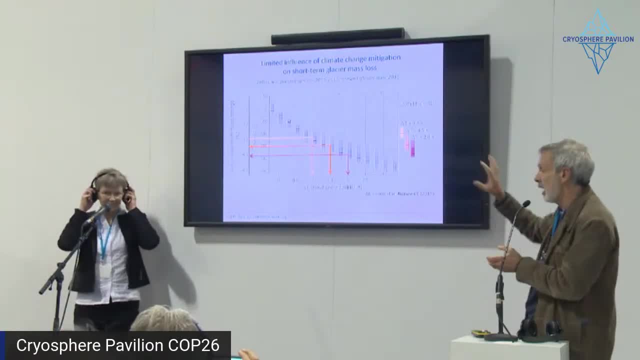 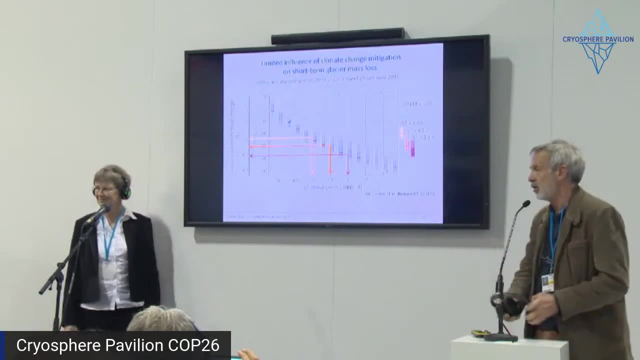 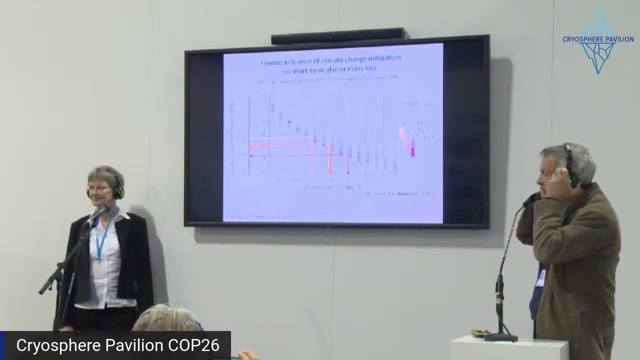 into the temperature, regional temperature developments and then project. But it is basically the numbers. The numbers are there, And what was the second part of the question? Yeah, it was really just about whether governments are looking at that in terms of the scenarios around timescales for sea level rise. 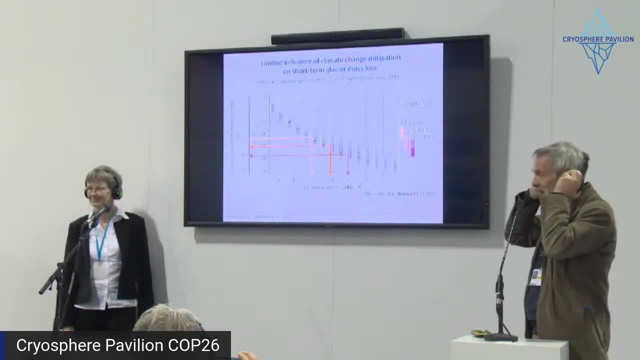 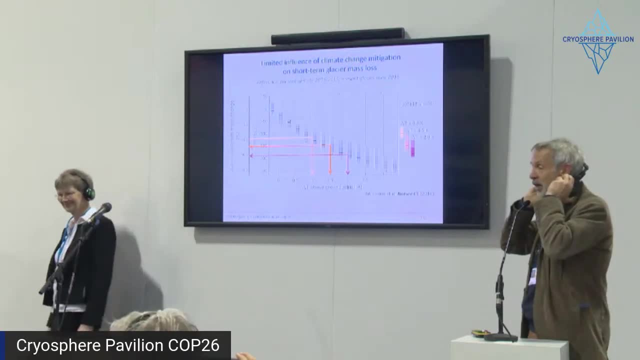 to do with cities really more than anything else, and coastal areas? The simple answer is that I have no idea what the governments are doing. Valérie may give a proper answer. She is in much closer contact to governments than I be. She is in much closer contact to governments than I be. 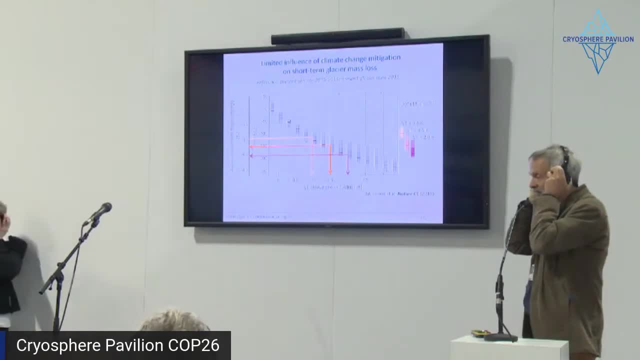 She is in much closer contact to governments than I be. The response of the Glacier is that. The response of the Glacier is that. The response of the Glacier is that The response of the Ocean Expansion and the response of the Ice Sheets is assessed in our Working Group. 1 report. 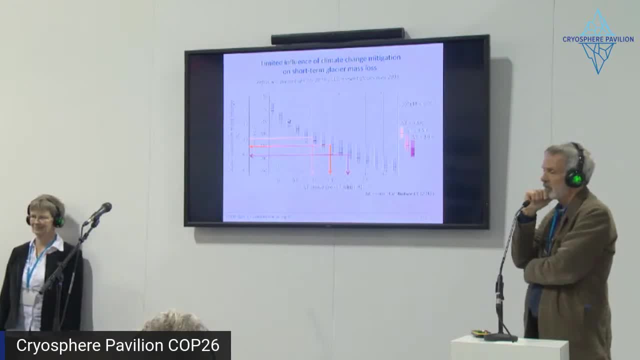 When you look by 2050, the projections for sea level rise are almost independent of the emission scenarios because of the committed responses, from the snow component in particular, And by 2100, they depend a lot, by a factor of two, on the emission scenarios. 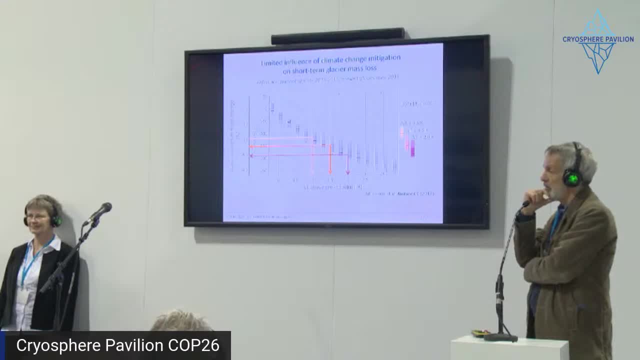 and what happens now and in the coming years. and what happens now and in the coming years. And we've also considered in the sea level projections the possibility for abrupt collapse of sub-sectors in Antarctica which are associated with low likelihood but could potentially strongly increase the amount of sea level rise. 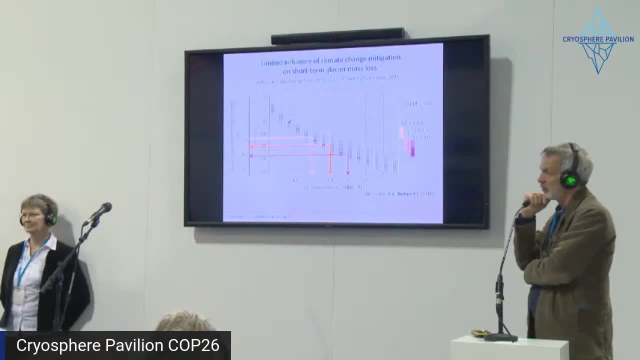 by this century and other ones if it is triggered- And this information was asked especially to us- by those involved in critical infrastructure management Because, for instance, when you design the protection for a coastal city or a harbour, you take a hundred or sometimes multi-hundred year perspective. 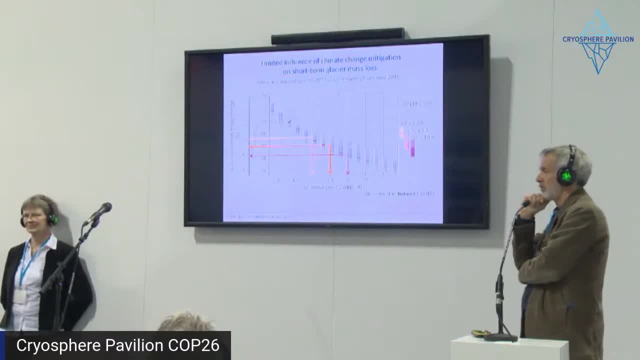 So, for instance, for a city like New York that was exposed to heavy floods in the last decade, this type of information has been considered And, as Regina stressed, the importance of sea level rise is not just for the mean trend For about two thirds of the coastline. 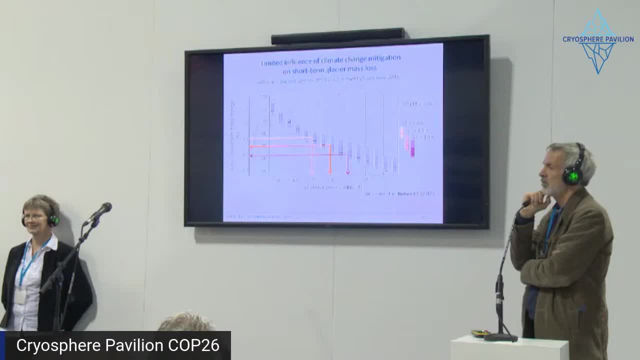 the regional sea level rise. the sea level rise is close to the global average, But it's also how much it affects coastal erosion and extreme sea level events, their peak and their recurrence. So this is also something where glaciers play a key role and which is included in the assessment of the implications of sea level rise. 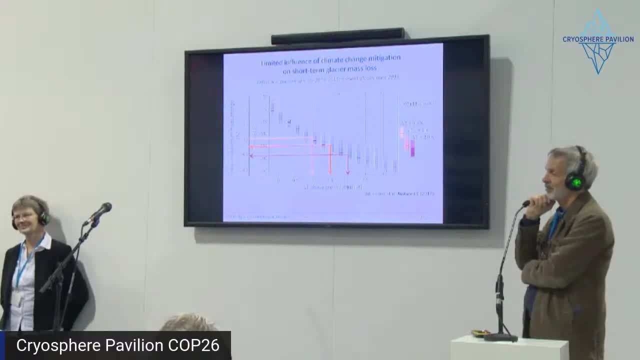 So you can help us check what decision makers are using and bring to their attention the latest science. That's also very helpful. You can, by the way, see the figures on this panel over there, And this is part of the report. Pam and her group. 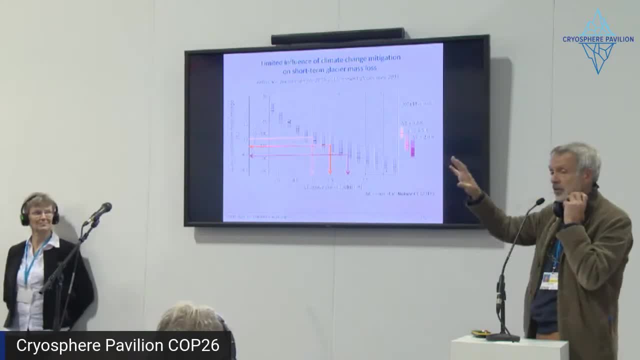 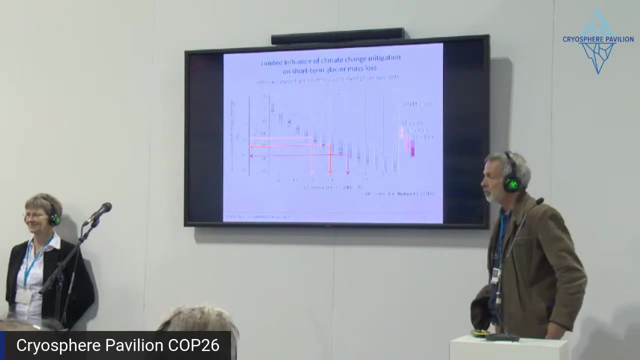 has prepared for this event. here There's a lot of information also on sea level rise And you can see, I think, the New York City area, It's just over there. And if I could just clarify, because I'm one of those who's trying to at least communicate this to policy makers, 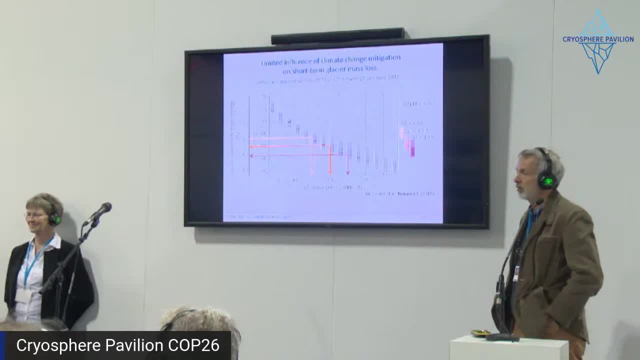 when? and, Valerie, please correct me if I'm wrong, but my understanding is that when the IPCC says low probability, that means, especially in the case of this potential collapse of the West Antarctic ice sheet, it means very few studies. It might actually be, especially at higher temperatures. 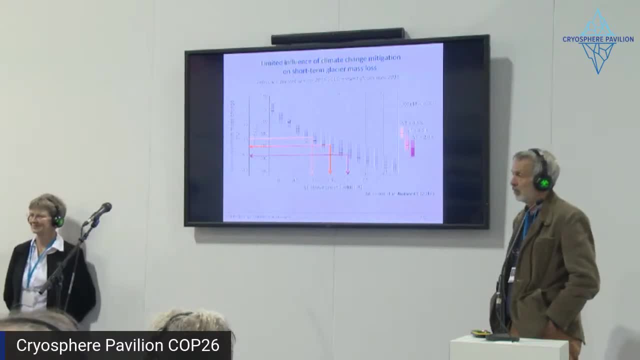 a lot of the ice sheet. scientists feel if we go especially above two degrees, it's a high probability and we're more talking about the rate. but it's an area of very, very active research, as you can understand, because that's rather important. 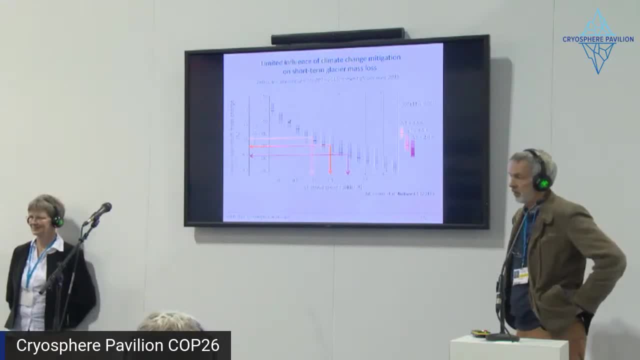 because if you look at some of these panels here, the dotted line that was in the summary for policy makers was going very much straight up and would end up by 2300, up to 10 meters of sea level rise, just from Antarctica in a worst case scenario. 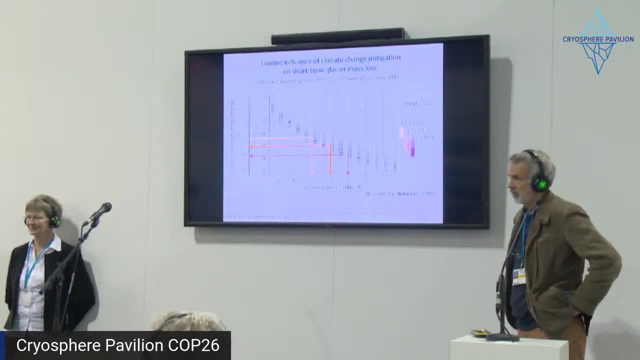 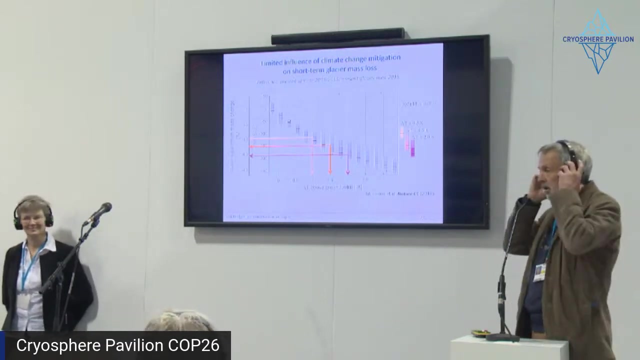 So these are highly impactful consequences of continued high emissions, which is the path we're on right now. Other questions, please? Or commentary on what I just said? I will say also, though, and I think this is important when talking about glaciers: 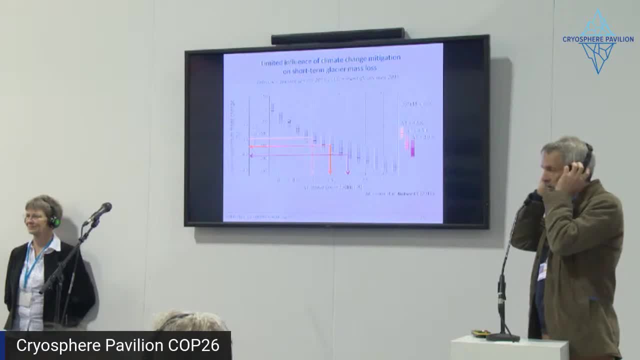 ice sheets. the main contribution it really is going to come from the ice sheets, But locally they are so important for power generation, for water supplies, for agriculture, especially in some of the places that Georg has studied, for example in the Andes. 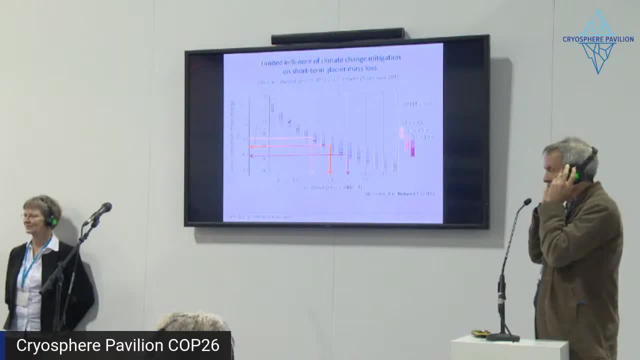 And I would say, would both of you agree, maybe the Indus and perhaps the Tarim Valley in China are two of the most vulnerable areas And there are millions of people living there. Agriculture, this huge agricultural area in China, is just tremendously vulnerable to loss of glaciers and snowpack. 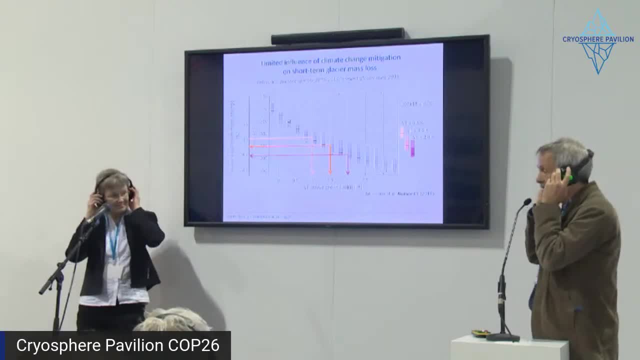 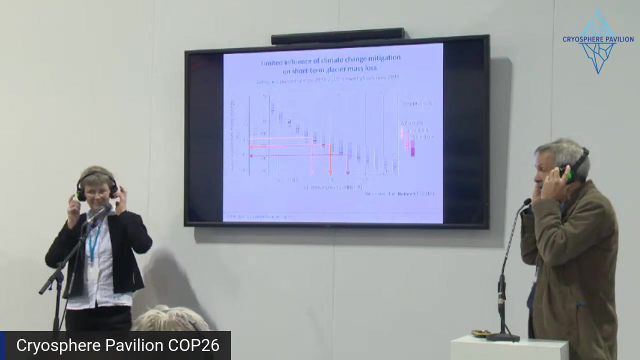 I think talking about agricultural vulnerability is also the solidification of the estuaries. In addition to the high waves, this is one of the most threatening scenarios I could think of, when we have just a collapse of agricultural area in many regions. And I think just to add on this probability issue, 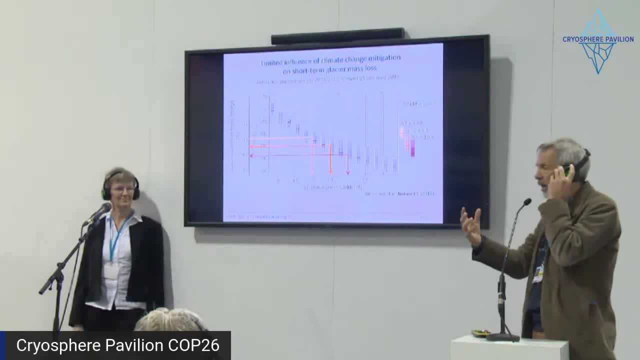 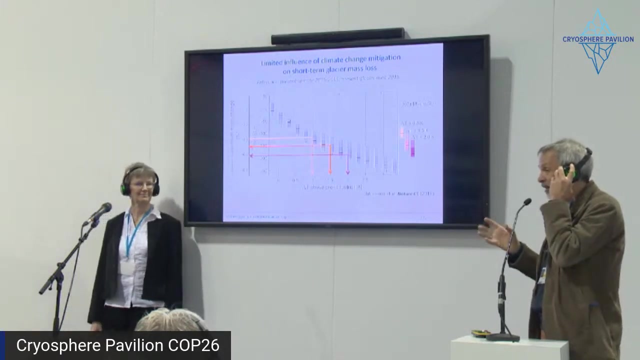 statistically the probability is not very high And that's why it is named low probability. But physically I see already the first signs. Maybe it is not happening, or happening a little bit slower than the worst scenarios are, But low probability is kind of a rather dangerous term, I would say. 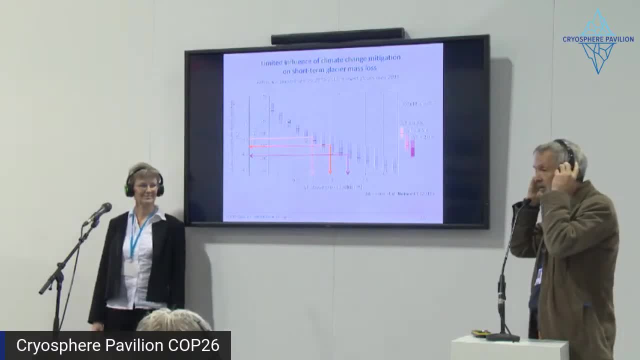 which we cannot change anymore Once such a term is out. it's like the social distancing That's the most stupid thing I ever heard. It's a physical one, not a social one. I just want to add to the agriculture and runoff. It's the timing for agriculture, So it might be very, very little changes sort of in the absolute amount, But if the water comes at the wrong time- because the glaciers melt in August and July- if it comes at the wrong time then it can have a huge impact. 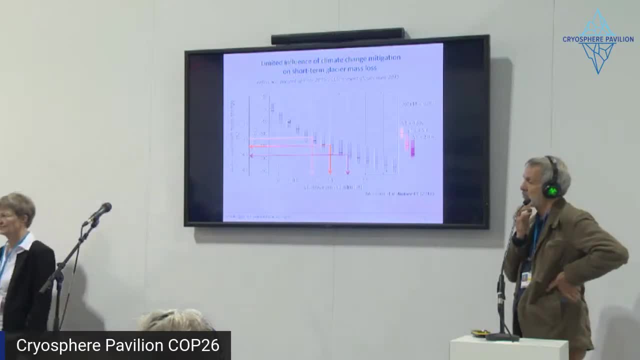 even though the change in itself is very small. I think, if you come here at 4pm today, when there will be a very large Swiss event jointly with the Swiss Hub, if I remember correctly and correct me if I'm wrong- but one of the findings 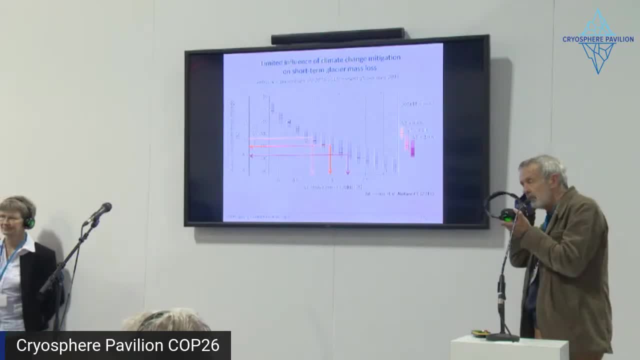 there is that the peak water, or the water runoff on which agriculture is dependent in Switzerland, will shift from August, when the farmers are very reliant on it, to June, when they don't need it as much, And so even a shift like that in timing is going to have a huge impact on agriculture locally. 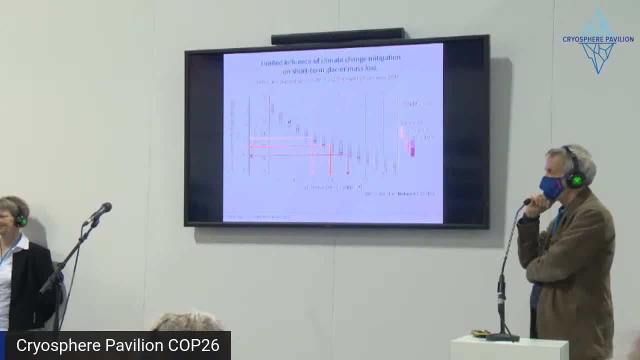 So thank you both for your talk And so thinking about. maybe we are not going to be able to reduce emissions now because our system is based on economic things And so maybe, yes, glaciers are going to disappear and to lose 40 or 60%. 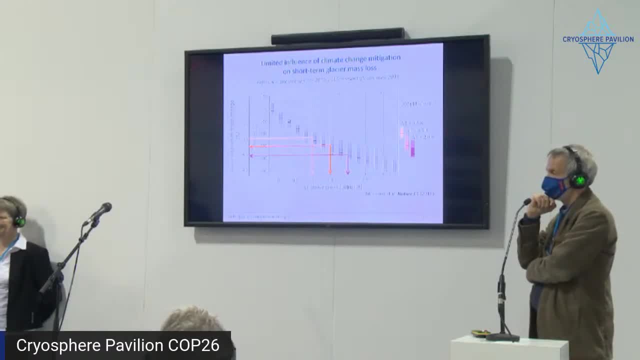 So I would like to think about more local based adaptation strategy, or maybe mitigation strategy. What are your thoughts about what can we do in mountain system to maybe reduce sea level rise? just maybe trying to store water in the highlands? Or what can we do to adapt from now? 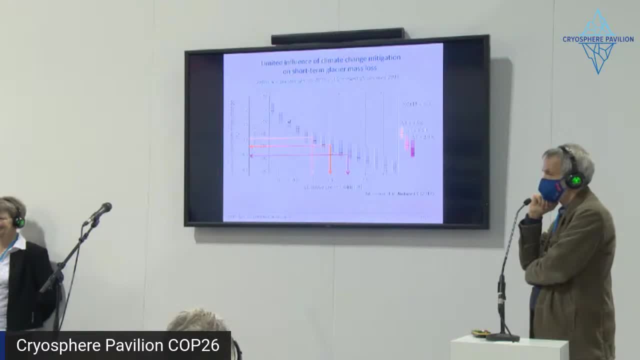 thinking that we are not going to reduce this emission because, unfortunately, like we have to change a lot of things in our economical system to do it. So yeah, it's my question: What can be like a very local, for example in the Andes, to continue to live in high mountain system? 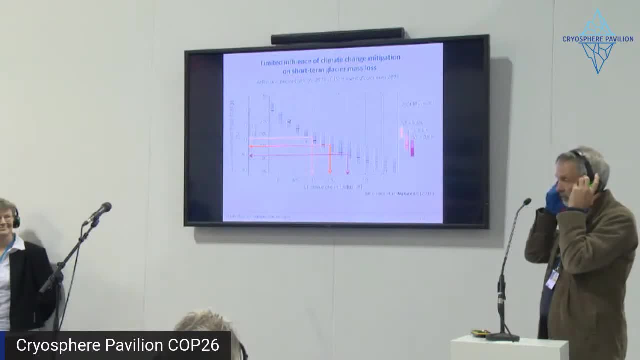 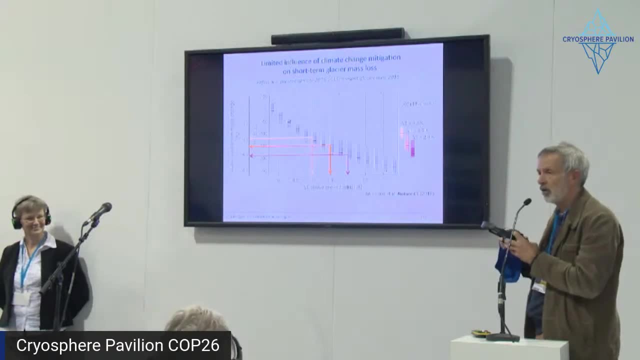 without having to migrate. I think we have to reduce the emissions and we will reduce the emissions. If we do not do it by design, it will be by disaster. So the emissions will be reduced By disaster. we do not like By design. we are obviously not able, but there will be some changes. 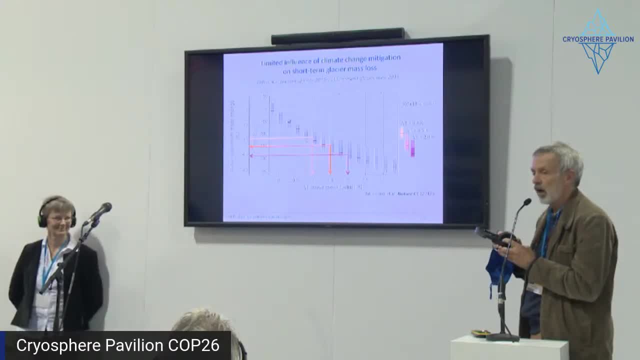 and tremendous changes. I'm rather sure. As for how people can adapt, I would just give it back to you. wait for your thesis to come out and then we will know. But there are studies out on different locations, different regions. 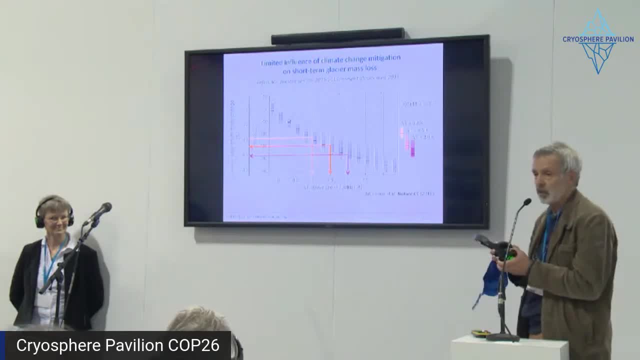 because every region has its different circumstances which have the ability to adapt, have the necessity to adapt, and particularly mountain regions that I think Regine can tell more about the mountain regions as a coordinating lead author on the mountain chapter. But there is a lot of work out there and many, many different solutions. 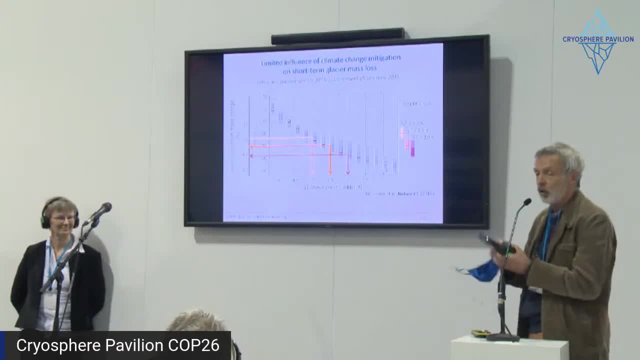 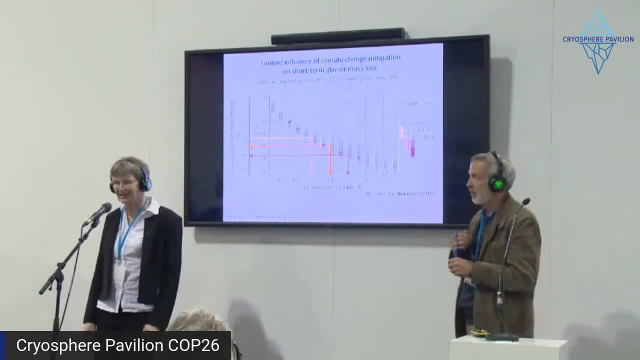 as in such complex changes will always be requested, But go on and tell us as soon as possible what you find out about the Andes, Maybe just to add. I mean, the impact, as I've tried to show, are multifaceted. 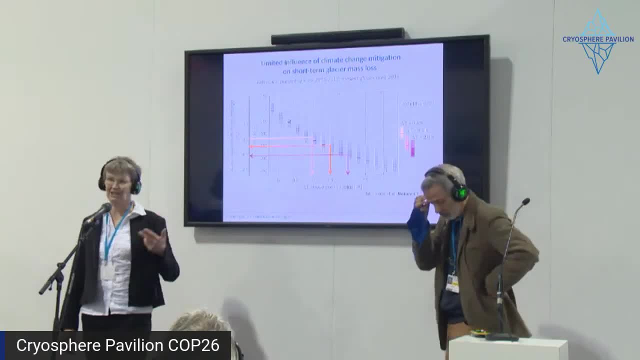 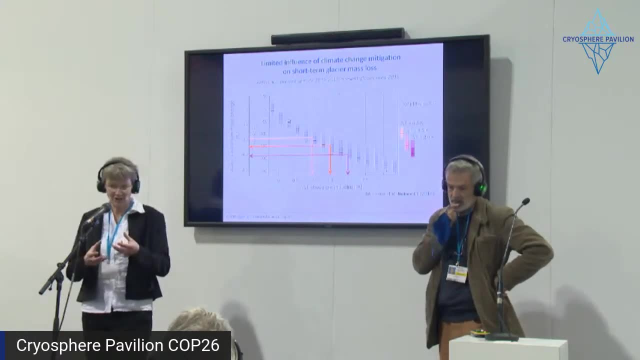 I mean there's so many impacts, from sea level to runoff, to hazards, to landscape changes, to changes in the water chemistry, So the adaptation and mitigation I mean it has to be locally adapted to whatever the issue actually is. The glacier change can have like totally different impacts in one valley. 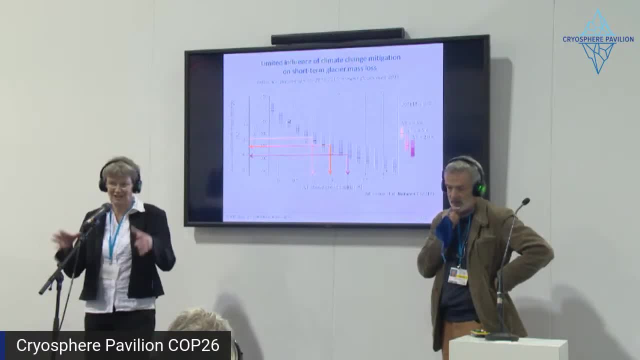 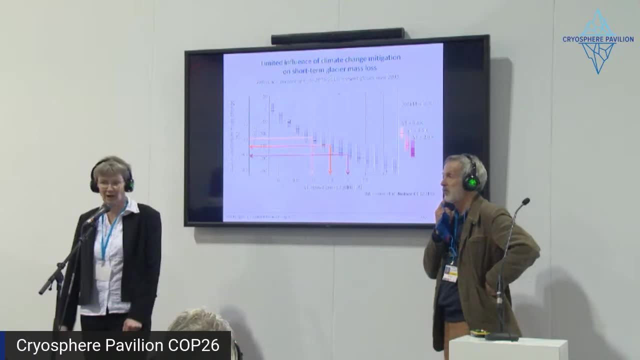 and the neighboring valley. it's a different issue. That is the point. So that's why sort of a general answer is not possible. I think it has to be really on a local level to see what is the main negative impact, or that might even be positive. 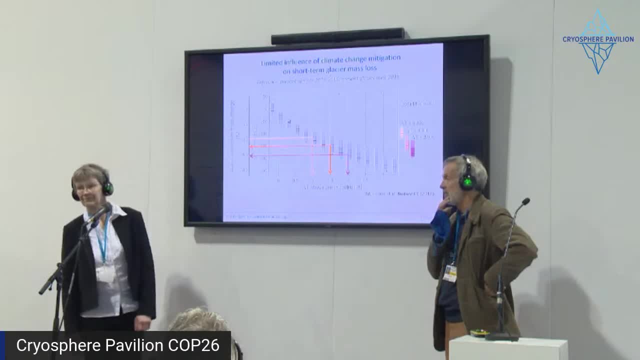 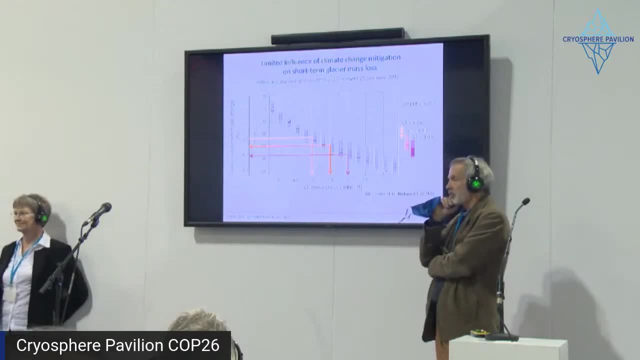 And maybe it's a very big impact which you can adapt and make the best out of it. Thank you very much for the presentation. I'm from Chile and I just want to second your view. I mean, a couple of years ago I did the Torre del Paine Trail. 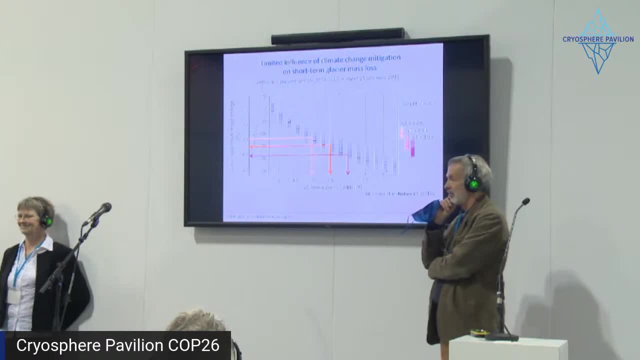 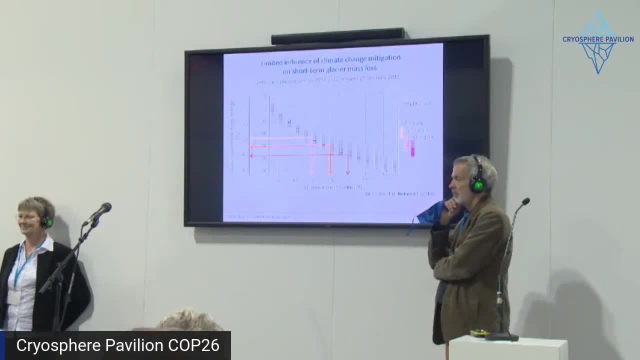 My question is: do you know whether the UN sister organization, the IPBES, is actually making the link between the losses in ice sheet in certain places, such as, for example, the south of Chile or elsewhere, the impact on biodiversity? 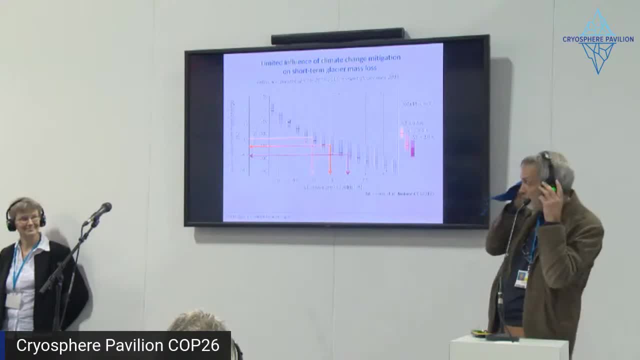 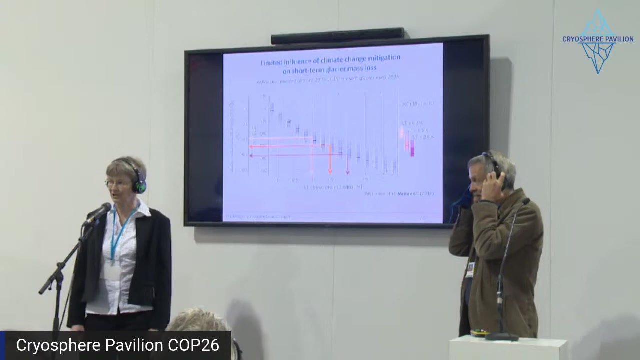 Thank you. I think Valérie would know the answer. So, Regine, do you know? Then go ahead. No, I don't know what is actually going on, but I have a hard time to imagine that this is not part of their assessments. 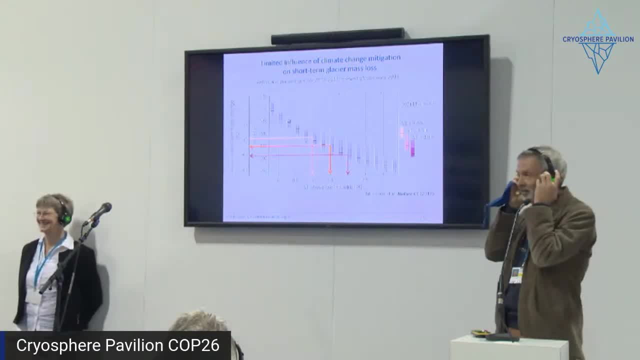 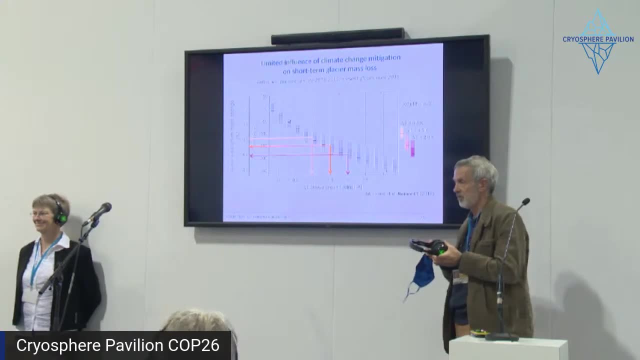 Valérie is nodding like this. so that is the answer, And I will say that one of the things we're often hearing- primarily, I would say, from the snow cover specialists- and we don't know what they're doing, and I don't have anyone like this. 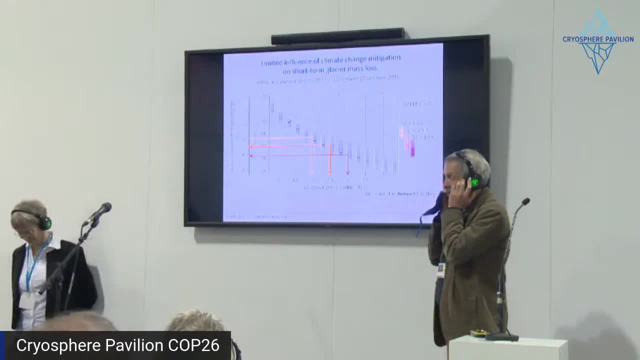 is that the changes at these high-altitude mountain ecosystems are great. The other issue that one deals with in high-mountain areas that people actually don't think about all that much, as well as polar regions once you get to a certain altitude- 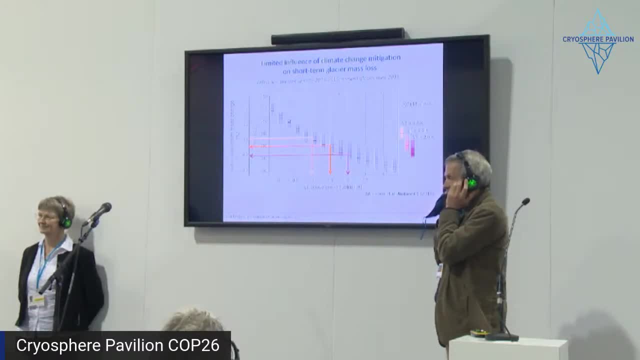 there's nowhere more where these species can retreat. They can't go any higher, And the same is of course true for the poles. So a lot of very unique species and ecosystems are at extreme risk because certain species only exist, say, in a certain mountain system. 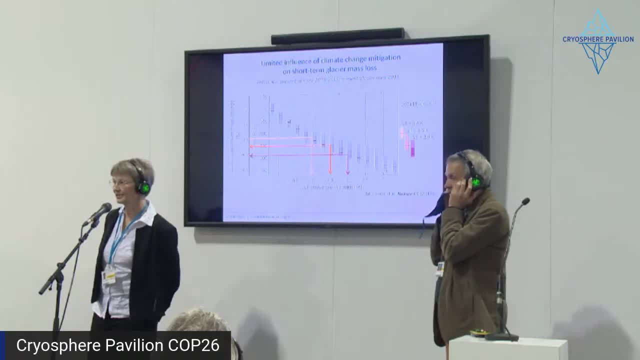 And so again, there's nowhere else for them to go. Just to add, there is actually a section in the SROC IPCC report on the changes in the cryosphere: the impact on ecosystems. It's a very short summary, but that gives you some idea. 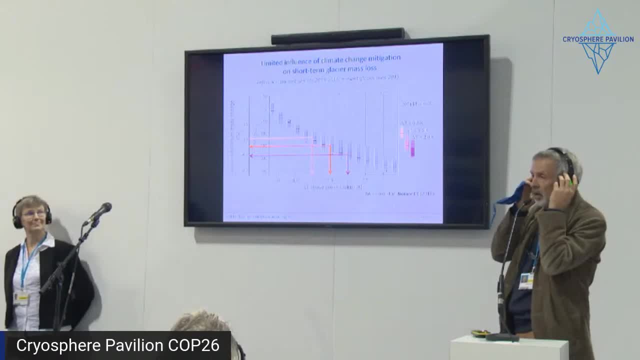 And there is some more information coming up in March where A cross-chapter paper on mountains is going to be issued within the Working Group 2 of the present assessment report. It's just in the very final review And by March, I think early March. 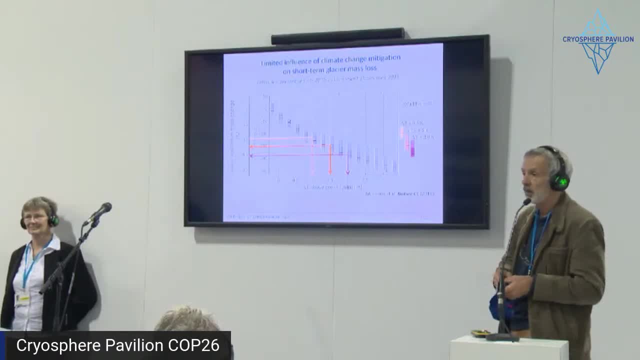 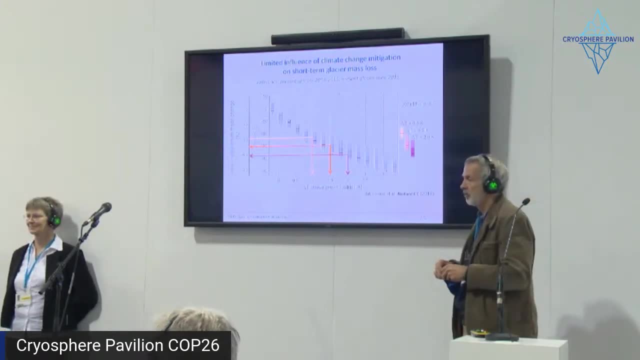 it will be negotiated with the Or approved by the governments and then it should come out. So I have a question. I have a question to both of you. Both of you work on glaciers. You've been in the field, You've worked with local communities. 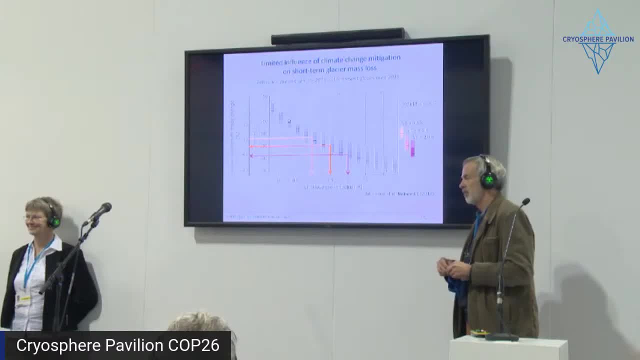 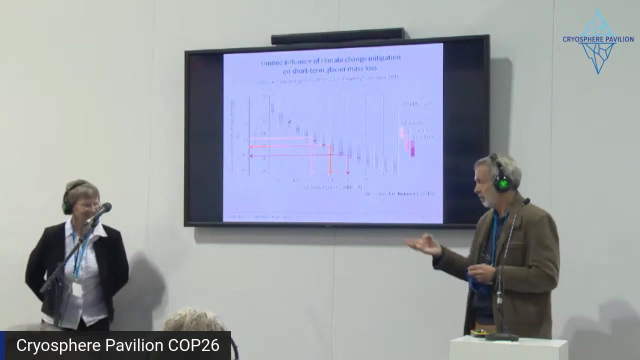 How do you engage with local communities to share the findings on future changes? What's your experience, What's your advice in engaging with local communities and sharing scientific knowledge with them? Well, I mean, an approach is to give public talks and engage with local communities. 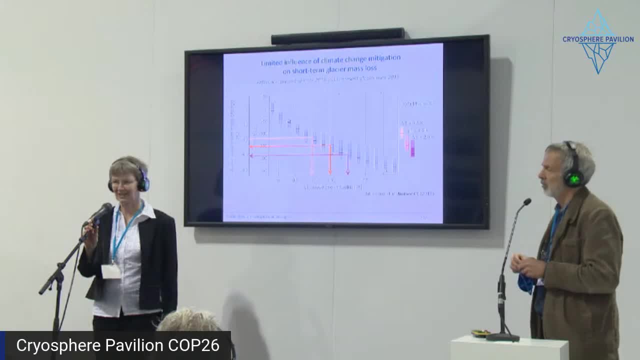 Also in schools. I have thought I've experienced that to be very rewarding and also efficient. I mean, even little kids at the age of seven can get very, very excited about these things and maybe then bring it home and discuss it at home. 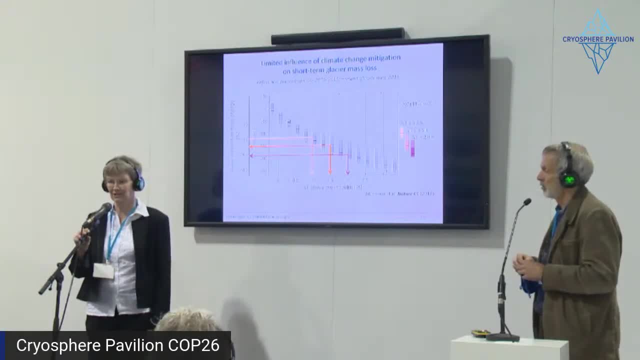 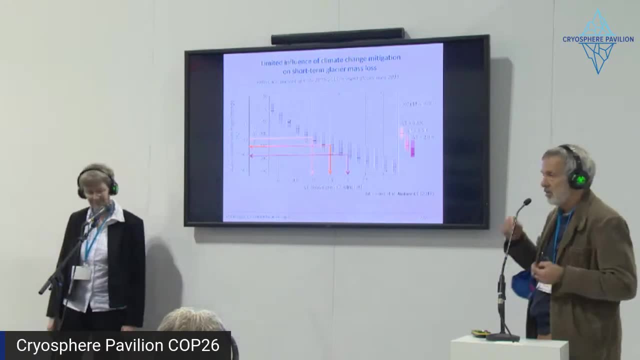 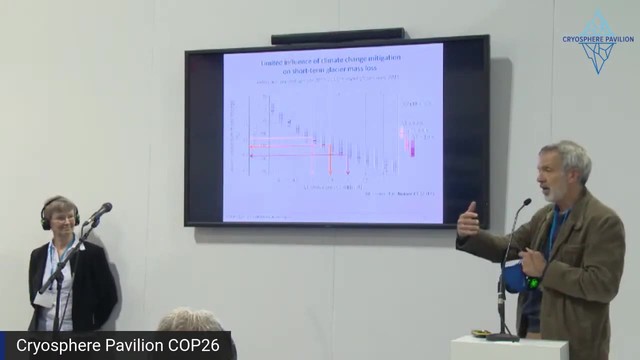 So there's certainly one approach to really engage with the communities and disseminate this knowledge or this interest or excitement. It is, in my experience, a bit difficult because there are always two parties. One is One, the active one, saying: 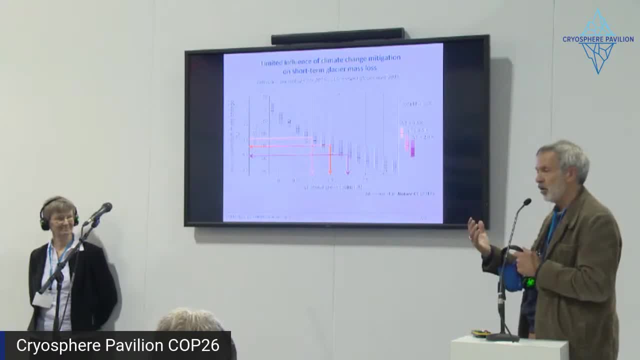 I know and I can tell you On the other side, if nobody wants to listen, then oh yeah, what can you do? And my experience is from the Peruvian Andes. mainly It is from East Africa, the Kilimanjaro region. 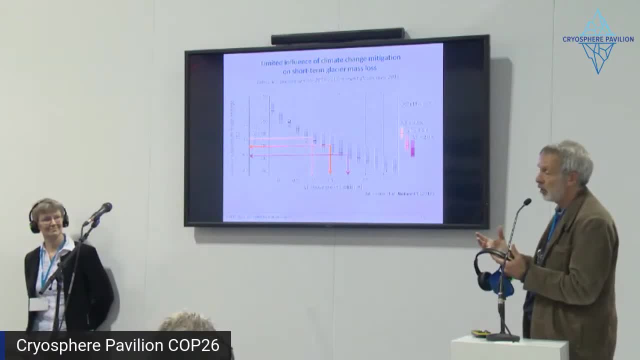 and the Mount Kenya region, Ruvenzore and the Austrian Alps. And it is totally, totally different because, again, in some regions, like for instance on Kilimanjaro, the people are much aware, because you can see these mountains from everywhere. 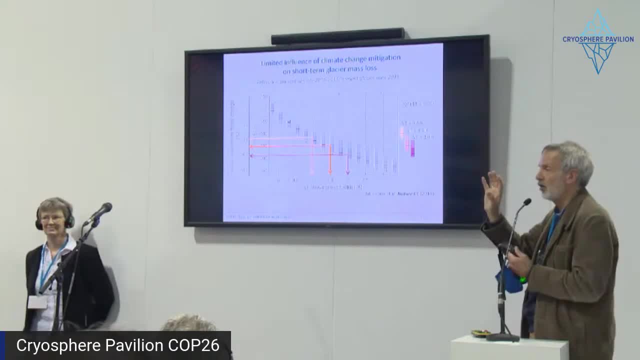 It's just one single mountain, like a kind of a model mountain, a Gaussian mountain, coming out from 1,000 meters, 1,500 meters, reaching up to 6,000.. Everyone sees this rim of ice and people are aware. 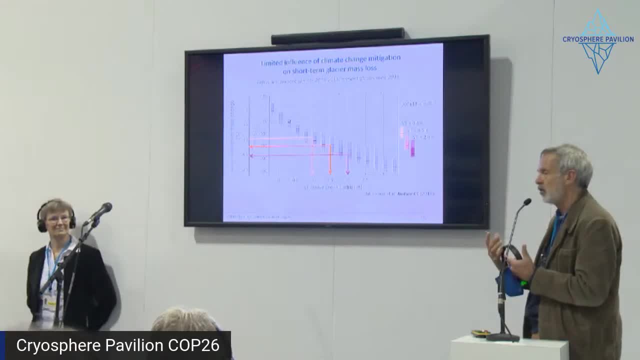 In some cases in Avron, they're aware that they are doing that, But now I don't want to talk about it just because I think it's important to talk about it. because I think it's important, because it's about lightness. 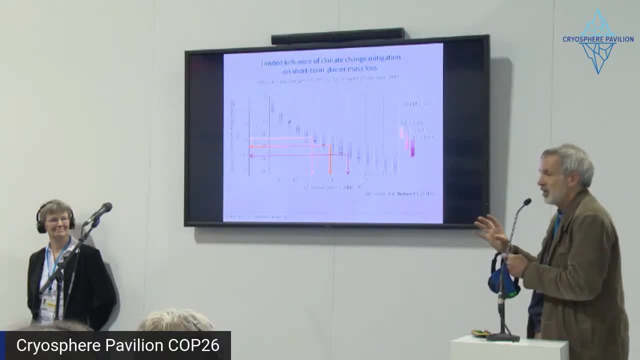 But in rare cases. if you're in the middle of a mountain and you're not aware that there's an ice, there's a lot of lightness. The first thing you want to do is to see the water. You have to try to get a better understanding. 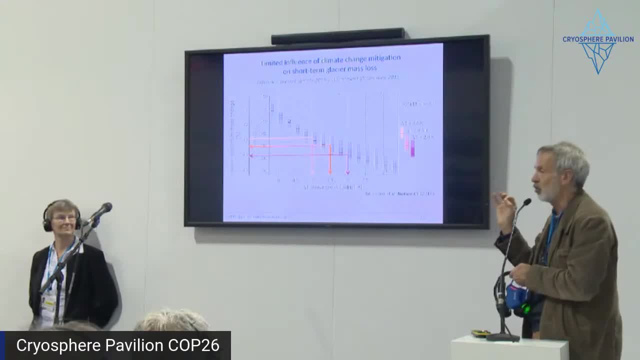 of how lightness is, And you can see the water going down from the mountains to the mountains, to the mountains, to the mountains, from the mountains to the mountains. I mean the water. so the rearmen to talk about in peru, it's again different. uh, you have always. it is a bit, i hope i, i am. 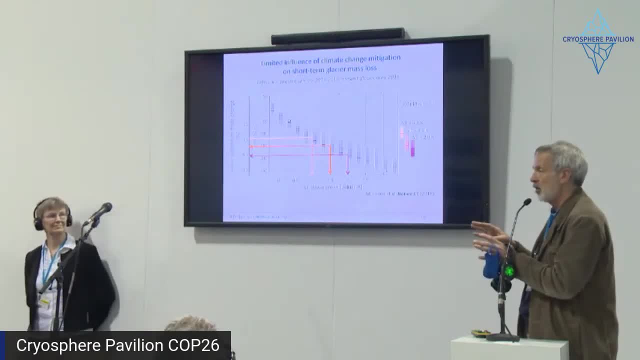 politically correct to say. in every discussion you enter with local communities, you always enter two tangential uh fields, very dangerous fields. one is uh the the coming from the first world or or the developed world, and uh the others being on on a developing site. and then there is an additional. 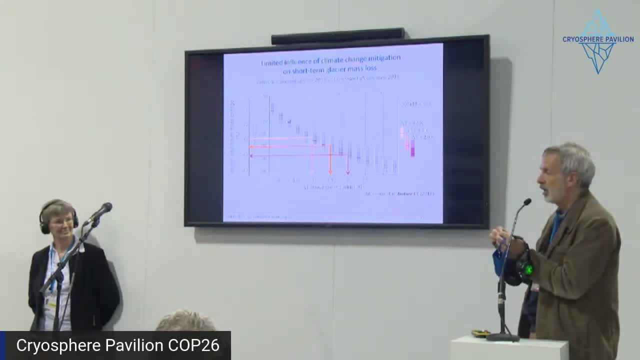 one which is even more explosive is the locals out in the mountain areas against the the government in lima, and they always try to to play out this, and so it is very difficult. as a glaciologist i have given talks to the ministers in lima, also to the local communities. 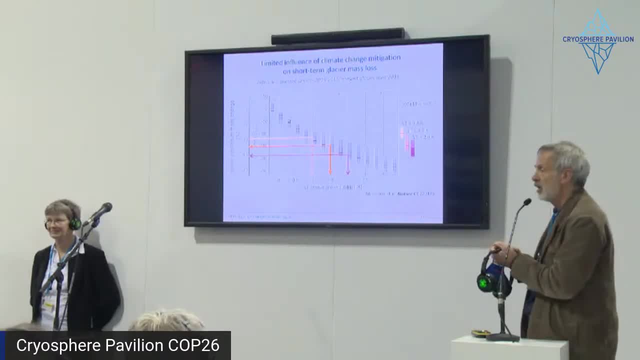 farmers, as we have seen with with heidi's uh figures, uh, that there is an experience where you have the same message, the same, the same issue and totally different uh, uh awareness, or even more than awareness. there is always kind of messages behind that: who, who is responsible, who is going to pay for it, uh. and there is, for instance, always if you go out. 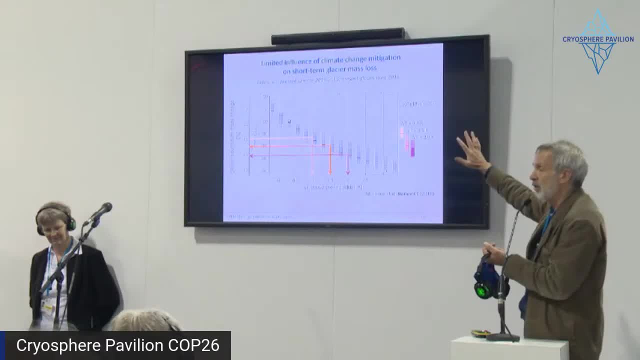 to the mountain regions, it's always the mining that's the reason for it. then you try to explain that it's part of it, but that's not all. there is also a global issue, and so on. then it's mixed up with contamination. we do a lot with school pupils. 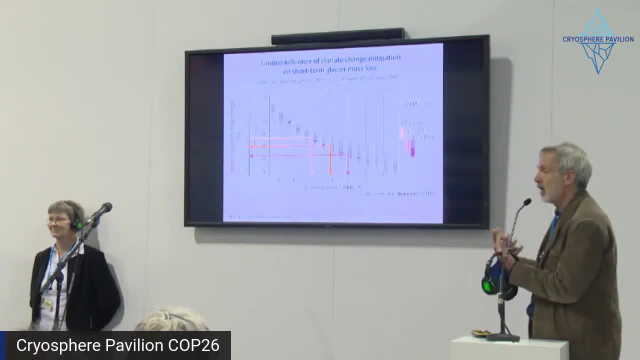 in in, whereas- or we did actually we even did studies with social scientists on the water availability and water uh demand on both sides turned out glaciers do not play a role in that catchment. we were studying but a tiny little rain which is not even measurable- less than one millimeter uh rain in an event has a special 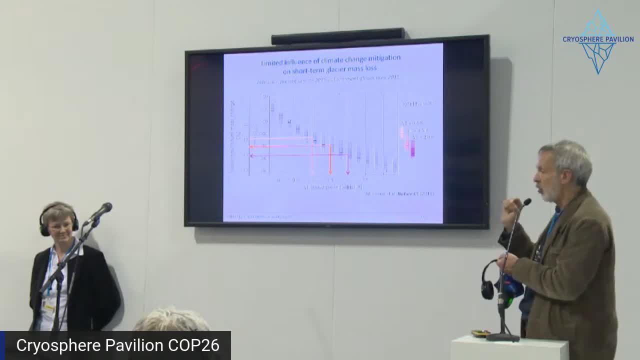 name, it's called the pusper rains and if this going it, this is going to miss or to fail, then the entire harvest period will be, or the entire agricultural period will disappear, or will will be lost, and it's just tiny little rains which we are not able, as natural scientists, to measure. 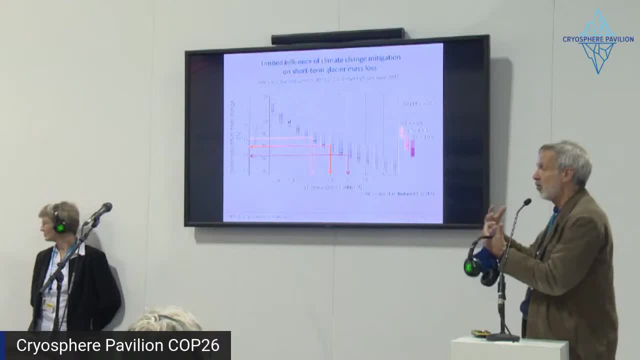 so that is things we find out by this communication. from both sides in the alps there is totally different. the glaciers, key resource, ask: how how many years can i preserve the glacier? what can i do to preserve the glacier? i always say: don't preserve the glacier, precise. preserve your little ice patch where you have. 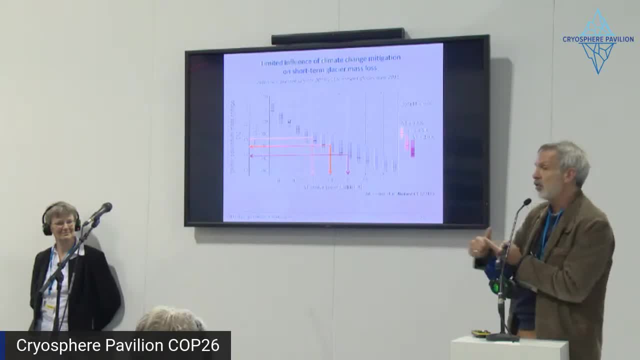 first, never temperatures above zero degree, which is easy then to to make technical snow on it. to put technical snow on it and it's smooth compared to this rough terrain underneath. but on a long term, calculate, do every calculation. do not lose money in preserving glaciers. use money or save the money to do then the ski resource. 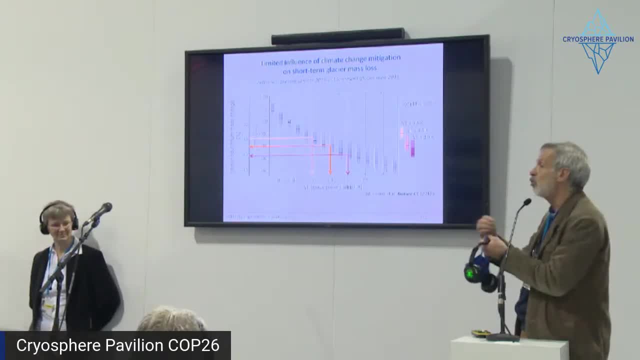 up afterward when the glacier is gone, or do, or do not make wrong infrastructures which then 10 years later you have to build up a ladder to reach the ski lift because the glacier goes down. just build this key lift where it is also going to work in 20 years and 30 years when. 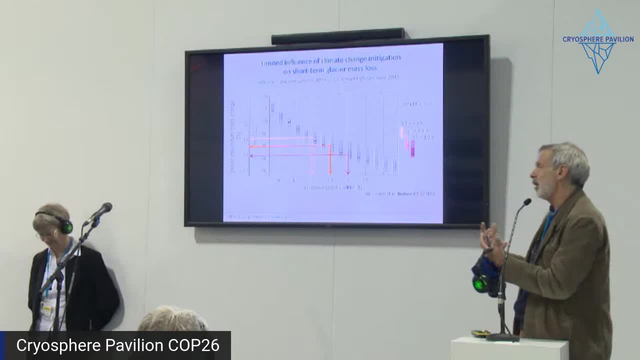 the glacier is gone, so it's a very important thing. it's very different approaches, but uh, yes, valerie, we are very, very, uh much behind that, and we, since i'm retired, i can even speak more openly to the people, not only as a scientist. it's a good. 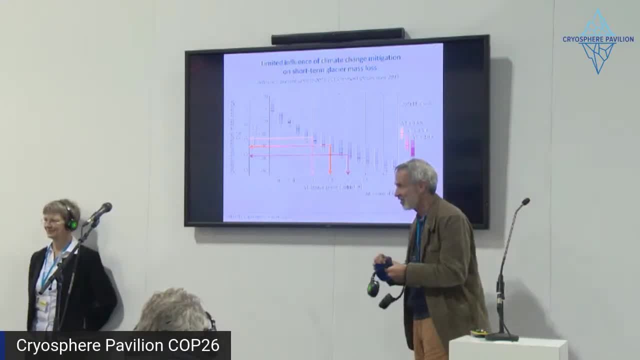 it's good state of. i'll say also, you know all of the the uh events and presentations here are um recorded in catch so you can find them on the web page. and uh heidi, indeed, sitting in the back there, gave an excellent presentation of one you know local connection. 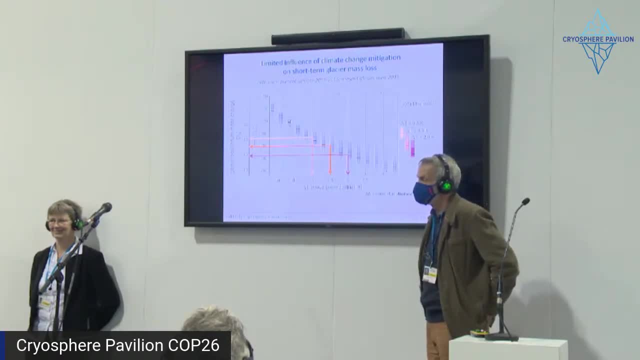 of scientists with local peoples. that was very helpful. um so, thank you for that. other questions, and i'll say, in our next presentation we also should have a representative from the protect our winters campaign, that is, you know, sports people who are interested in, uh, working in the snow, obviously, and that that actually is their. their message is, uh, i would say,